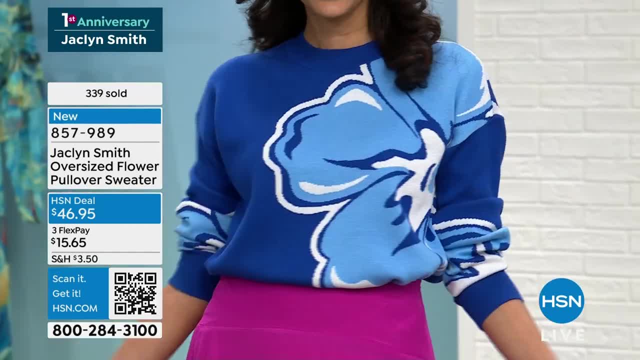 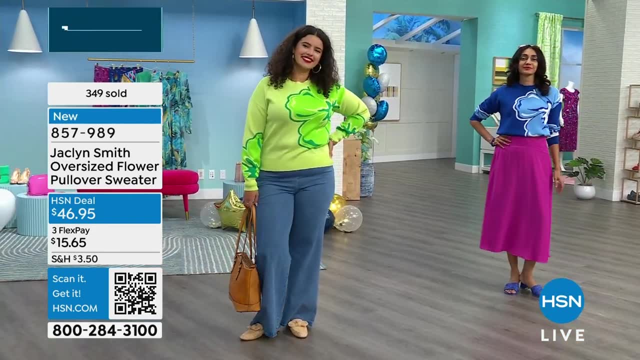 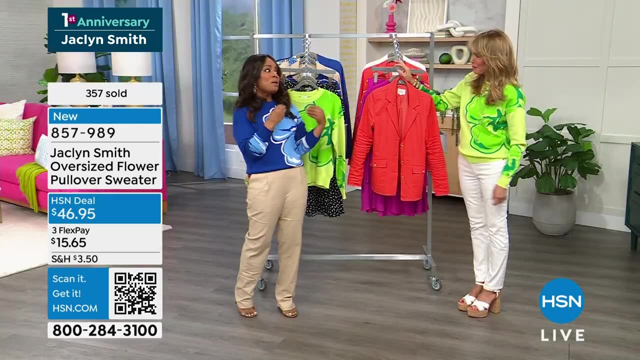 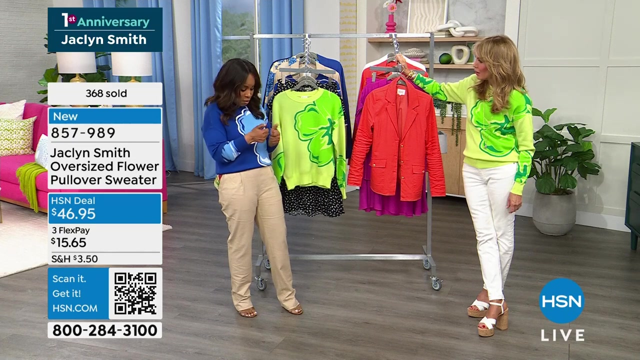 So as hosts when we come in. actually I started early. My producer today is the famous Rocky. Many of you at home know Rocky. Rocky has been here at HSN for many, many years, for over two decades- So he's a very famous and popular producer. So a lot of our customers know Rocky by name. They may not know him by face, but they know his name for sure. So Rocky is a producer of the show. He called me earlier at home And so I was looking at the pieces at home before I even arrived to work And I said: Rocky, this is, I love you. 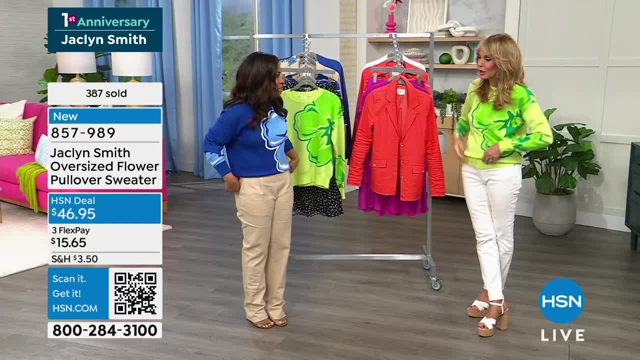 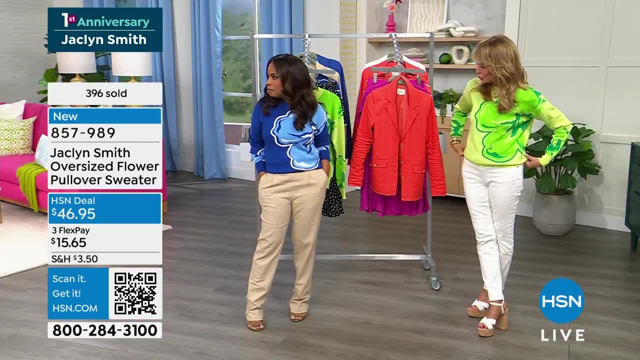 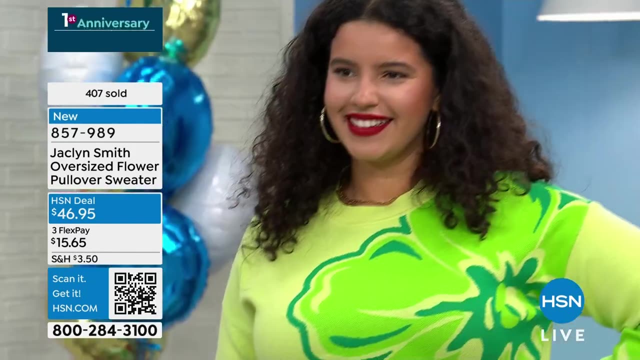 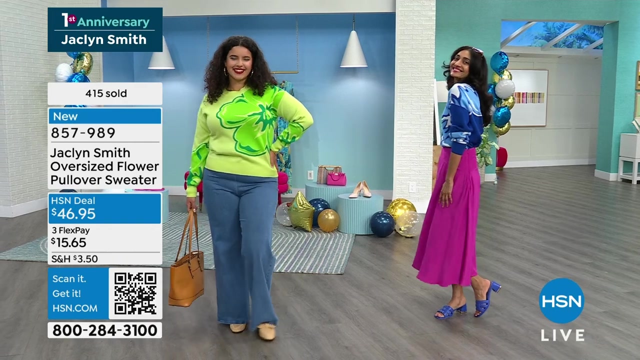 You want that. I said I love this sweater. You know it looks perfect. I like the way you ruched it up. Yes, I just kind of turned it up. You turned in that and that's she's tucked it in. You've made it a little shorter and made it crop, And that's the great thing, And it's so. it's an easy piece. I slipped it right over my head. I still have the same blouse on from earlier. You can tie it around your neck. You can even wear a shirt under it if you want. Yeah, you know it's nice to have it on hand And you know we talked about it. You know you were saying how the nights in California are cold. And then this time of year, 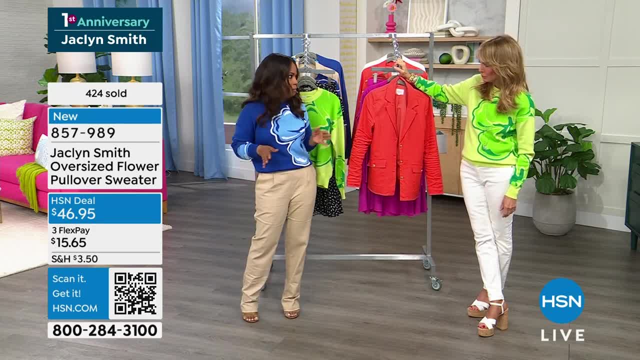 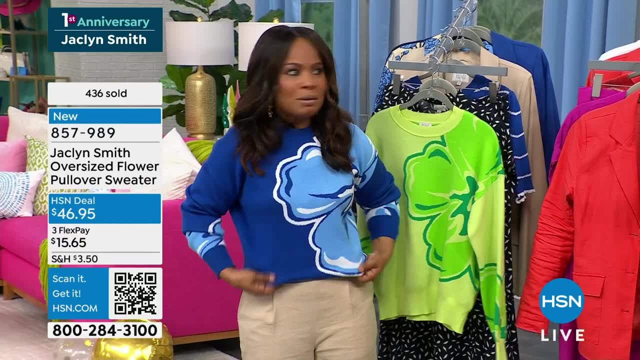 you know it's interesting, The weather. I sometimes say the weather is- has a little bit of menopause- right, It's warm one day, Right, And then the next day it's raining, It's raining cold. Yeah, So it started out that way today. Yeah, exactly, I thought we were having a hurricane. 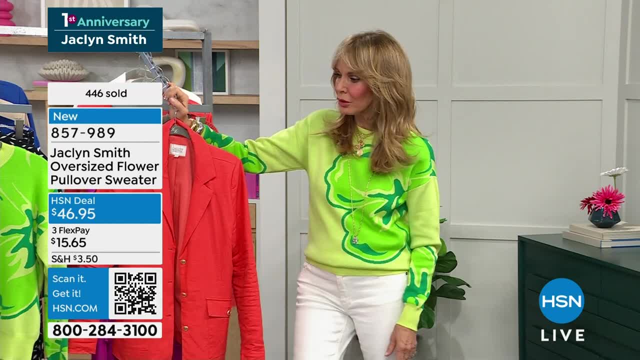 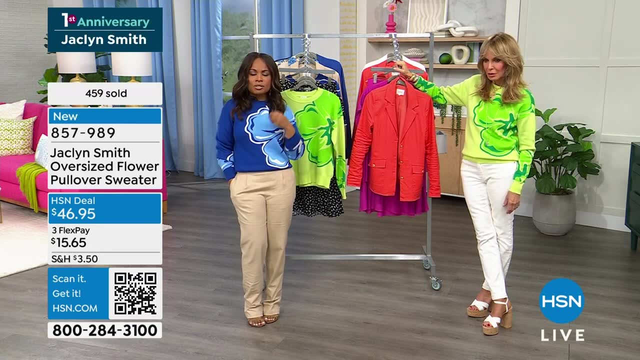 Yeah, today for sure, Right, And now it's sunny, So you have to be prepared. You have kind of four seasons and any type of weather, and even one day You're right And something like this is very striking. Like it just has, It really looks great. Yeah, I like the way. Okay, Extra small is sold. 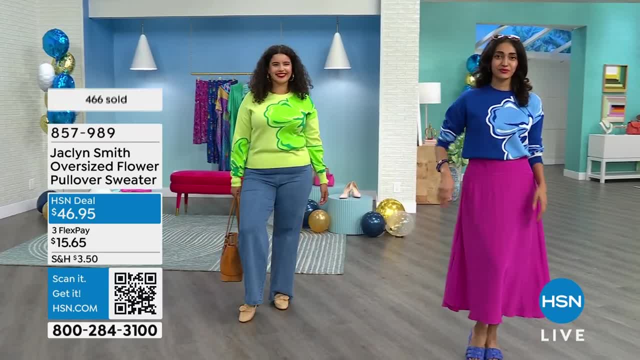 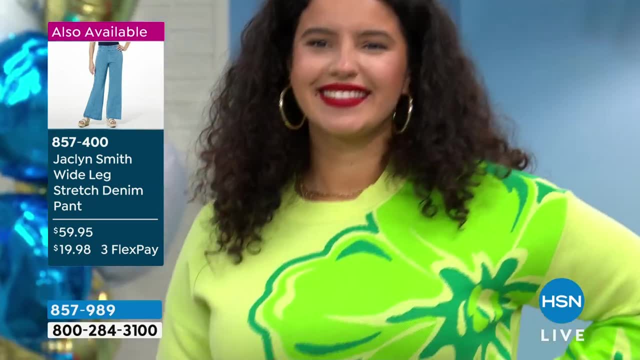 out. in both choices, Your extra smalls go. Wow, So the extra smalls sold in that blazer. by the way, if you love those, those, those denim stretch pants- I've been eyeing those. Well they're. 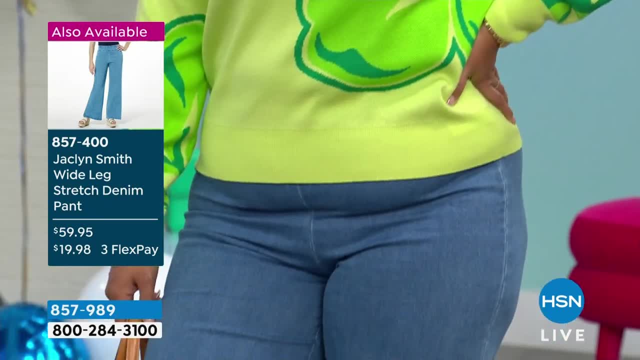 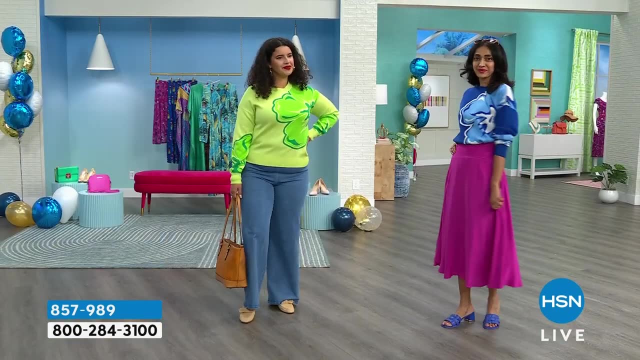 very comfortable, but they have a great fit. They're very flattering. Again, the flat contour front, the flared leg- Those look great on. It takes me back to the seventies. Yeah Right, You inspired the girls earlier, Yeah Right, But look at how great they fit. 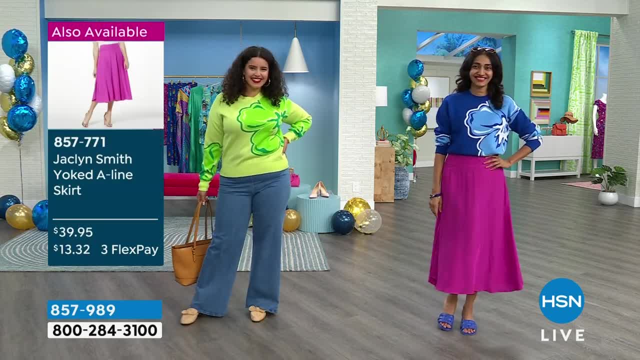 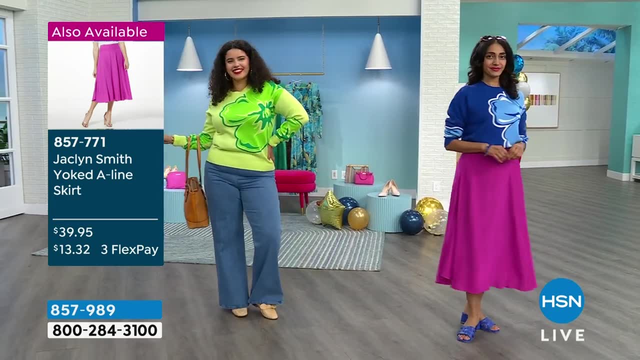 They look great, Yeah, Really. on all sizes and shape. They're very flattering, All right, If you'd love to have this sweater, by the way. by the way, we're providing you also with the item number for the skirt. So if you want to recreate Simi's look, there is the item number to the left-hand side. 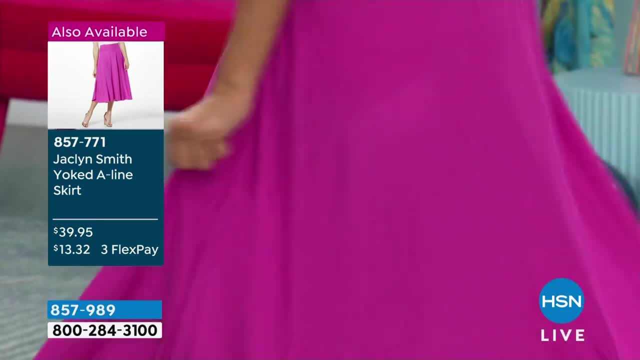 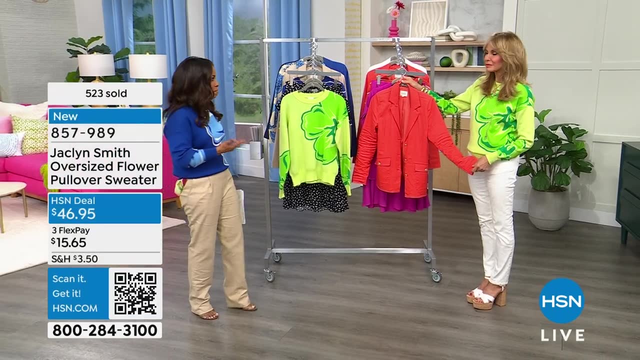 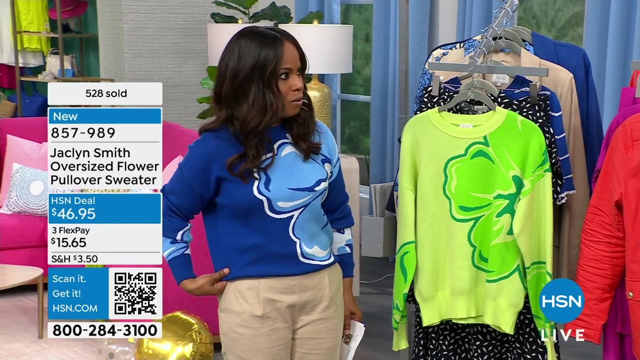 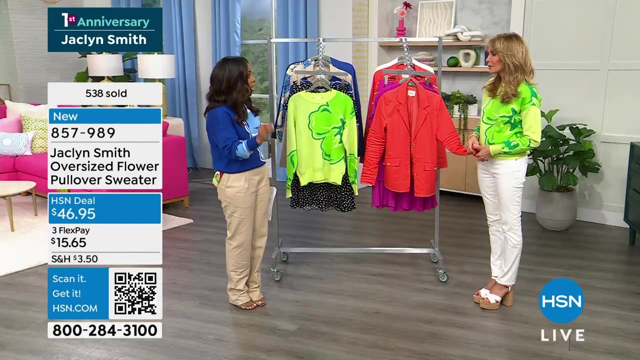 for the A-line skirt. I should also let you know that, as you're shopping with us, we make it easy for you with what we call our flex pay, And that simply means, Jacqueline, that you can actually pay $15.95 plus the tax, And we actually ship it to you right away. And then, if 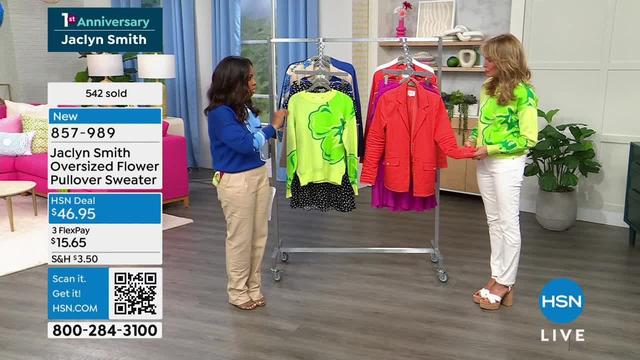 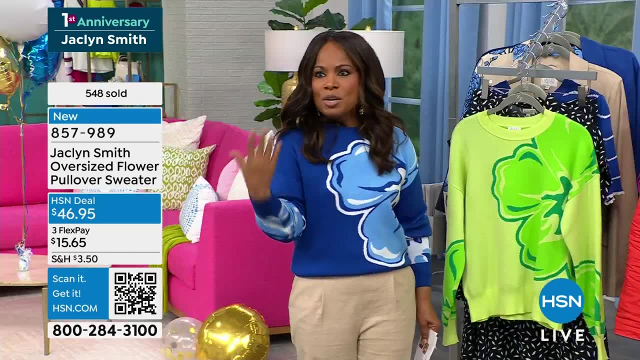 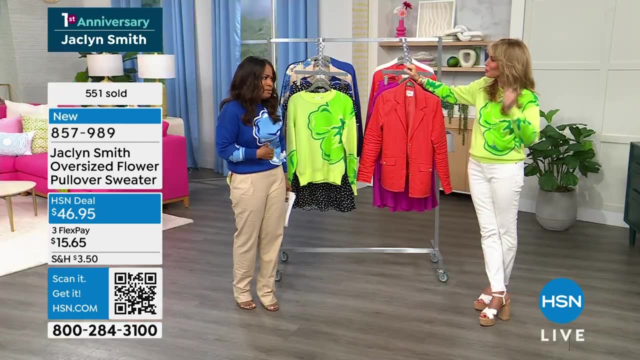 you're using a major credit card. we have three interest-free installments every 30 days of the $15.95.. So we do that for you because we know that. look, sometimes you just need a little shopping therapy. You do It just sort of lifts the spirits, It does Something new to put on. 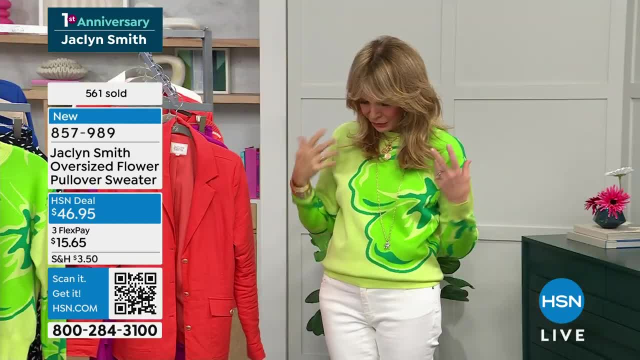 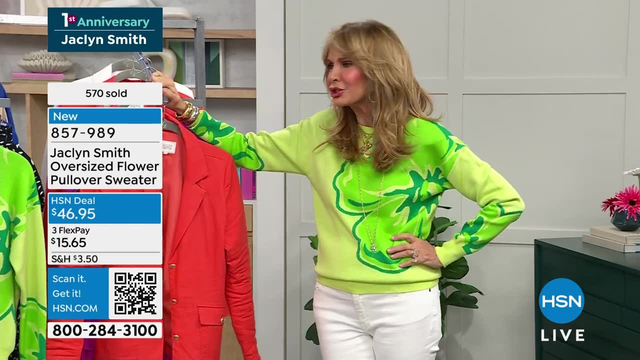 You know, I had a little jet lag from coming from. I put this bright color on and it just was like sunshine. It was like vitamin, pure vitamin D. That color is phenomenal. So colors and shapes, they can sort of lift your day. It's nice to feel pretty. I mean, the A-line skirt is 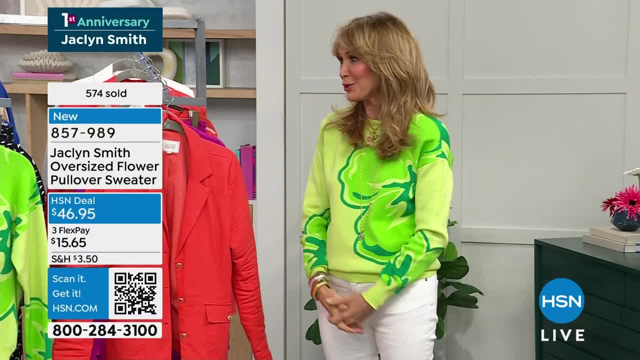 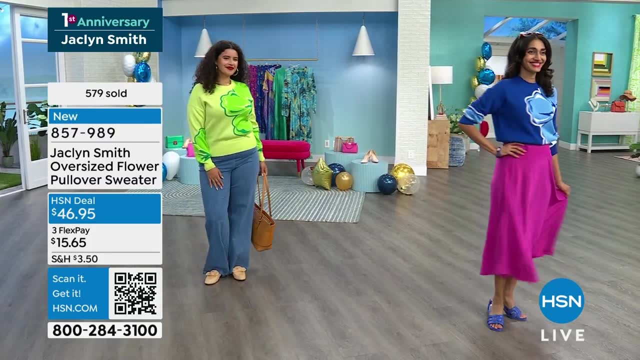 instant femininity. My husband always wants me to wear skirts and it looks so feminine. That's all right, It just moves, It has choreography. I want to give you an update and I apologize, In this sweater that you're seeing. 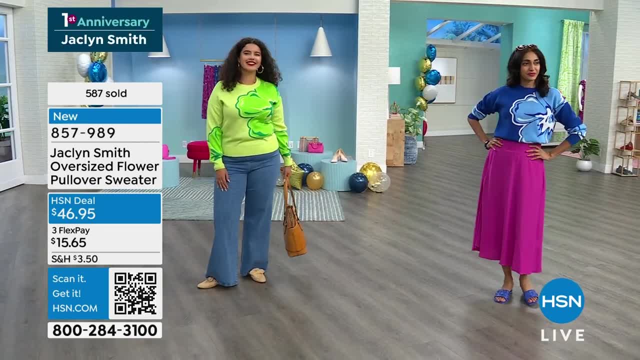 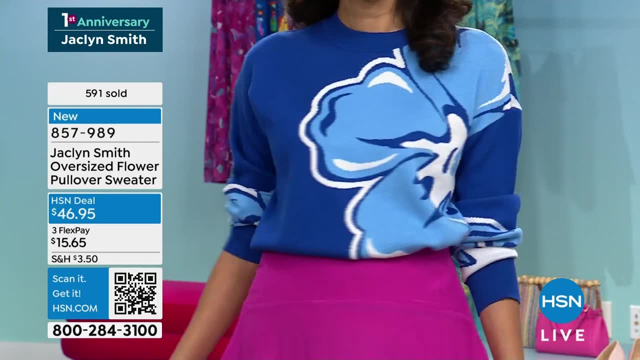 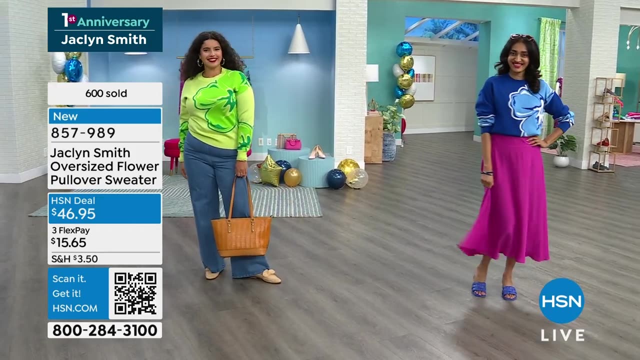 we've sold almost 600.. This is remember. I said earlier that I've had the great pleasure of working with Jacqueline before, And there are occasions where we'll launch a new garment and that garment will only be seen in one show and one airing. That's going to be tonight And it's 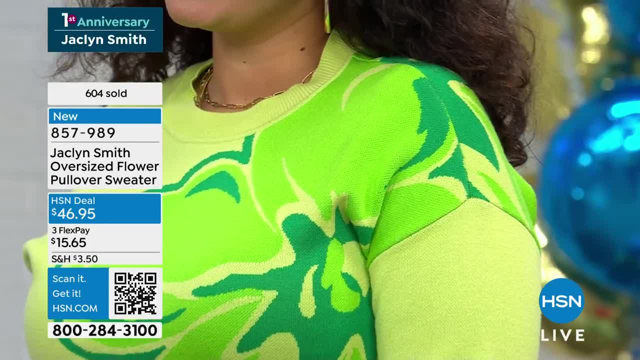 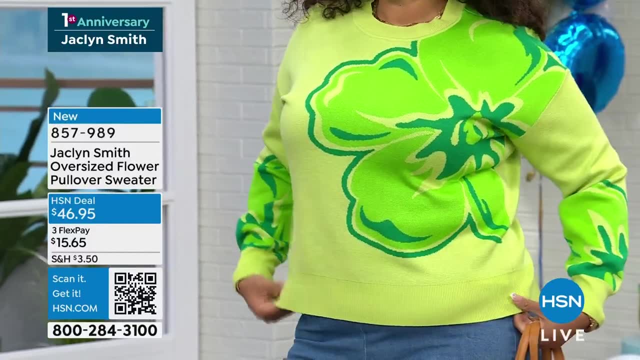 going to be with this sweater. This sweater is on its way to a full and complete sellout. You're the first and only audience that will ever get a chance to buy it. It's new tonight And here's what's. here's what's remaining. We're actually going to count it down. 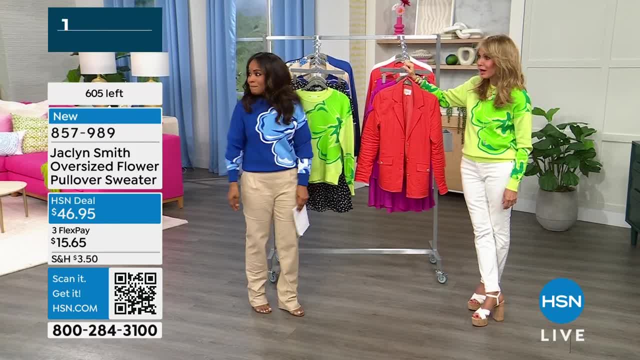 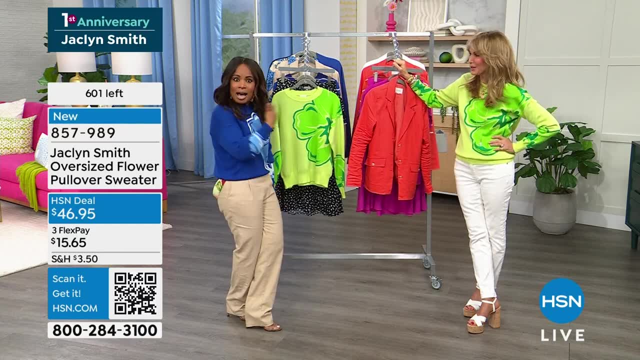 Wow, I know Wonderful. Well, I, I, I, love, I know how to pick them. You girls, you did great. I think we're all on the same vibration tonight. Yes, Because I loved it too. Right, We all love it. I think we all love this. 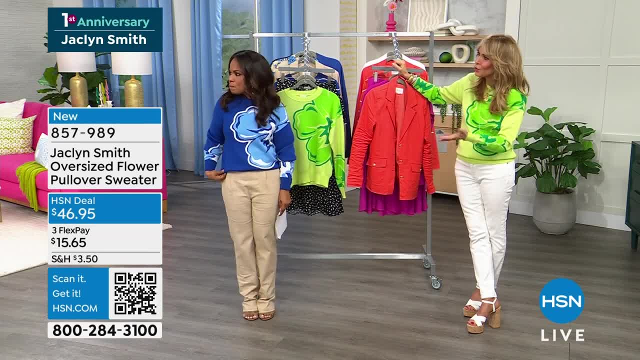 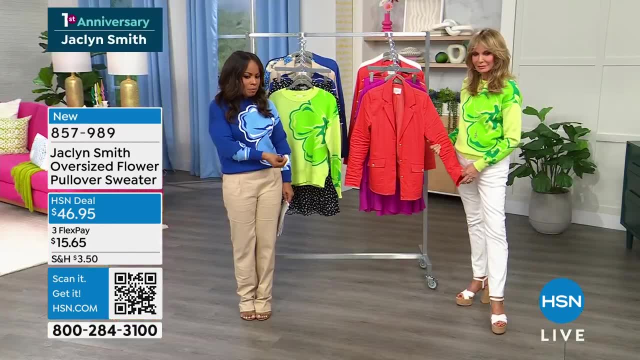 one, Yeah, And my floral offering seemed to do well there, there, you know, a season ago. Yes, It's just. you know, I think, when we're looking at this, when you look at the price, right, there's, there's, so The price point is amazing. But also, 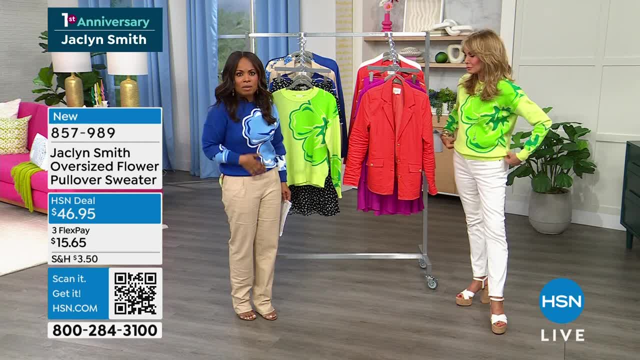 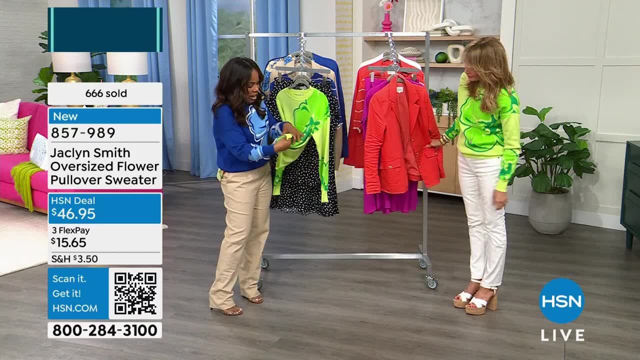 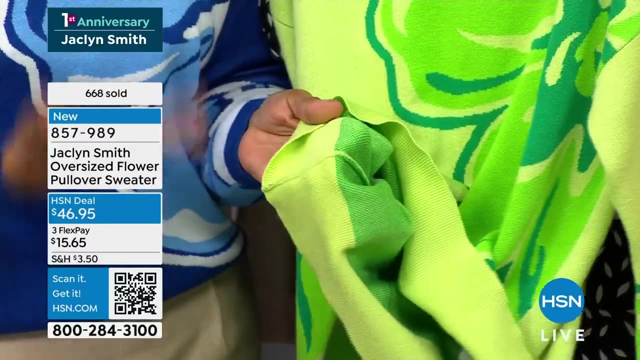 your quality. That's one of the things that, if you're new, I cannot wait for you to touch it and feel it. It feels good on, And when you turn even the garments in, they're just made so beautifully all the way. Oh my gosh, Like Jacqueline knows, I'm such a big fan Like 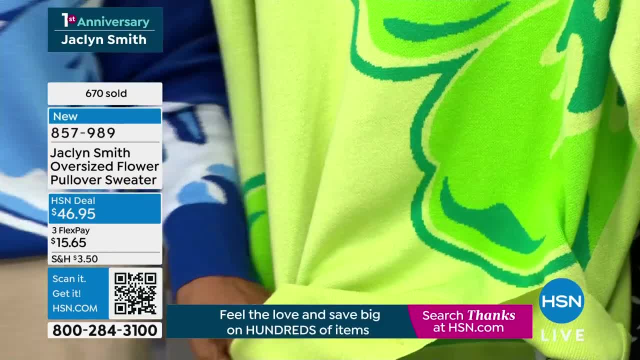 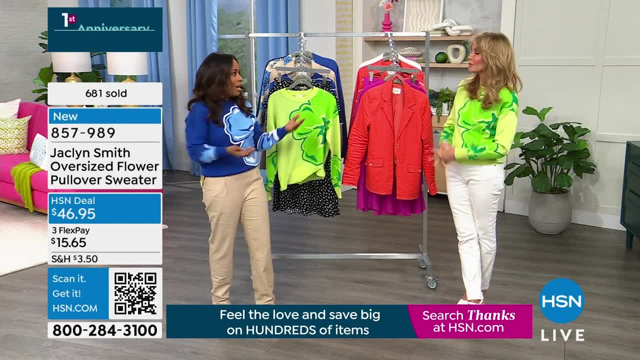 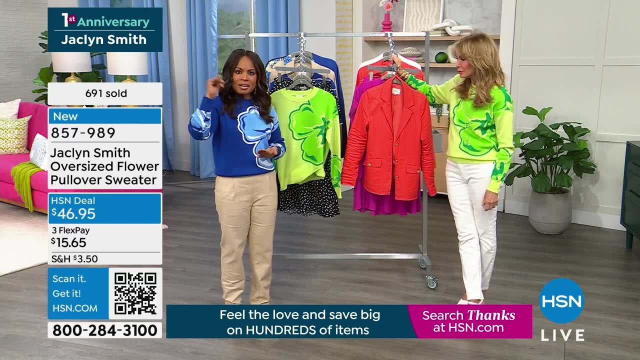 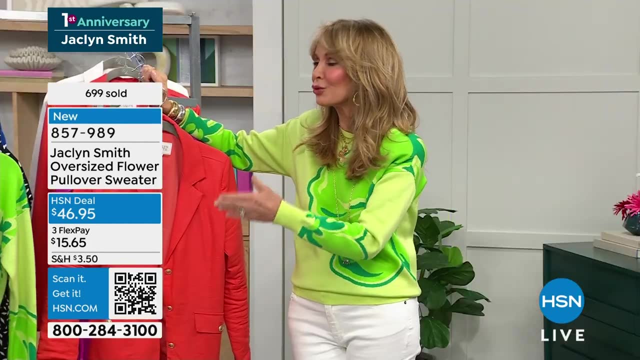 and these are pieces that you love. that obviously looks stunning on you, but It looks stunning on everybody. You, you give us this, this really elevated look, But at an affordable price. At an affordable price, And that is the DNA and my brand identity: being able to dress beautifully and not 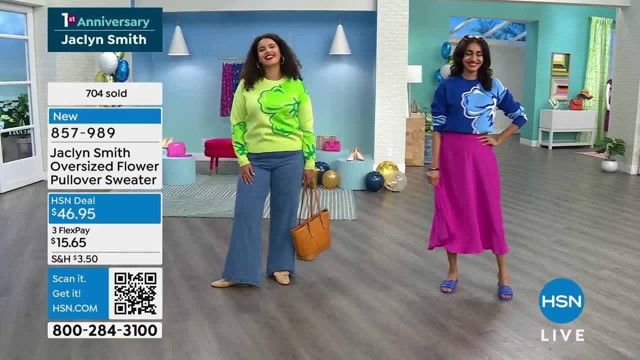 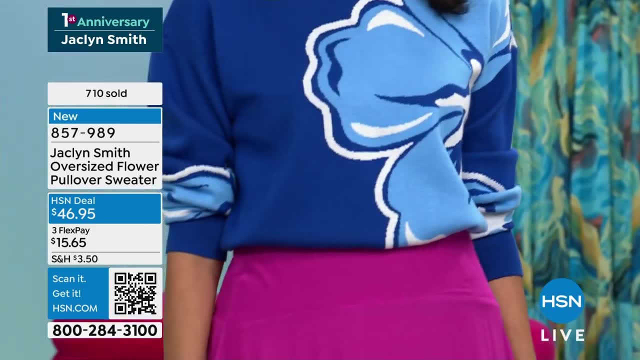 spend a fortune. Yes, Not spend a fortune. Everybody should be able to do that, And if you're a smart shopper, you can. Okay, Let's talk about the lettuce green And the lettuce green green choice. we only have large through 3X, So if you need the large through 3X, you'll need to. 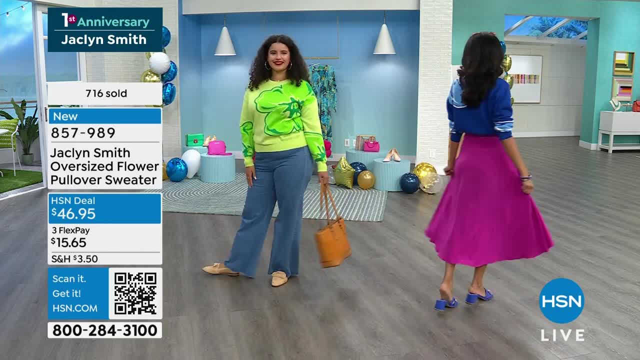 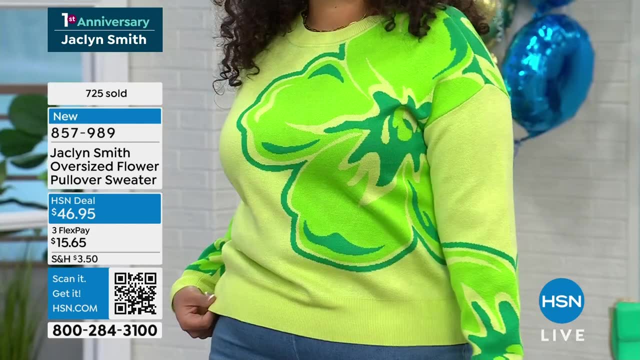 hurry. in the lettuce green, Our beautiful Natalie is wearing the large in the lettuce green And if you're large like Natalie, you can still get that through the 3X because we still have it available for you. Natalie is wearing it with that denim, jean, And we all, most of us, all, most of us have. 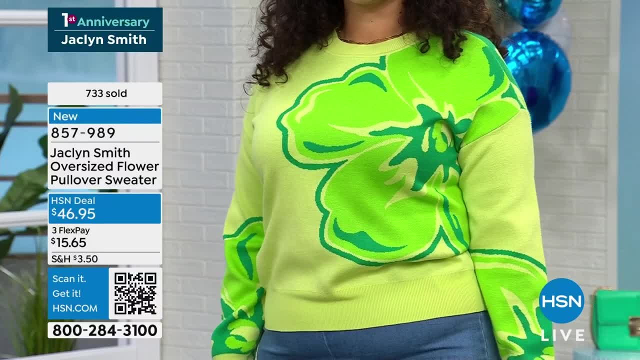 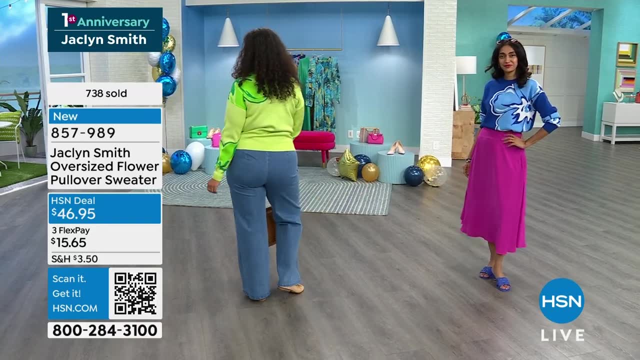 a pair of denim jeans. Look at how great she looks with her denim jeans. It looks great with dark jeans, faded jeans, medium wash jeans. It really yeah, And I should mention also on this one, we are simply talking machine wash dry flat, like you would with all of your sweaters. 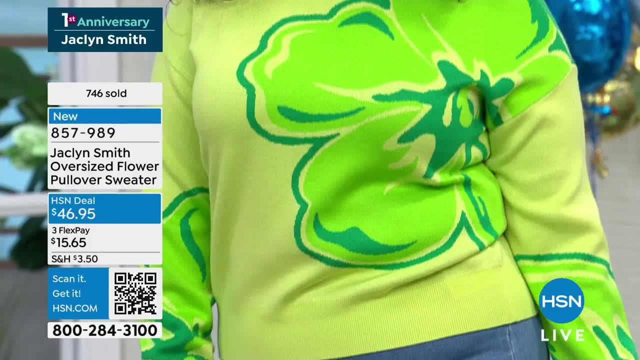 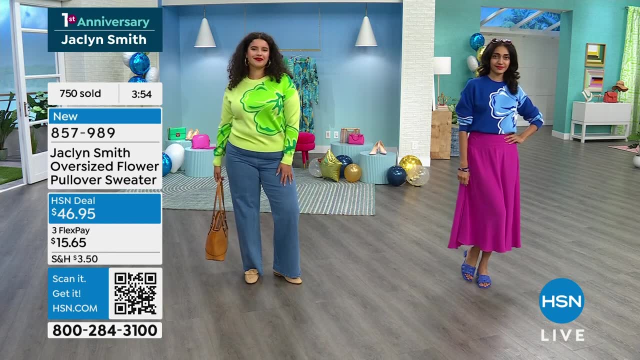 The length is 23 and a half inches in the length, Natalie. by the way, her numeric size is 16.. Just to give you reference, she's also 5'9" Also, so that you'll have all of the information to make. 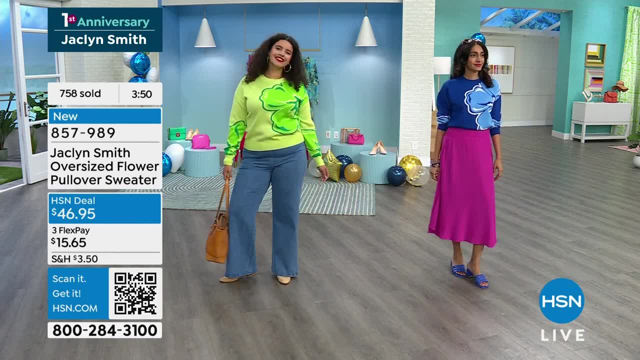 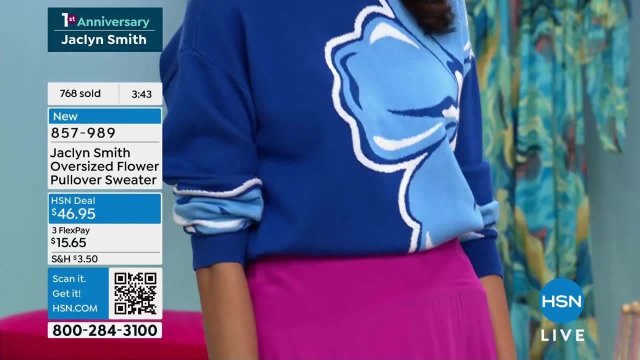 a decision, So she is wearing the large. By the way, 758 of these are available And we're going to be talking about all of these in a little bit, So if you're large, you can. we have to also talk about my beautiful Simi. She's 5'7". She's wearing the color that I'm. 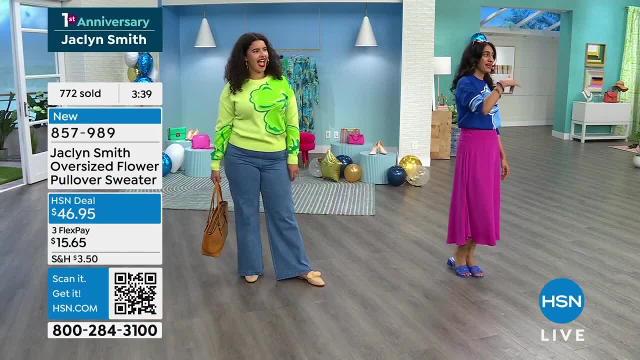 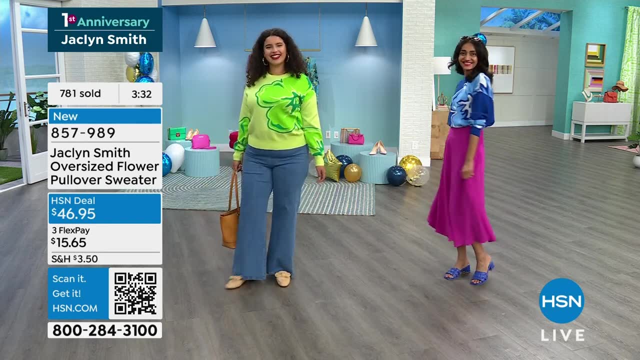 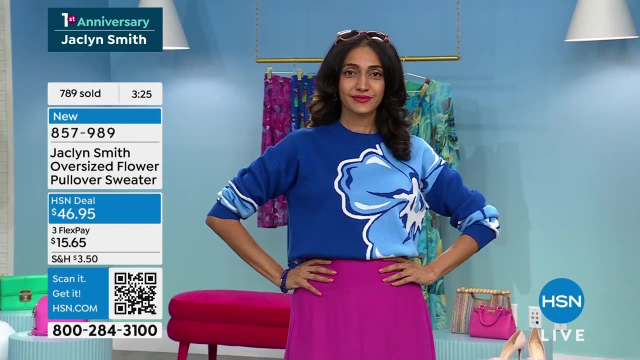 wearing, which is called Surf the Web. That's such a fun name, But that blue is phenomenal And I love that. you have that deeper kind of cobalt blue, but then you also have the light blue and then the optic white that's woven throughout it. for me is everything, because that white jean 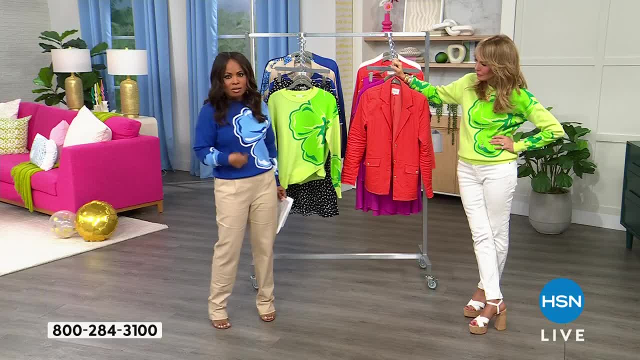 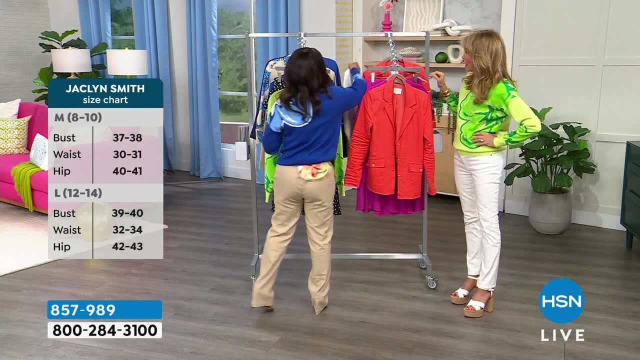 that white trouser that you're going to wear is going to look phenomenal, But it even looks great with what you have on. Yes, Even if you imagine, if I had, imagine if I had on like even a pair of denim jeans- Right, If I had a pair of? 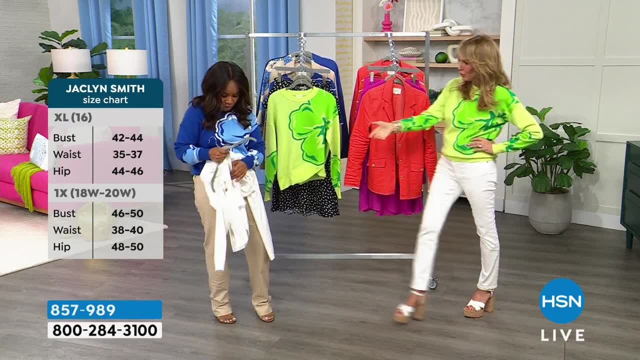 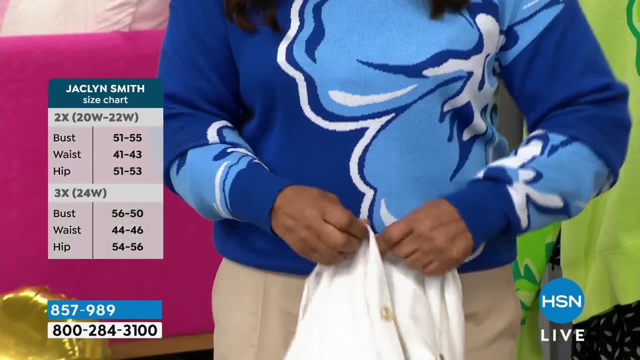 denim jeans and even if I had this white blazer over it, Let me hold the hanger for you. Thank you, Because it has- I don't know if you can see it has- like optic white Right. So any other white. 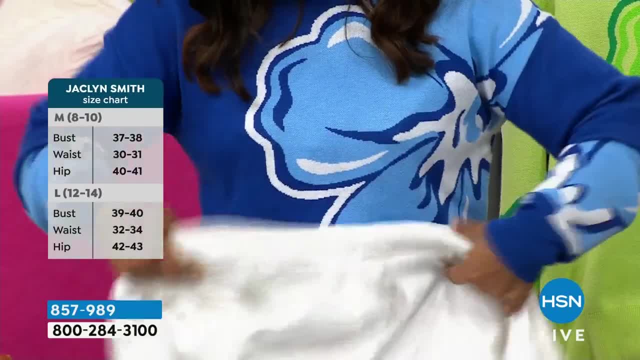 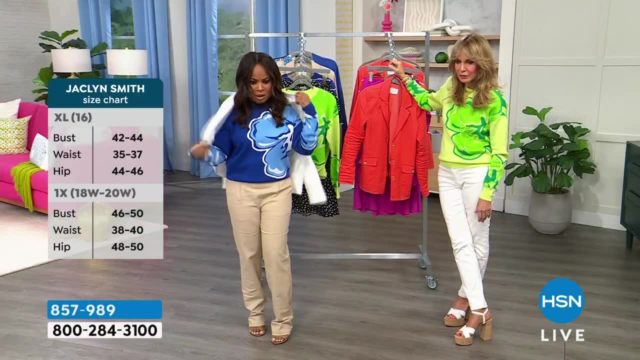 that you pair with this. oh my gosh, it is going to look like beautiful, Like a million dollars. It looks great, Right? I know I've got a lot going on here. Yeah, Yeah, No, it looks great, I don't. 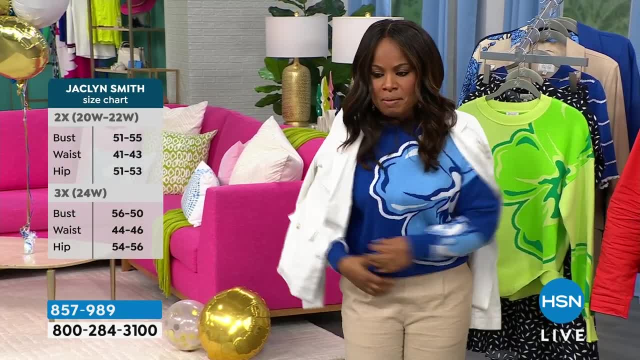 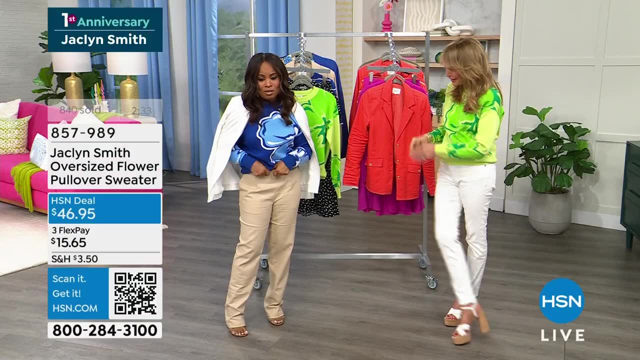 have a mirror And you can. But you can imagine just kind of pairing it together, Right, You know I have quite a number of clothes right now, but you can imagine You have three layers. I do, I have one, something else from earlier, but Right, And it's working. Yeah, It's working So, but just 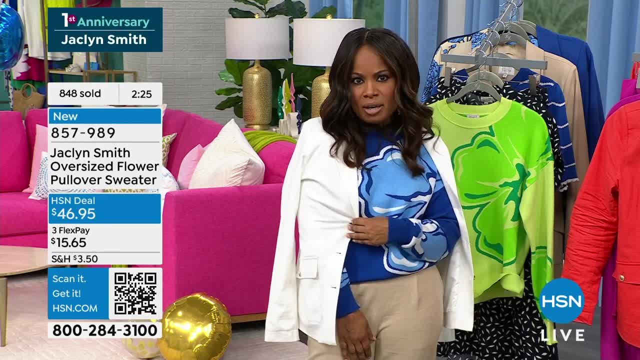 it would just be beautiful with any type of white. I love the blue with the white, Me too, Me too. And it works with this too, Because it has the white in it. But it really looks good with the blue. Yes, 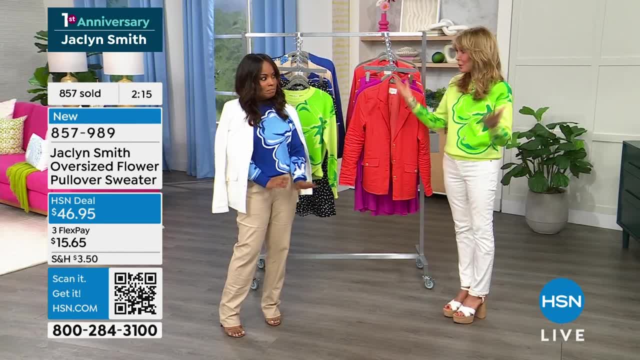 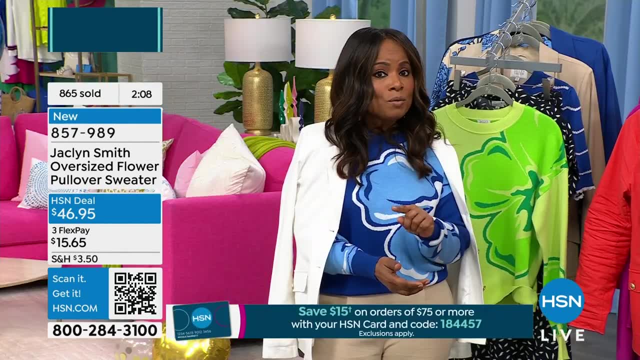 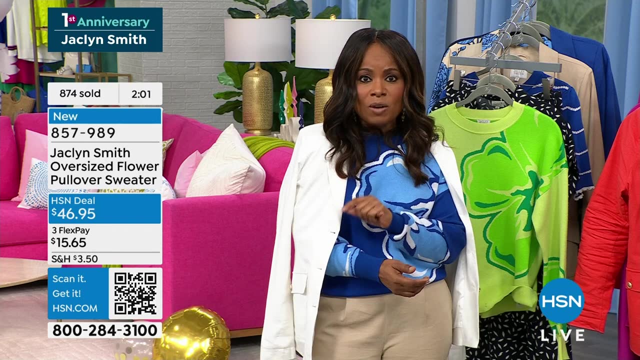 So you might decide you know Both colors, You might. We have the Flexway. We're approaching almost 900 that have been ordered, And remember that when you're shopping using an HSN card, you'll receive $15 off of every purchase of $75 or more. Now remember once you get to $75,. 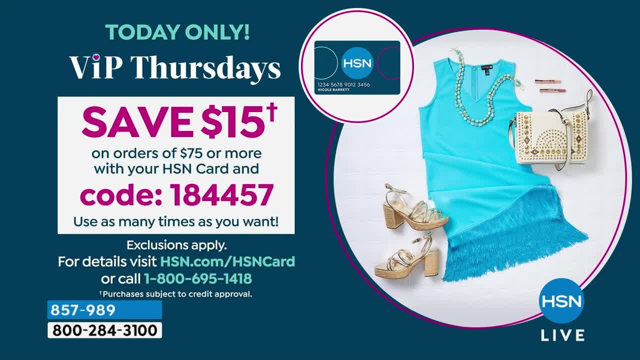 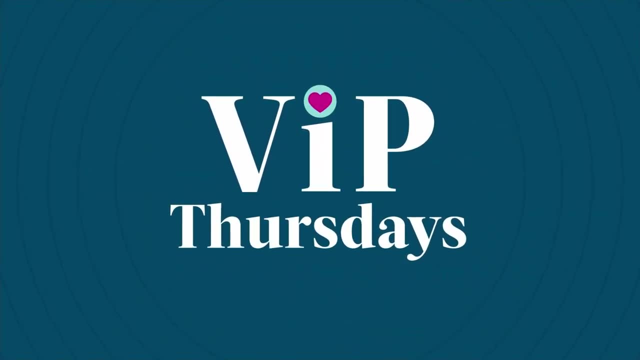 check out, Because that way, because you can use that several times, Right, You can use it repeatedly. Okay, Here's an update. It doesn't matter the color that you're choosing. There are a little over 120 remaining in either color. Ooh, It's, you've got to react. Yeah, I know It's. 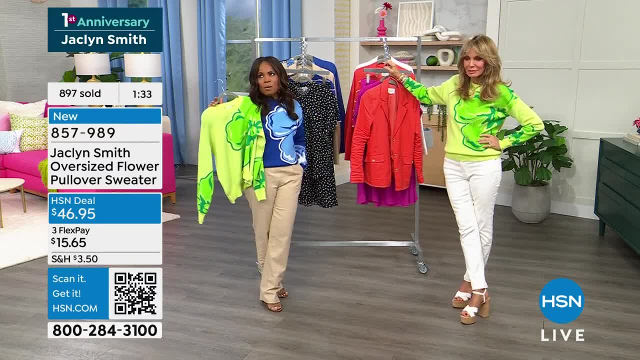 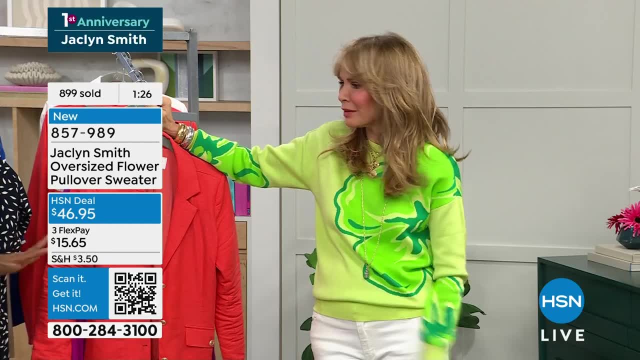 hard, But I will tell you. what is it that you know? are there class reunions that you're going to be going to. This would be so beautiful. Well, it's just great all summer, for you know, Because there are a lot of class reunions and family reunions, Absolutely, And 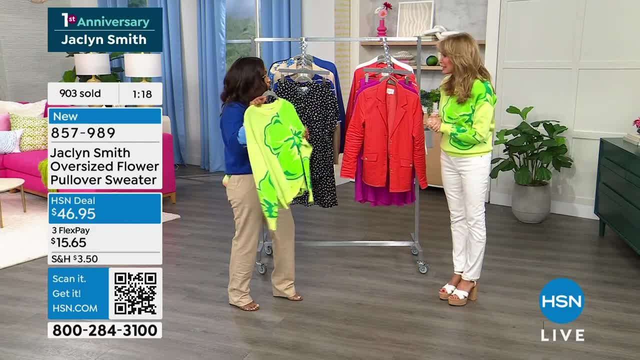 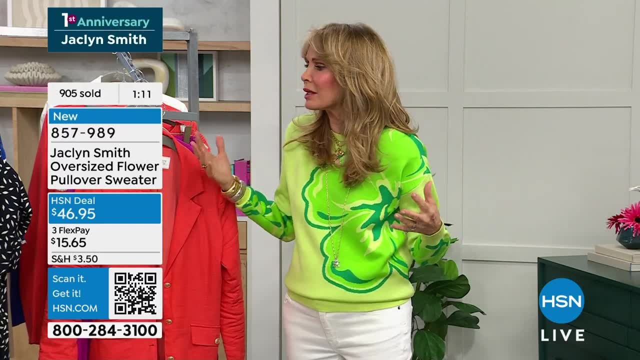 This would be beautiful to wear to church. I have church Mother's Day. That would be stunning. Tees, Tees, Birthday parties, Book clubs- I go to a lot of granddaughters' birthday parties. Yeah, All her friends, Oh, that would be so pretty. So it's. they love bright colors. It's fresh. 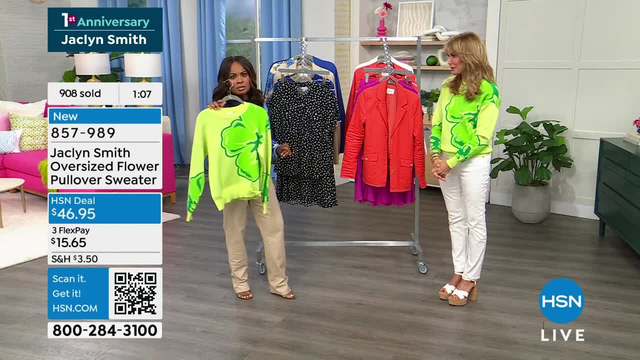 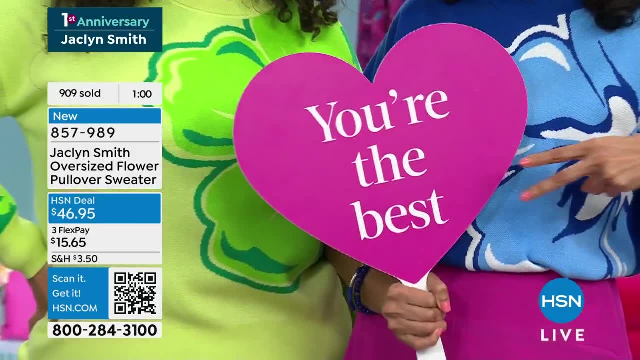 That would be gorgeous. Yes, You'd get tons of compliments. Right, And color is everything. Oh, I think You know you talked about, Well, color shape, Yes, Can change. you know the illusion and how you look in something. It can diminish areas you might not want to highlight And it. 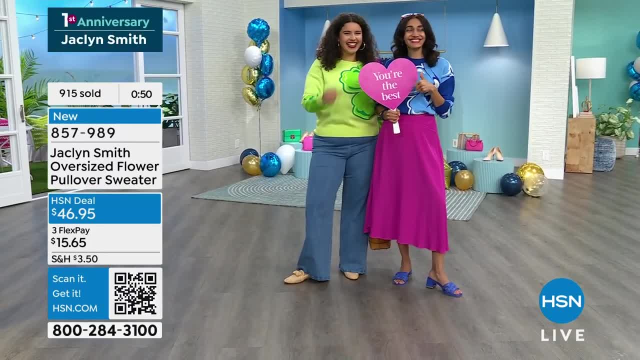 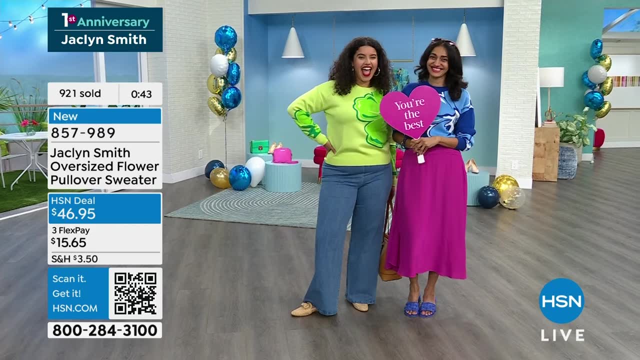 can highlight other areas. Yeah, All right, So you can see you're the best And guess who we're talking about. We're talking about you, You at home. We so appreciate you being an Asia Sun customer. Don't forget that. 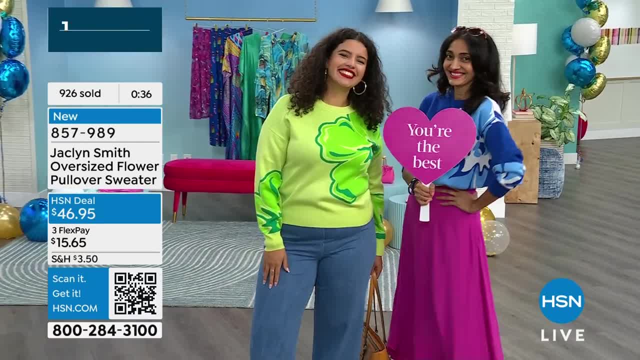 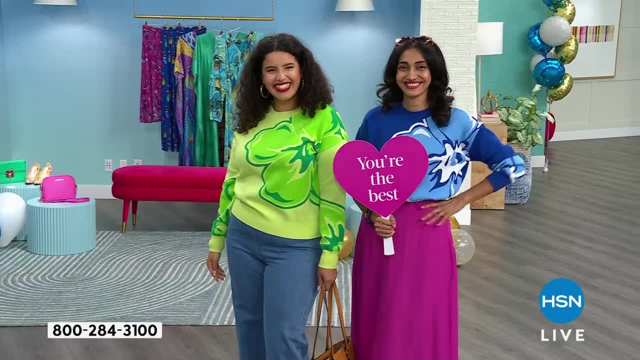 when you shop with us. it is our goal to make you happy. We do offer to you free exchanges, So if you get a garment at home and if it's the wrong size, or if you say, oh gosh, but I really wish. 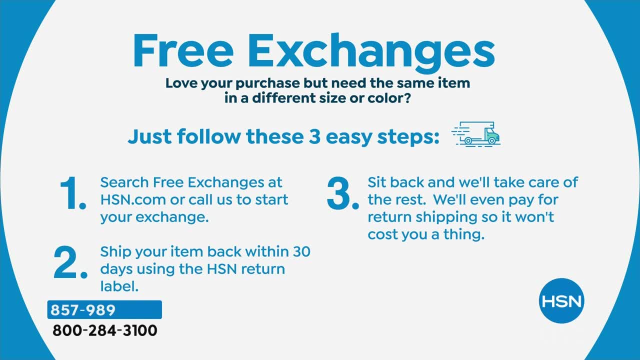 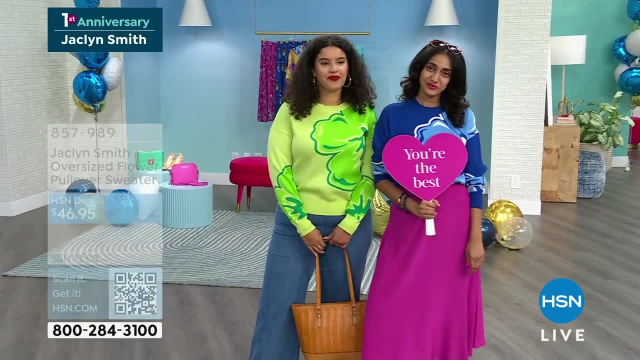 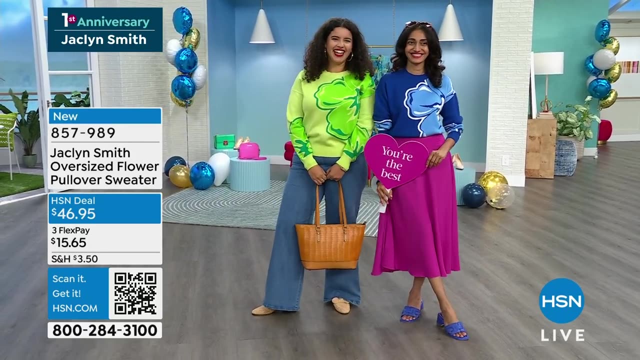 I had purchased the other one. If it's available, we'll be able to send it to you And it doesn't cost you anything. So just make certain that you ship the item back to us within 30 days using the ages and return label, And we'll be able to get it out to you. I'm so happy you found this sweater. Sometimes isn't a great treasure one little gold treasure that you find on the 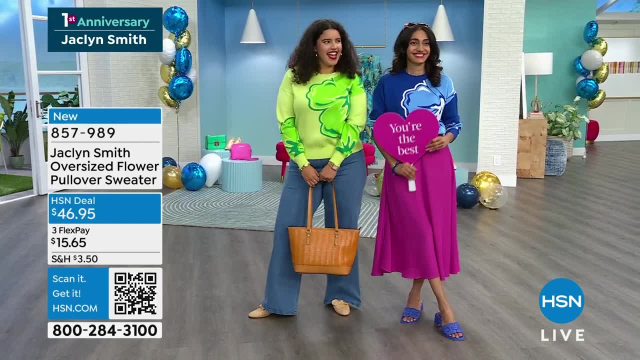 day And you're like, yes, that made that, it's made me so happy. That's all it takes for me, Just one, one, one special treasure. That's all I need sometimes, By the way. thank you so much for your phone calls. If you're on there in the ordering process, Stay there. 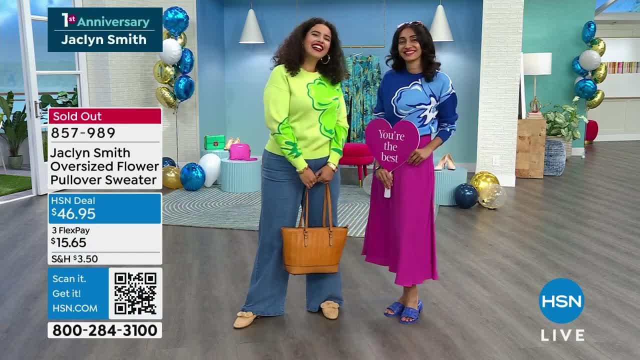 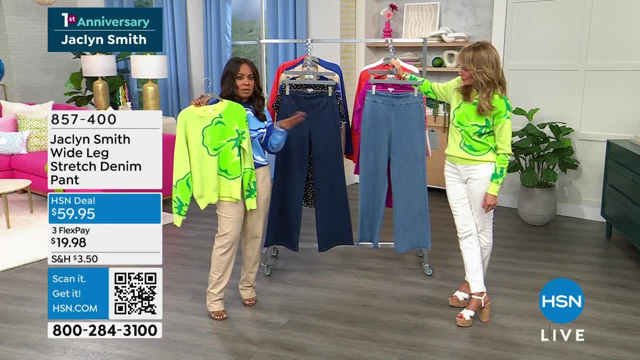 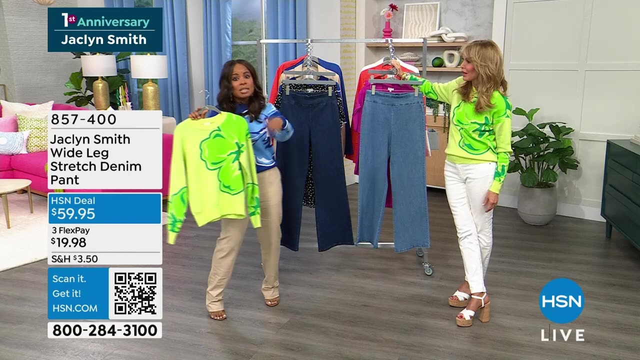 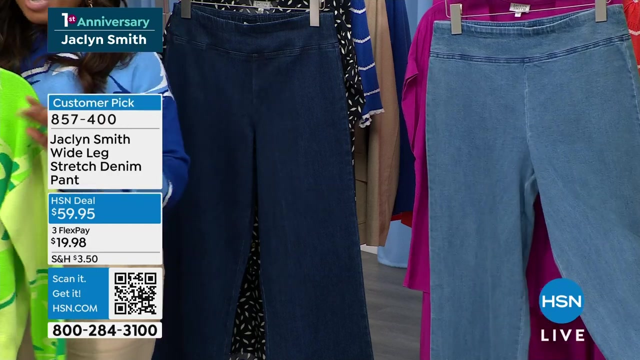 Next time don't hang up, okay. or if you're in the ordering process, don't don't check out. yeah, i mean check out, check out, don't stop your ordering process. what i, what i was trying to say: don't stop, okay, otherwise it's completely sold out. thank you and congratulations. i am not surprised that these are. 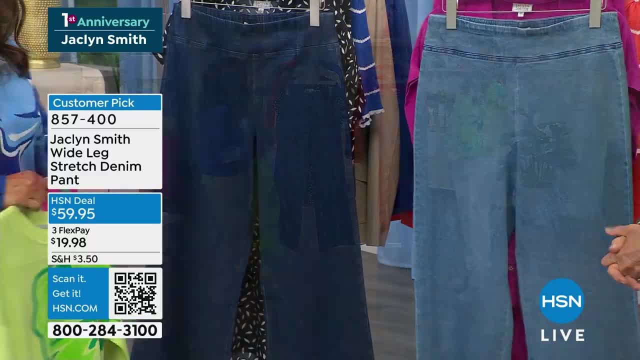 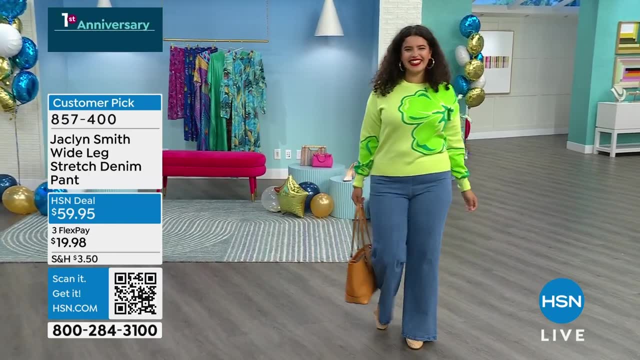 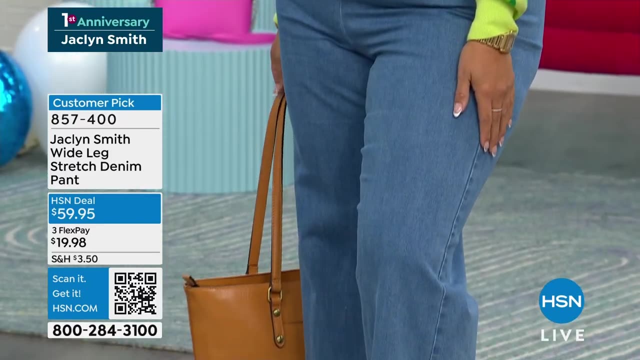 customer pick because, as i see them on every single model, they look so good they do on every, have made them a customer pick at home already. and it looks good with the jeans: linen, blue jeans, white jeans, a trouser- how good would they like? yes, so these are the wide leg stretch denim pant. 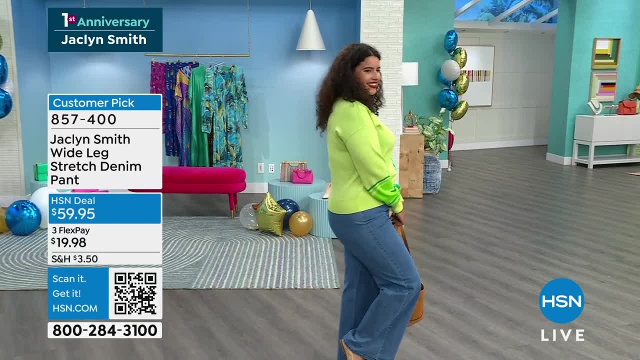 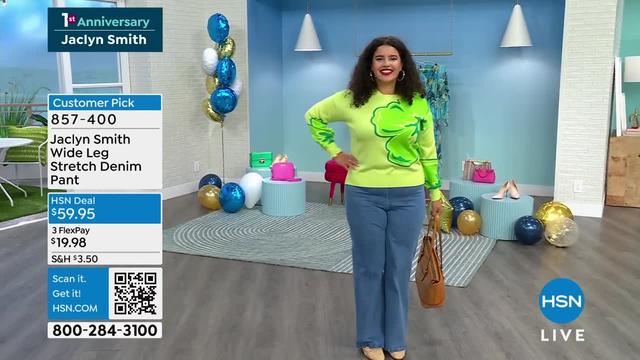 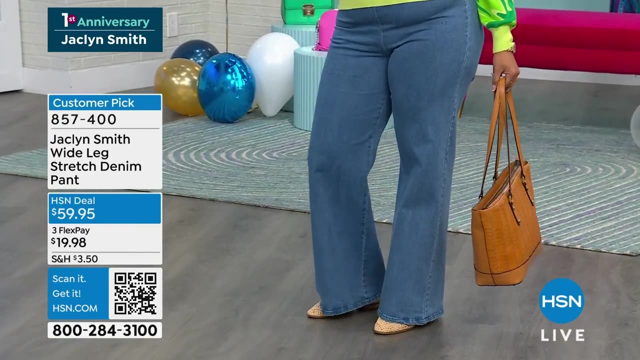 it makes me so happy that they're a customer pick, yes, so let me just tell you why. that means you saw them on one of our models, like miss natalie, and you're like: i like how those look, miss natalie or whoever the model was, and you decided to give them at home. and when you put them on, 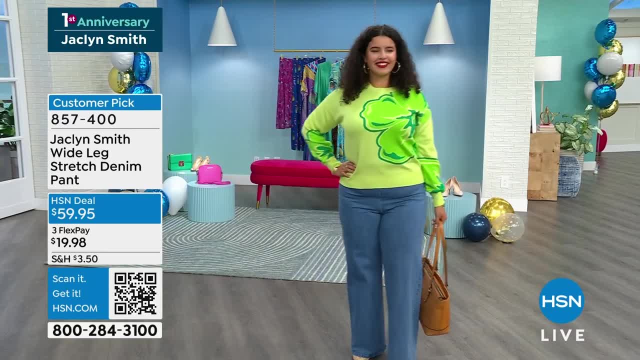 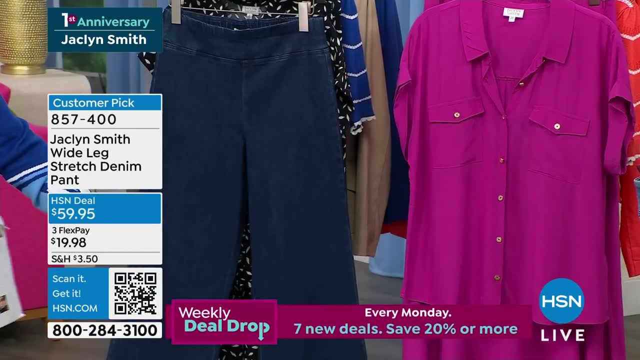 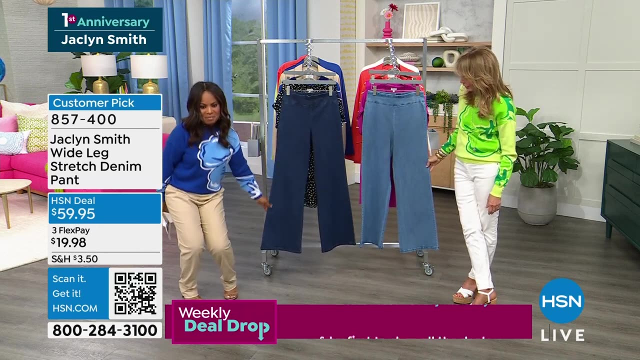 they look good on you too. that's right. they go on all sizes and shapes. yes, and it's so easy you pull them on. no zippers, no buttons, flat contour waist- which i fight for all the time, that signature flat, but look at how they're cut at the bottom. that's what i love. yeah, they're fun. 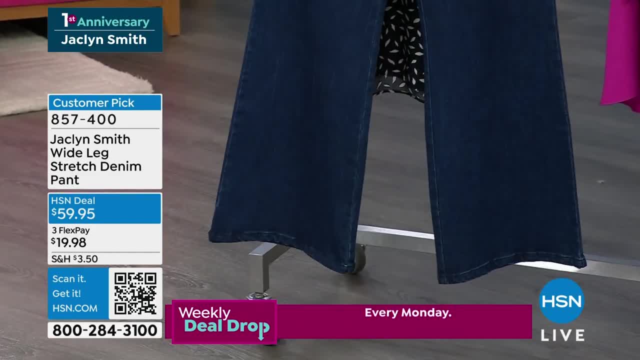 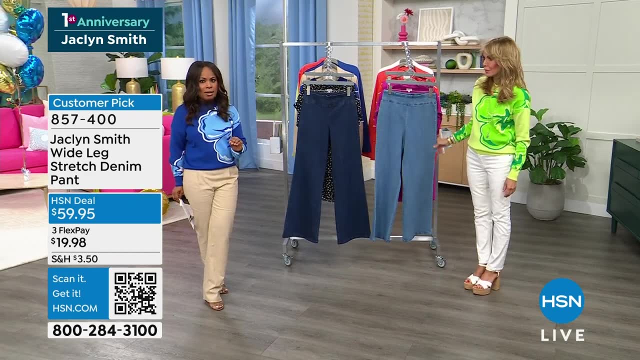 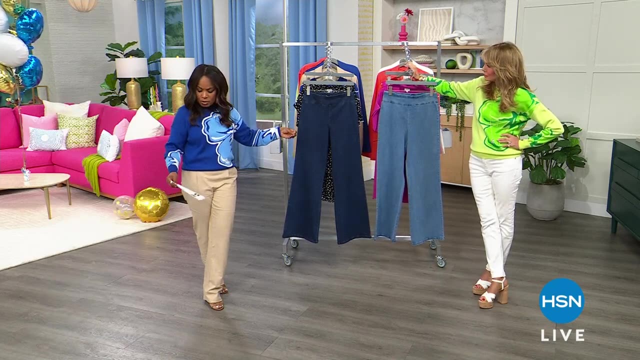 a little bit of flair, mind you, right. i'm charlie's angels, for sure, right, but i like that. it's not so you exaggerate, but enough to really give you that kicky, very modern, very of the moment look, which is what every woman desires. just let us know if you want the lighter denim or the darker denim. 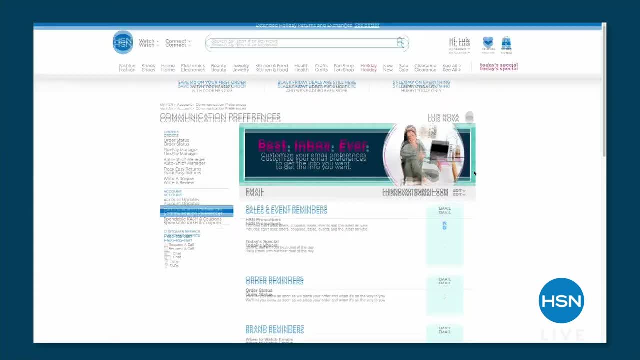 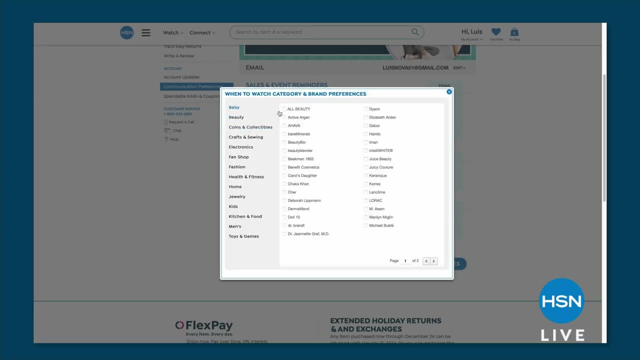 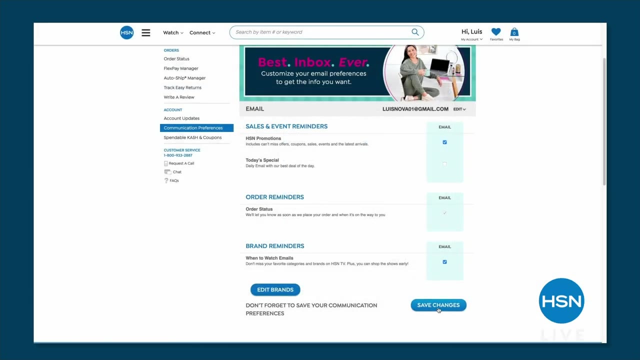 and we have every size extra small through 3x. let's talk about when to watch. i hope that you have fallen in love with the jacqueline smith collection, exclusively here at hsn, and if you have, be sure to sign up for when to watch, because we will email you whenever she's back on hsn and 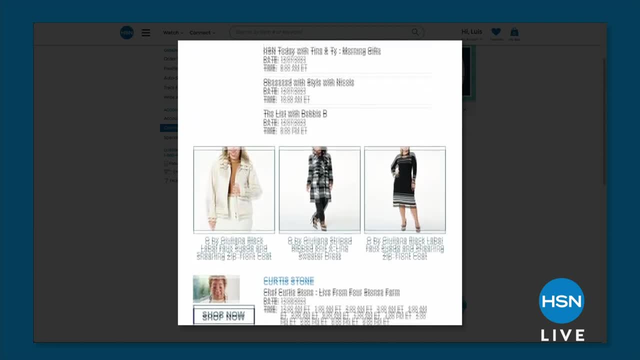 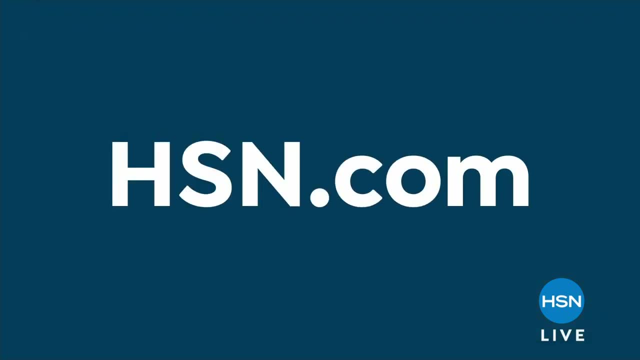 that way you can get more information about what's going on with the jacqueline smith collection. you won't miss any of her shows and, as you've seen for yourself, oftentimes when she'll launch a new piece it will sell out in just one earring. so do sign up for when to watch. we're glad you're. 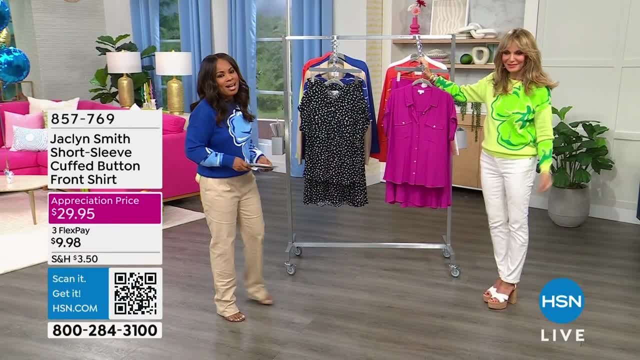 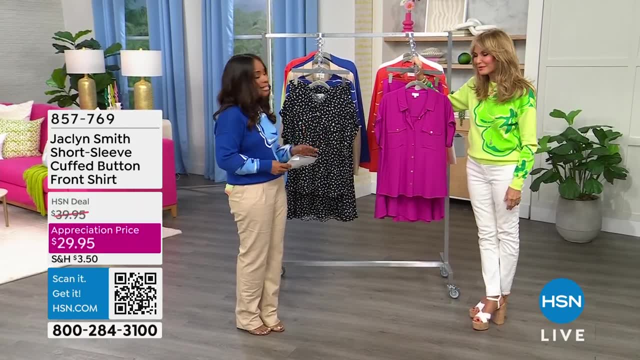 here. happy gotta watch thursday. uh, and of course, debbie d is coming up with the list, which is our big show on thursdays. um, and so we can't wait. they tell me you're gonna be out with debbie d, all right, so that's gonna be a lot of fun. 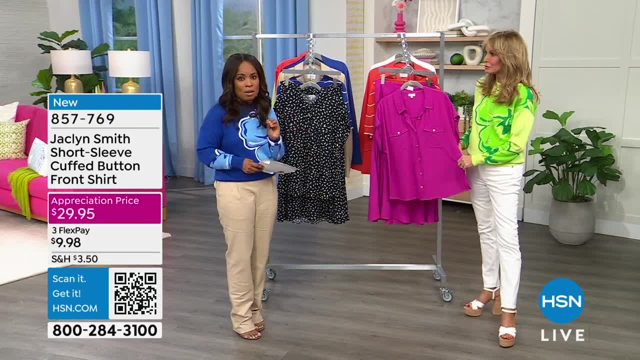 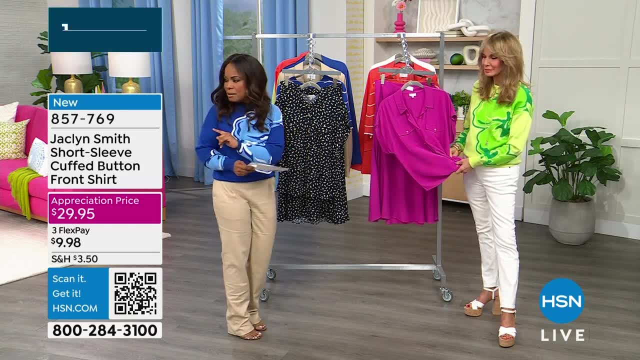 um, so don't forget debbie d, always at 9 pm eastern time with the list right here at hsn, and that's coming up tonight. but let's talk about this beautiful blouse. i know we gave a little sneak peek of this earlier and throughout the month, as we celebrate you, our customer, we're. 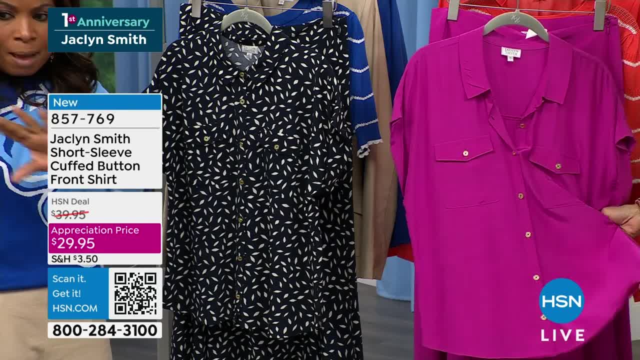 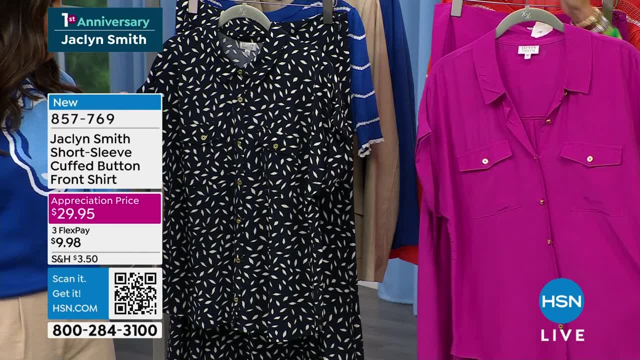 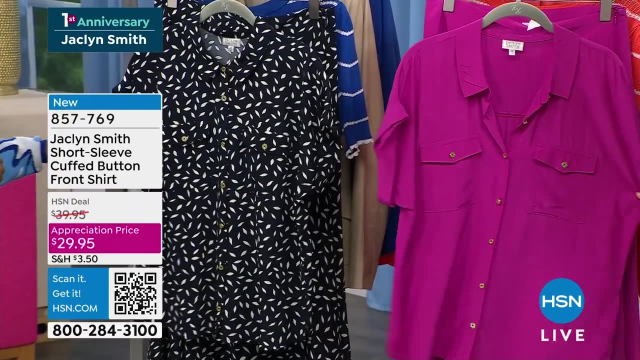 going to be sharing with you- and i want you to look for these- that pretty pink banner where it says customer appreciation. these are really, really extra prices, extra special pricing that we're doing. this particular blouse is a customer appreciation um price so i grabbed the wrong card. i'm going to 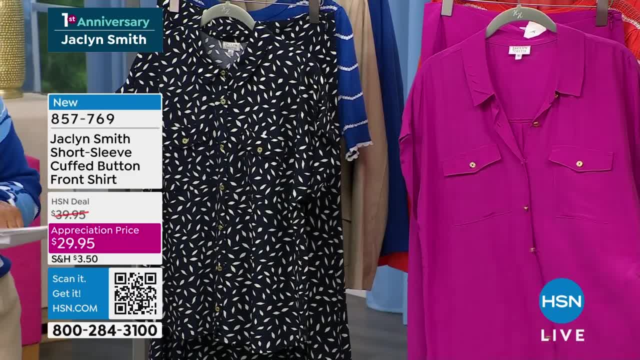 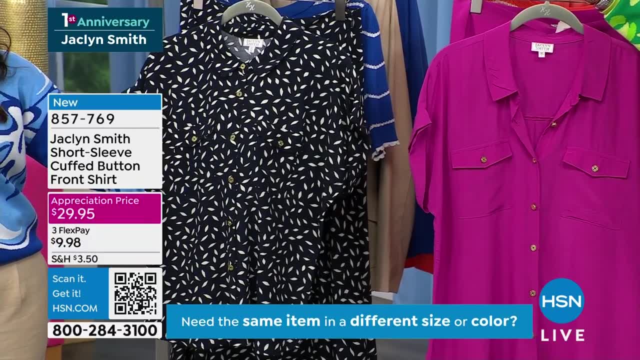 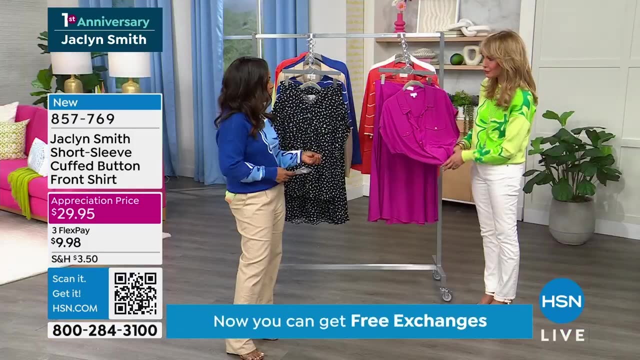 grab the right card to get the correct name. so we have night sky spectacle, which is the one that's next to me, at 29.95, extra small through 3x, by the way, 24 and a half inches in the length, and next to you we have fuchsia red. we're calling it fuchsia red, but it's fuchsia. yeah, it's fuchsia definitely. 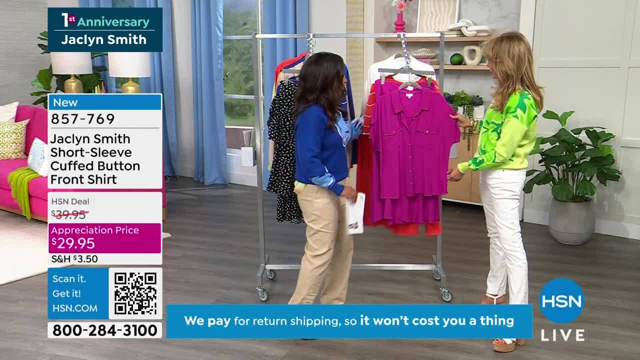 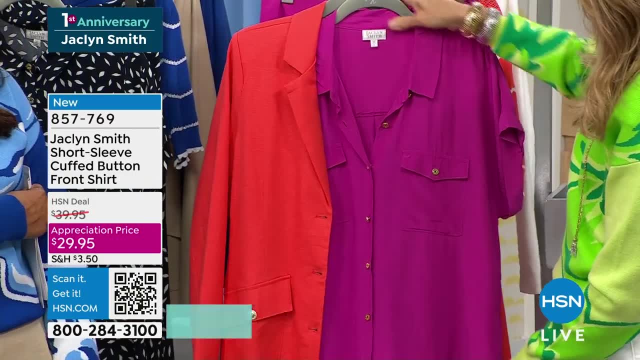 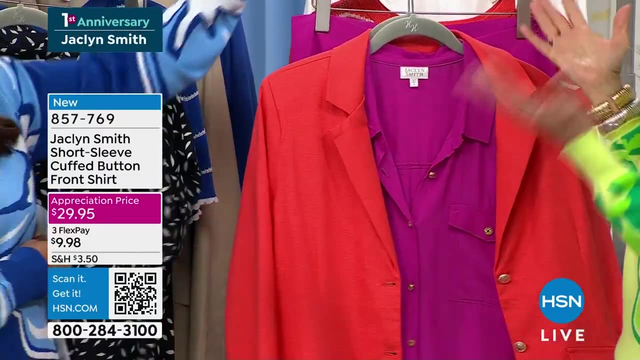 yeah, it's definitely. there's no red. and you know what, jacqueline, i know, don't think i'm odd. no, i know, i love the orange with the. yeah, it's beautiful that color combination. it's like pink with red, so fabulous together. i mean, the mix is a. marlo is going to go and order this blazer. 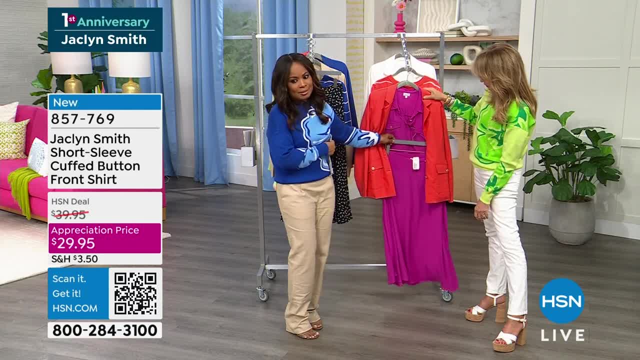 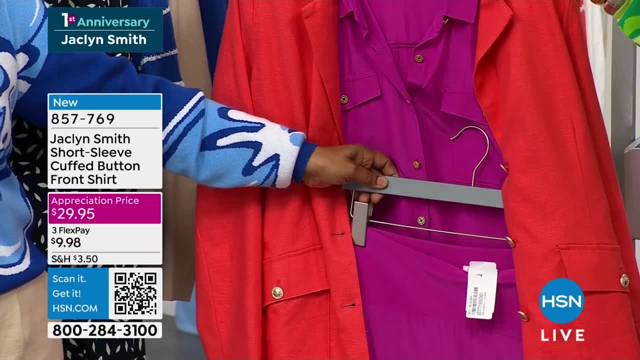 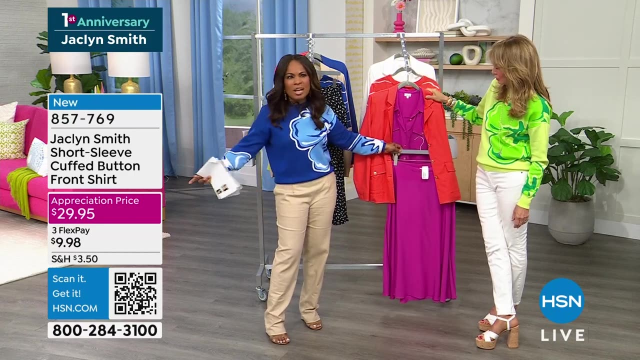 and i love the skirt. with this it looks great. i love that color combination together, really chic. yeah, that's how you pull off color. i mean i love color with the deeper, darker skin- me being from miami and florida- like i love color. put that on with the sandal and you look like you step right out of the magazine. 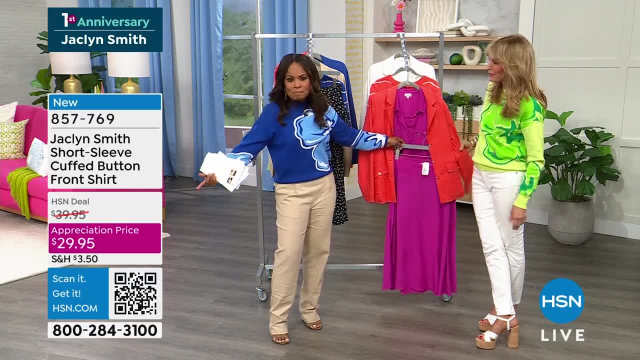 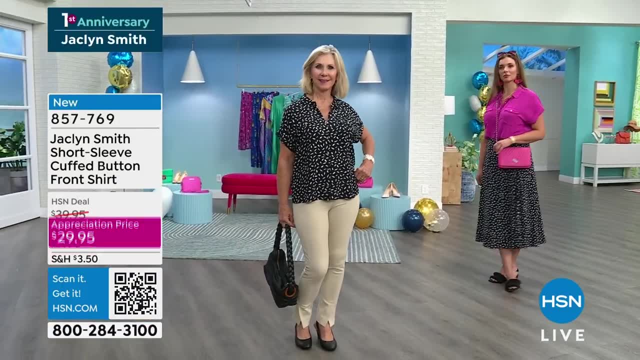 that's right. you're an influencer, you're a fashionista. that's how women, that's how you do it. you add these colors together and they, they look. i mean, it really is a plus, isn't that gorgeous together? it's just beautiful. and so the blazer. by the way, we're going to be giving you another look. 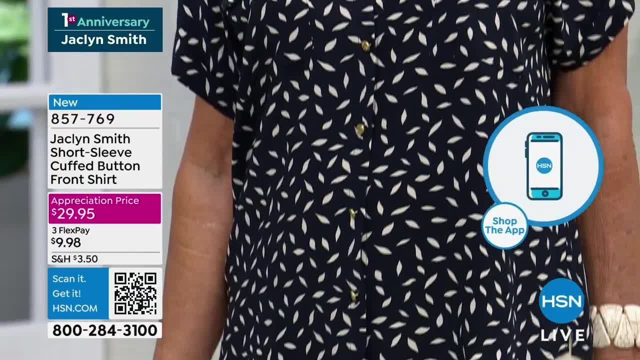 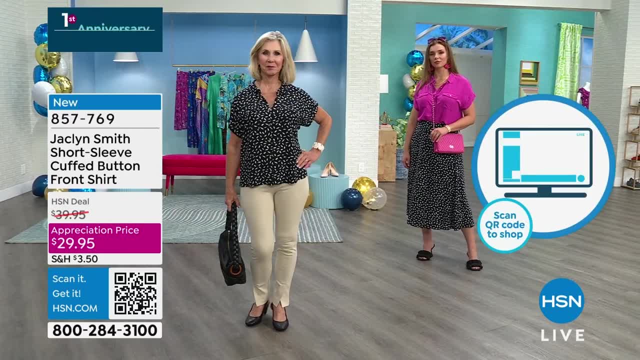 at. that's our weekly deal drop. but this cuff button front shirt, as simple as it is, i think really will give you, i think, a great example of the color combination that you're going to be wearing, and i think you're going to love all of the detail that you put into your pieces. i mean it. 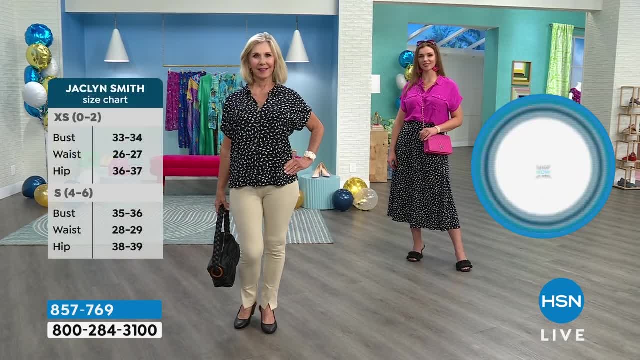 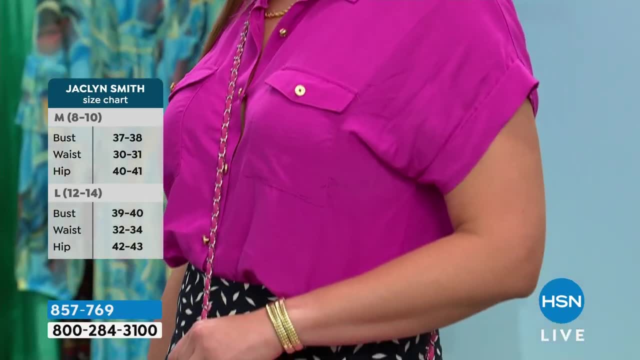 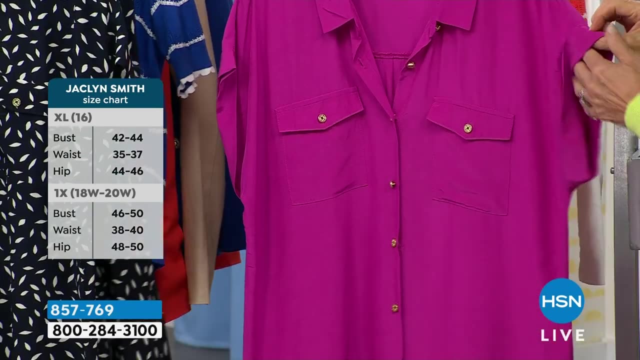 i mean, listen, this was inspired by a vintage camp shirt that i wore on charlie's that. i keep these treasured pieces. but this is a special shirt. it's a workhorse. it'll go a million different places. it has my go logo button that i love, and the angled cuff sleeves. we tack this. so this because 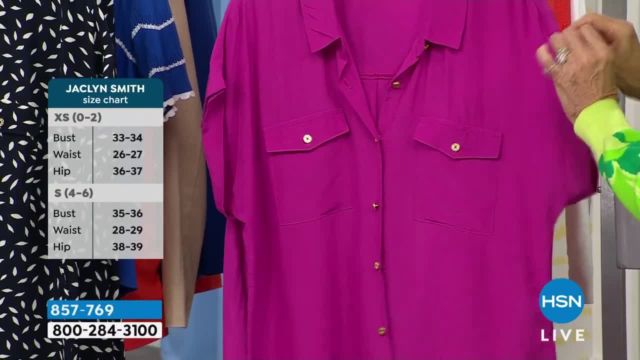 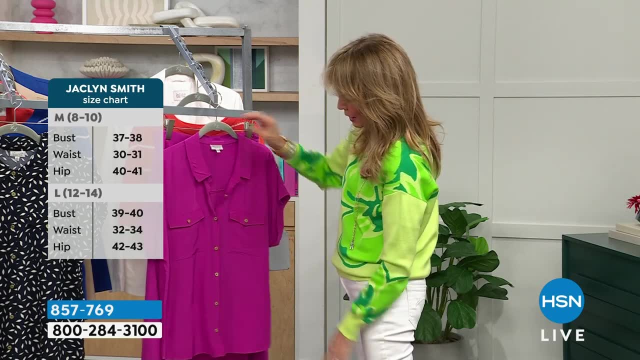 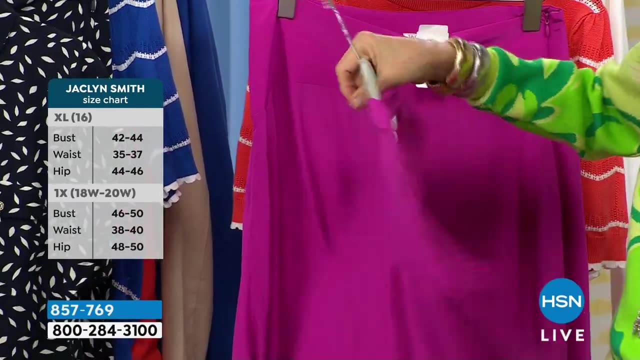 this is a very luxurious fabric. slick it could come unrolled, this will stay. it has an open collar that can be worn open or buttoned up pretty. the pockets were placed carefully to not add bulk and it has this back pleat which you know. if you're going to wear it out, you move easily. 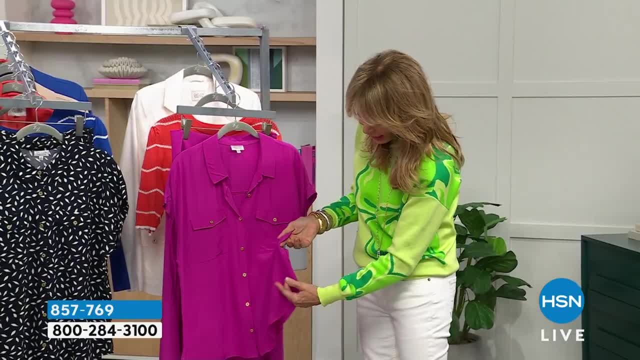 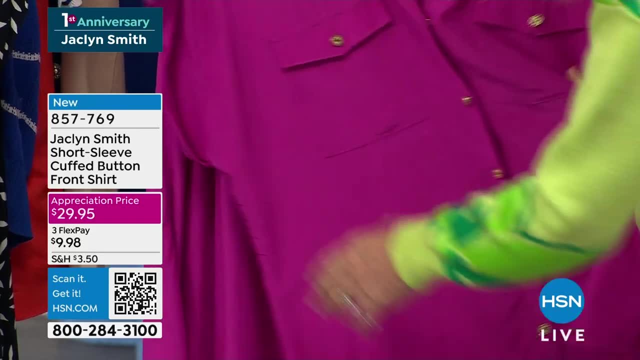 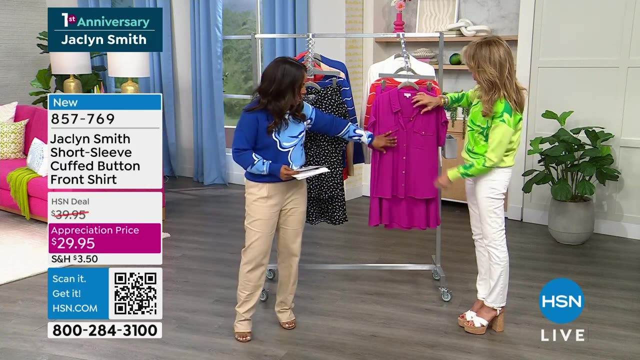 simple lines. it's easy to move in and the little side slit for an extra detail on fit. you see this little slit here. that's great. there's a lot, a lot going for this. it has some magic. it's not just a simple camp shirt and you can button it all the way, all the way down, and wear a little t-shirt underneath it. 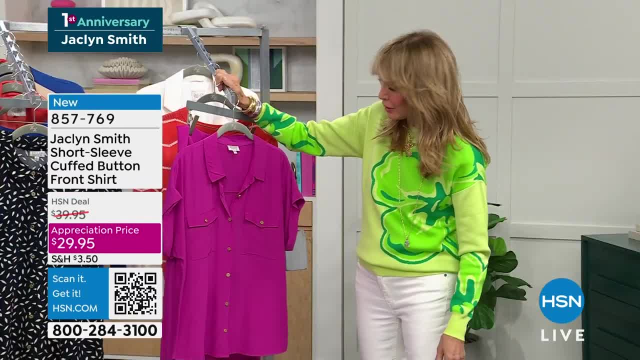 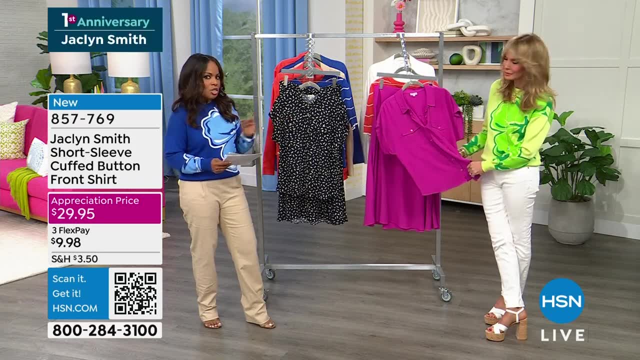 tie it, yes, tuck it in, or you can wear it as a piece over a tank. yeah, that's a great piece, extra small for 3x, 24 and a half inches in the length. just let us know which of the two is going to be. 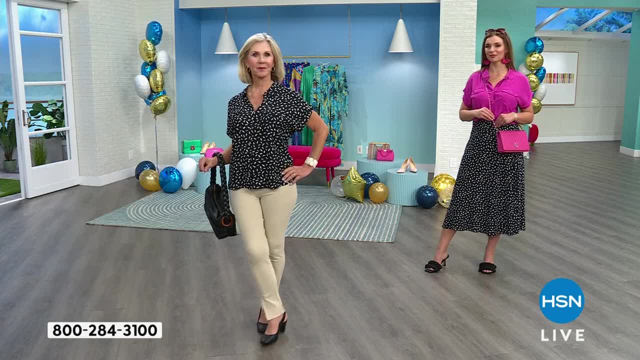 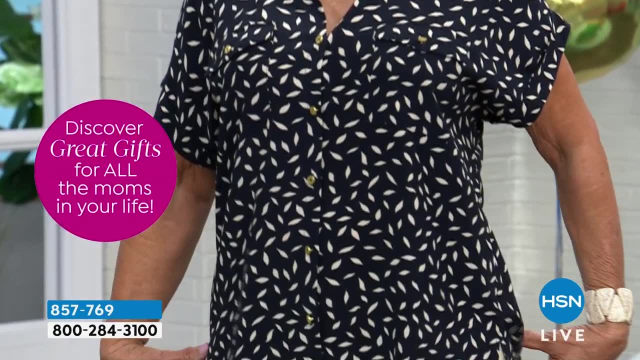 your favorite color and this one. i tend to favor that fuchsia. i just love the brightness of the fuchsia and it is such a pretty color. i love the way you did it. i just kind of gravitated towards that one. i'm like, oh my gosh, that looks so beautiful. 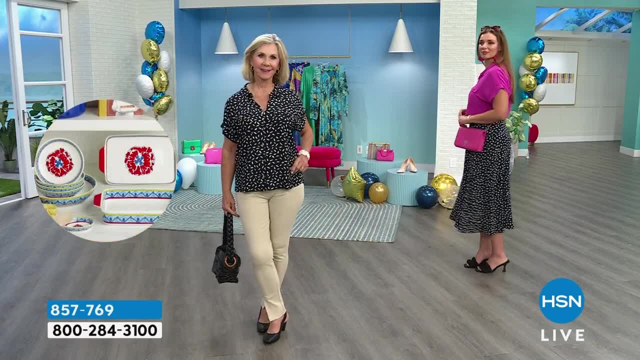 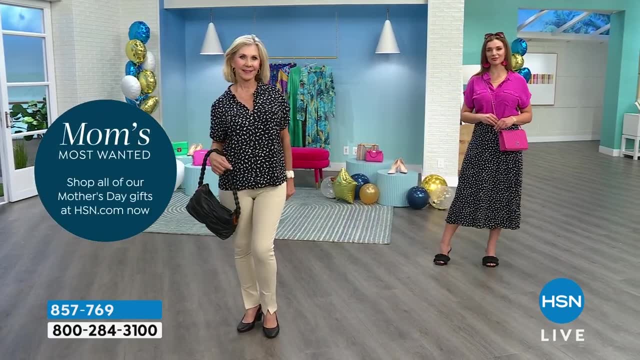 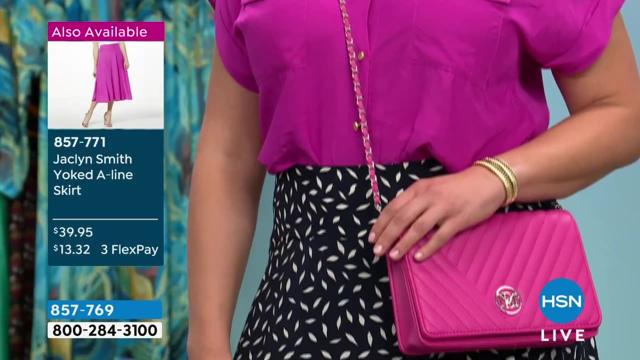 together. but look at what we've done here with both bonda as well as with our wonderful doug mara. so we kind of kind of pulled it off. we switched it up a little bit for you and as i see she- uh, the ponte pant there looks really great with a little camp shirt. the tan ponte, yes. so if you, if. 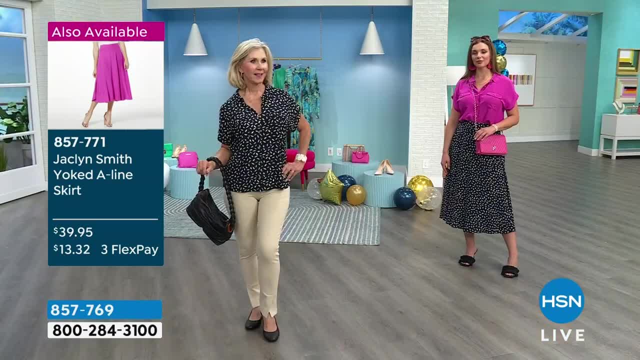 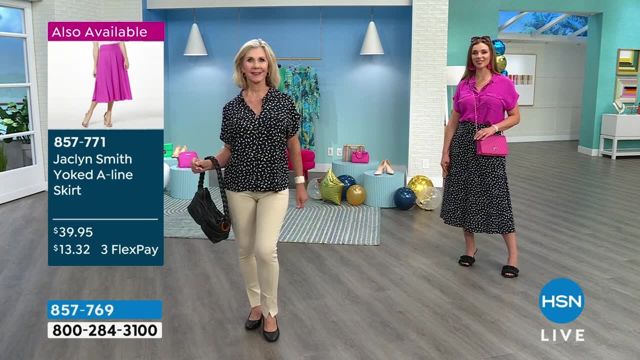 you do tend to wear, want to wear a pant or trouser, you can do that and i love how that looks, um with, of course, the other choice that we are calling the night sky spectacle and that's going to be, i would say, is that more of a dark navy. it is okay. 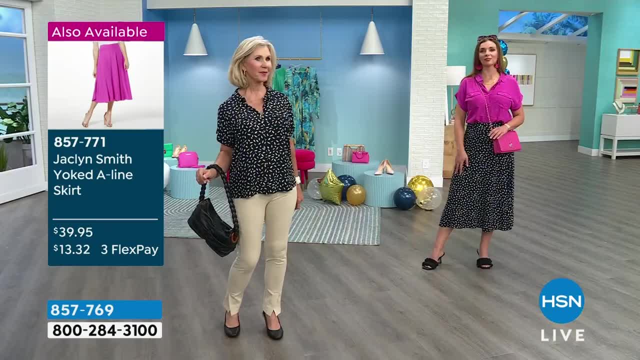 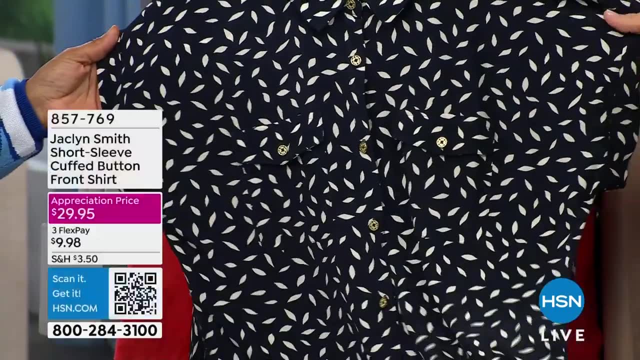 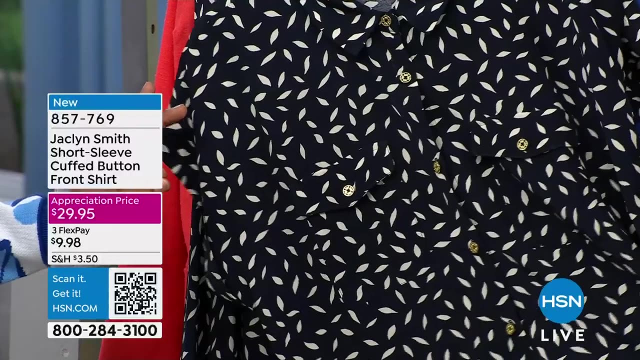 navy- i'm just thinking black, but it is a dark navy, i mean, and i would say an ivory, more of an ivory, or an off-white, not an optic white. it's pretty though. that print is very pretty and i love how the the print is small. yeah, polka dots are very popular and yes, but we didn't do the. 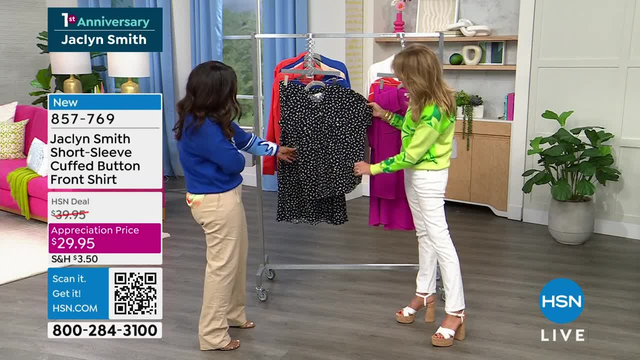 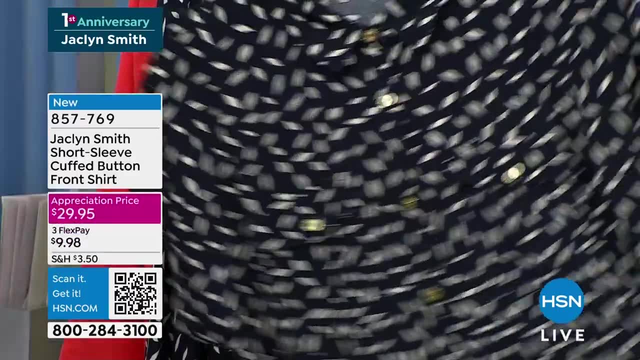 typical polka dot. we didn't do the typical polka dot. we didn't do the typical polka dot, we didn't. they did this little feather, yes, of uh, that's great, yeah, and the fabric feels like a silk, so this feels like you're in your nightgown and this, this would be beautiful just underneath the. 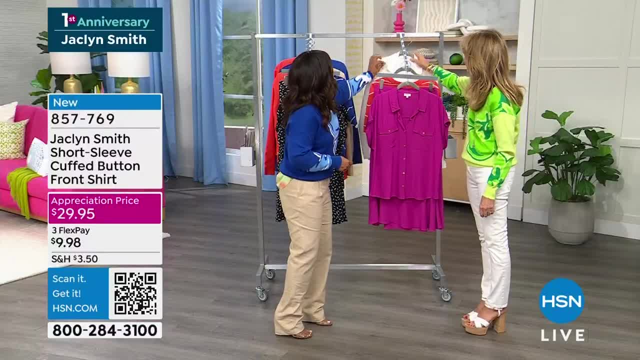 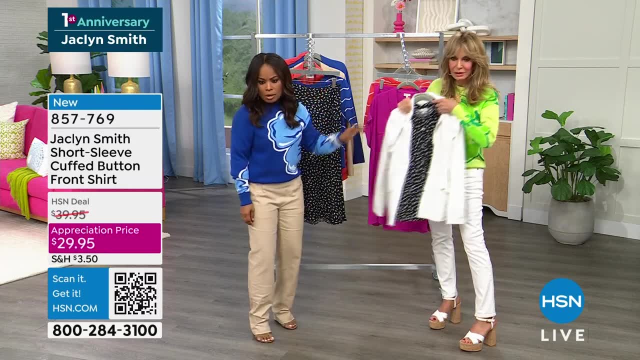 i would, even even with the white. oh right, wouldn't that be great underneath there. you know, if you just wanted to have a little pop, even my white jeans, you know, that would be terrific, that would be fabulous. i love that look would look beautiful. yeah, it looks amazing. 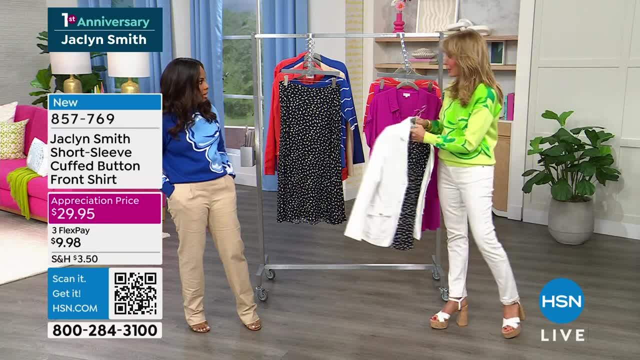 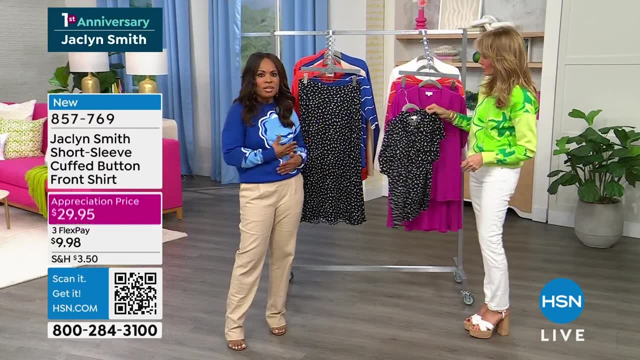 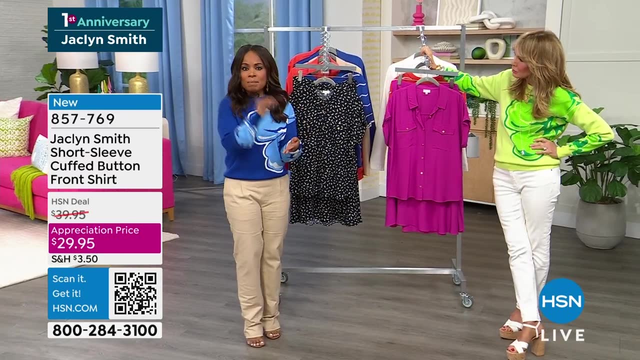 everything is interchangeable. That really makes your money go further and you build a wardrobe that way, And that's what I love about your collection, Like, if you just kind of are piecing the selections together, they just all work so nicely together And you end up having these pieces that are going to work and play well with things that you already have at home. 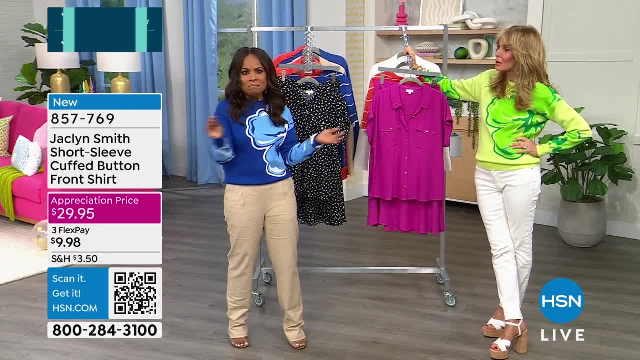 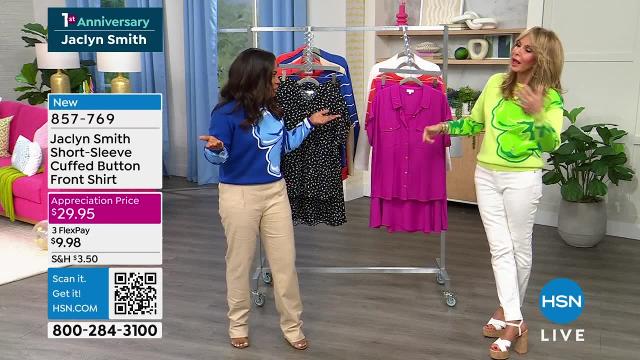 but that will instantly elevate your wardrobe And you don't need to even buy a lot. The blazer that we're showcasing that's. It goes with so many different pieces in my collection And it's a weekly teal drop And in the past, 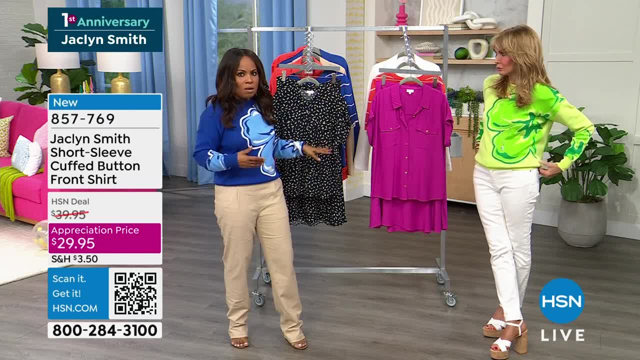 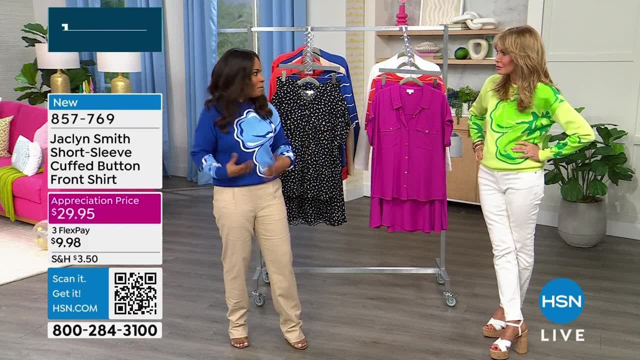 I would say that the sweater and maybe a blouse, and interchanging those pieces. you'd be surprised with how far those three pieces will take you, depending on how you're wearing them and what you're wearing them back with. It would be amazing for you. 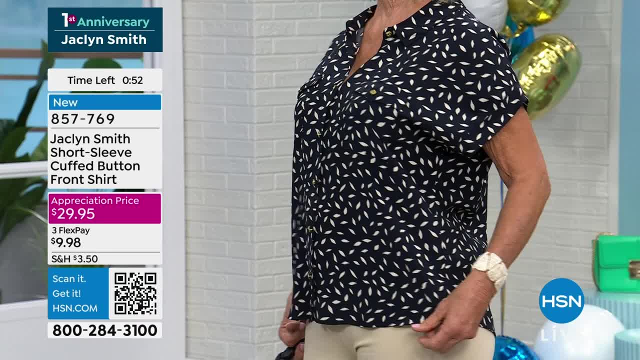 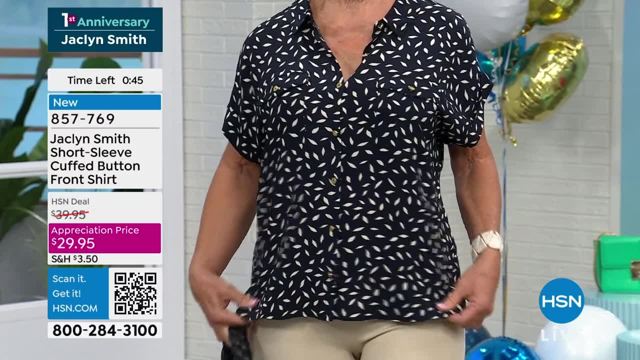 In the meantime, if you'd like to have this cuffed front sleeve top, I do want to let you know that our incredible Vonda happens to be 5'6". That's her height. She is wearing this in a small. Her numeric size is going to be: 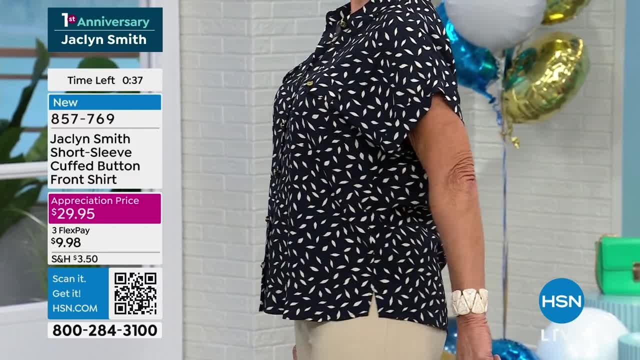 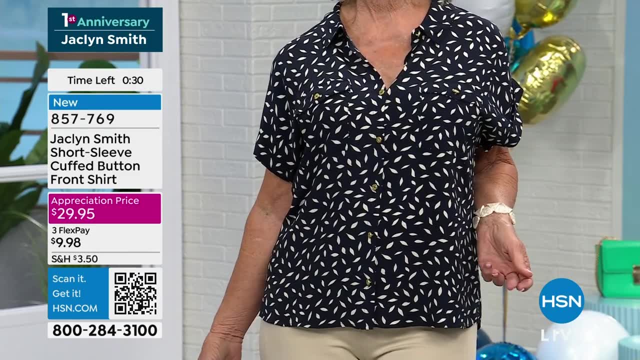 5'6". She's wearing it untucked. You can see that tiny little slit on the side. Notice how this does cover the upper arm, the flattering V-neck and how it falls beautifully on her body. Height-wise again, she is going to be 5'6". 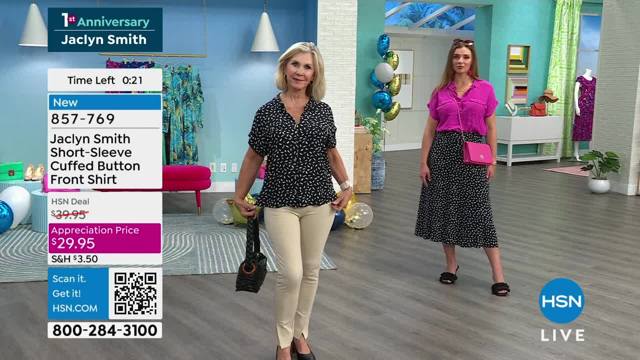 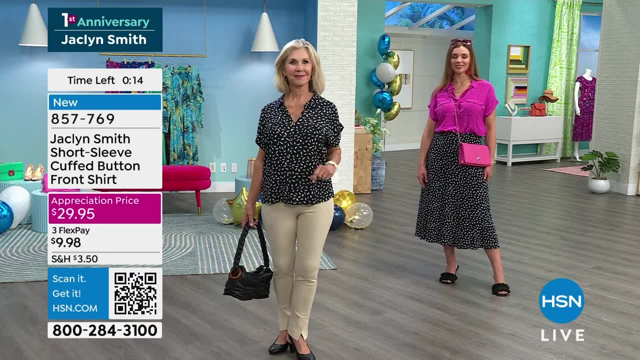 And the top is 24 1⁄2 inches in the length. She's wearing it, of course, with the ponte knit pant that is available. You can shop that pant on hsncom. I have to mention also, you're looking at less than $10 on any credit card. 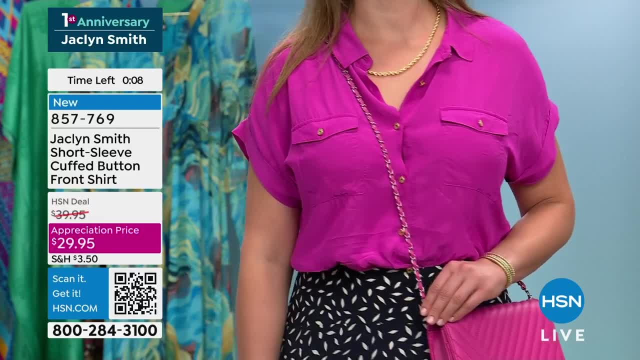 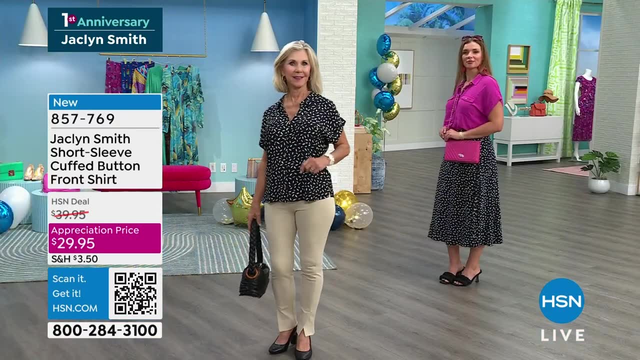 because this is offered on three flex pays. And then there's going to be the fuchsia paired back with the night sky skirt, And we're going to talk about that skirt right now. Yes, and the secret weapon is this contoured waist here on this. 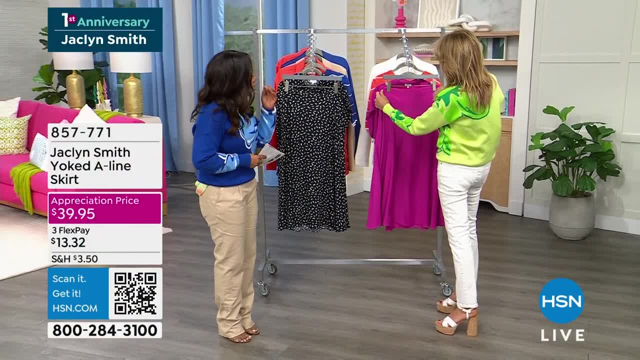 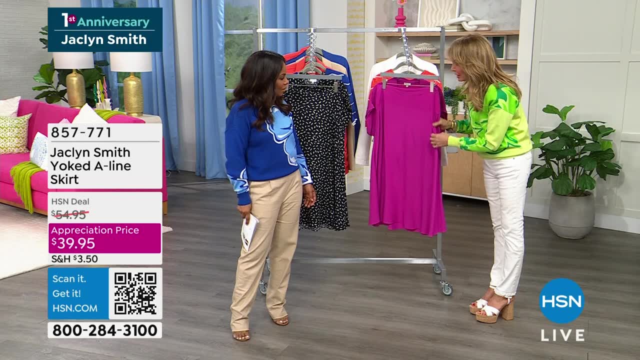 It's double-faced fabric here, So it's flattening but it's not confining And it has a little side zipper, but almost individual. I mean invisible is what I mean. You don't really see that. That's really beautiful. 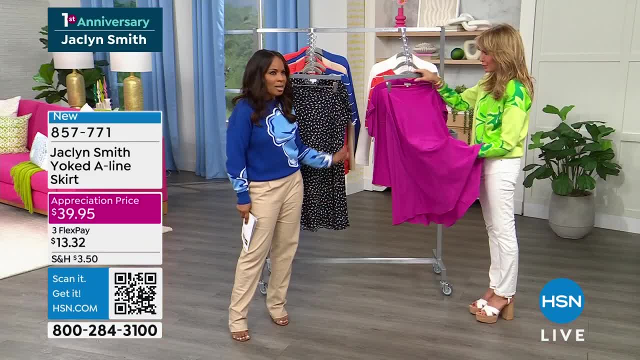 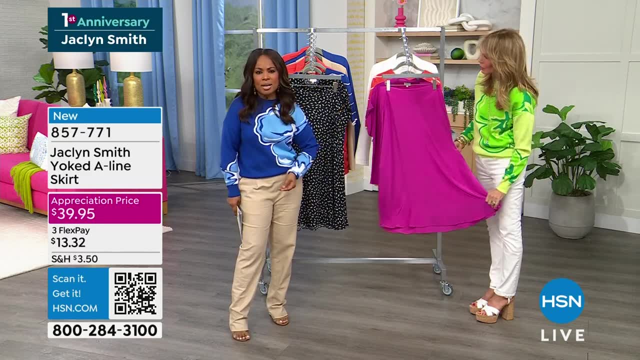 And you know that it's unlined. It moves with you, It sort of dances with you. Yeah, I love this. It has fluid. I love it. It's so feminine. I mean to a shower, to a banquet. 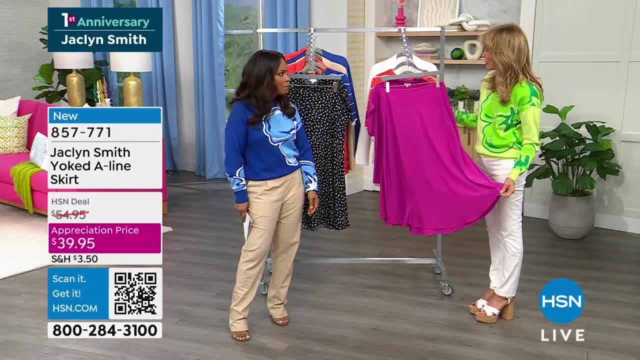 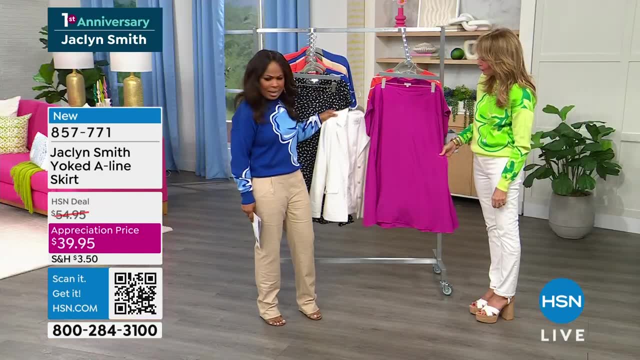 To a tea, to a party. It's beautiful And you can wear well- I love fuchsia- with black, with navy, with white, Even with- I was going to say even- with white over it with the white blazer. 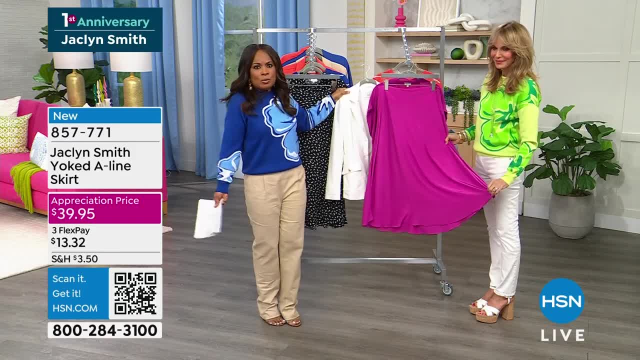 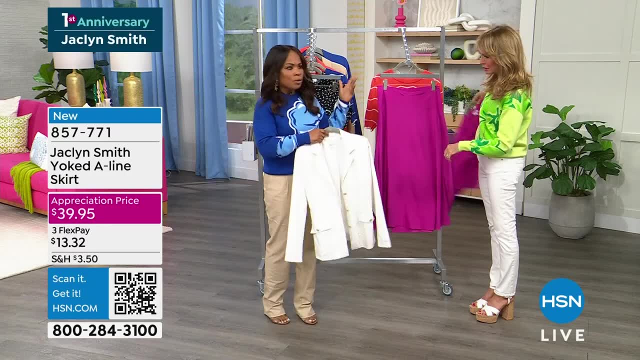 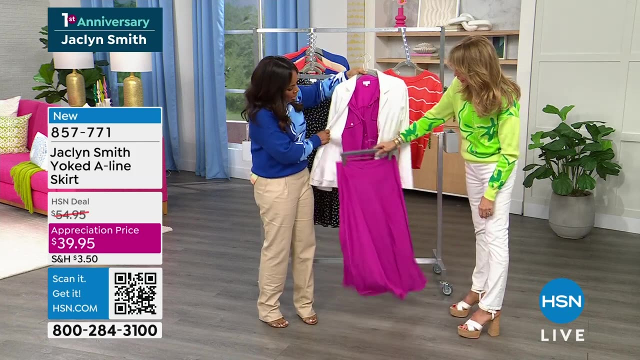 Yeah, You would look gorgeous. You step into that banquet or you step into that conference Here, let me put this down. Let's show them, Okay, Because I know your lives. you are leading such wonderful lives And when you are looking for, I mean, just think about how beautiful you will look. 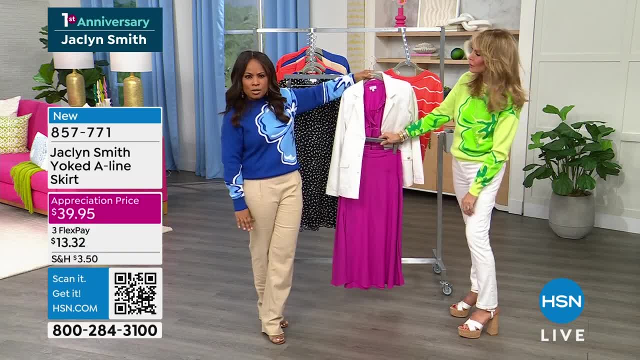 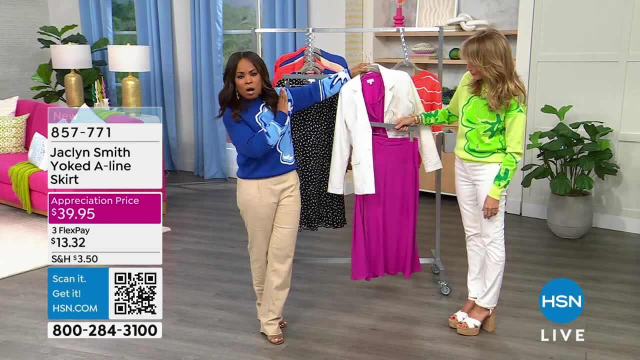 Wear it to church With your gold jewelry, your bracelets. a pretty shoe, Really very feminine and refined, Yes, And elegant. It's timeless. Yeah, you'll look gorgeous, And all the pieces are being offered on FlexFay, which is really wonderful. 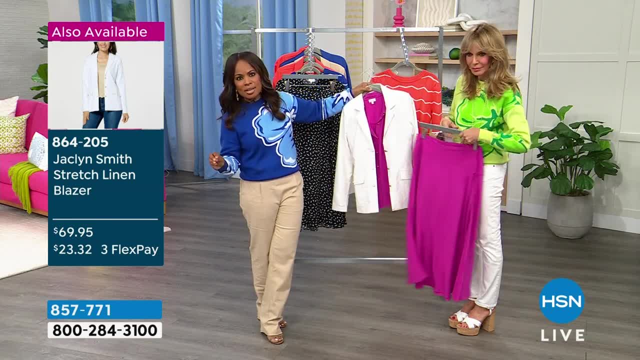 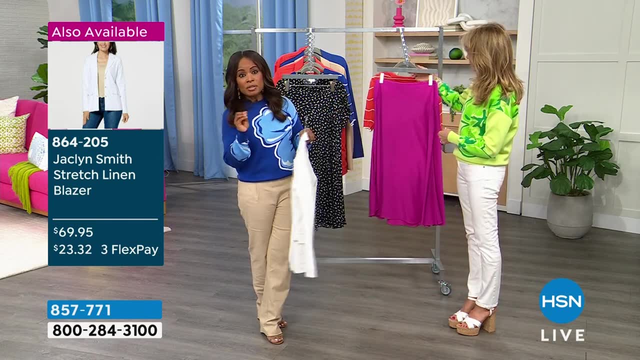 Because with FlexFay, we ship it out to you immediately. You still have to wait, You still have 30 days to be able to pay for it And you can probably get all three of these pieces at home today, I know for sure, for less than $100 on the FlexFay when you're using them. 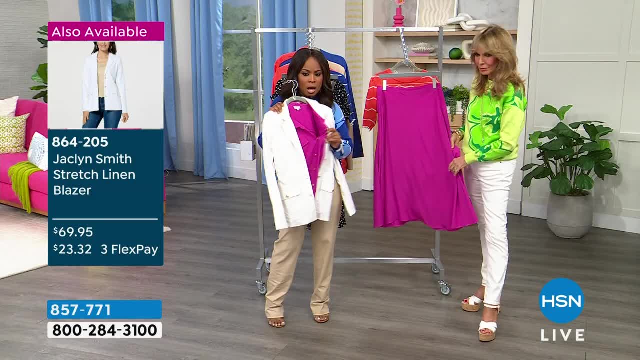 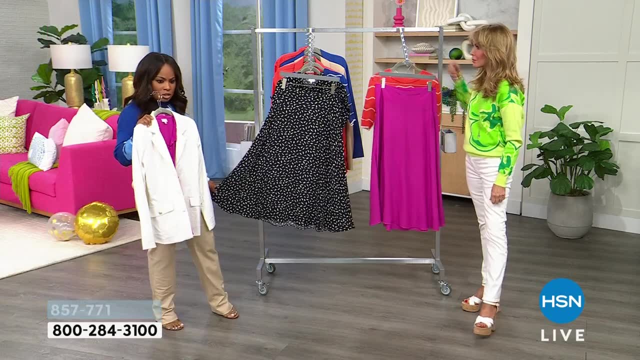 We are going to be talking about the blazer in a matter of moments. The top we've given you a look at, But the skirt, I'll give you all the information. You can see it has that little bit of a flounce, just a little bit. 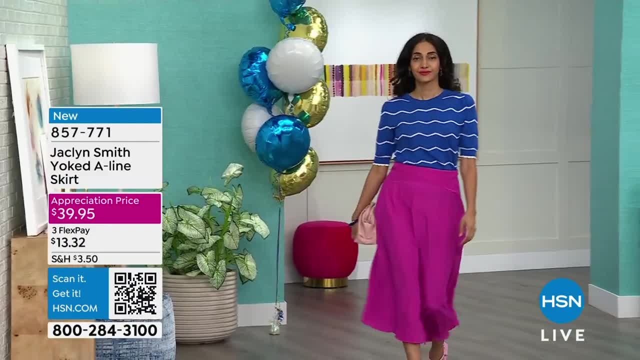 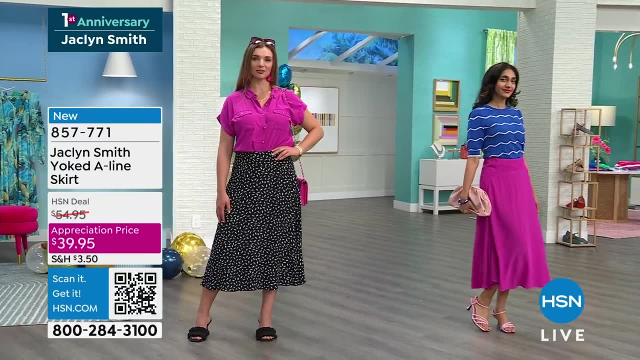 Under $60. And my jaw dropped when I saw the price on this skirt. Wow, Look at that. That looks $39.95.. It looks like a rich Fuji silk The skirt does. That's beautiful if you can grab that. 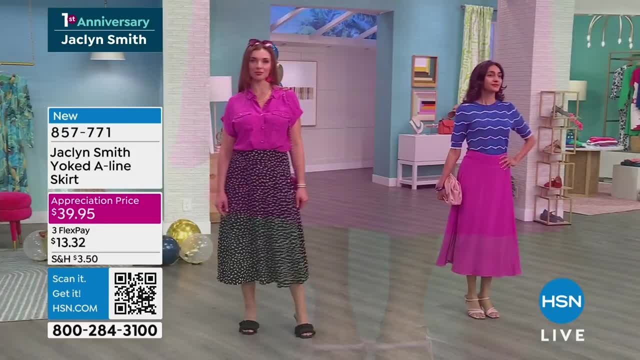 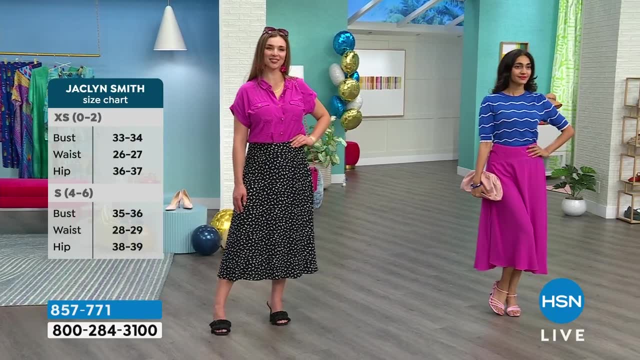 That would be pretty enough even to wear to a wedding, Absolutely, You know. and that fuchsia color, If you're pairing them side, you know, top on bottom, tonal. I like it as an ensemble. Yes, together It would be phenomenal. 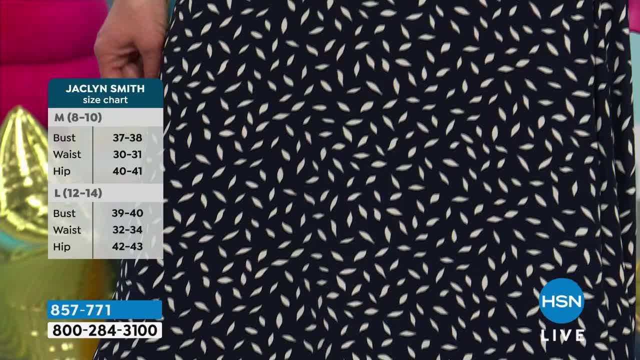 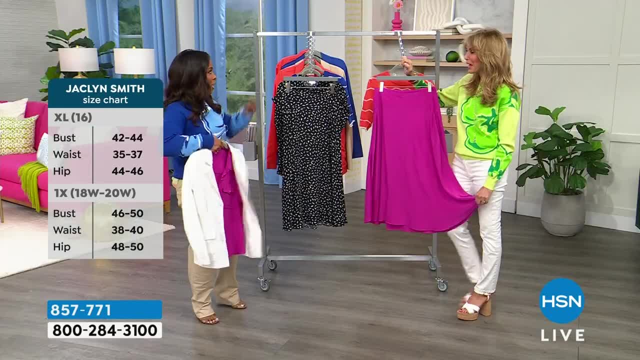 If you're not afraid of color, I might invite you to get that ember glow jacket and put over the fuchsia. That's another one I know, And unexpected. I'm going to show you what I'm talking about, I know. 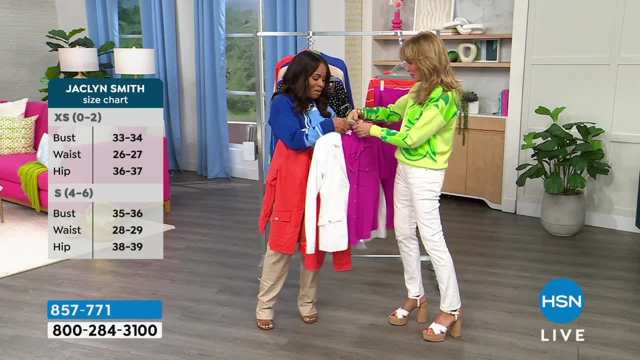 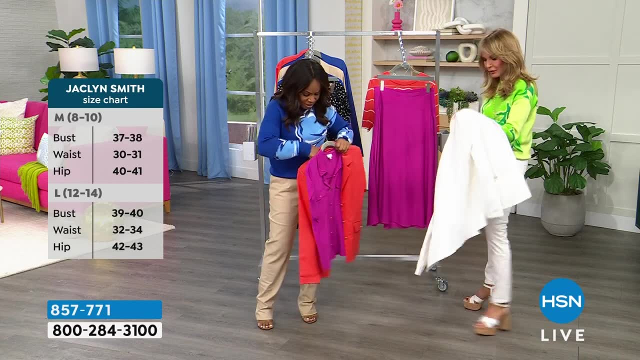 You're like Marlo Marlo, But it's true, Marlo knows Marlo, I'm going to follow your lead. I've learned a thing or two, you know being here, But this- if you're not afraid of color- would be incredible as well. 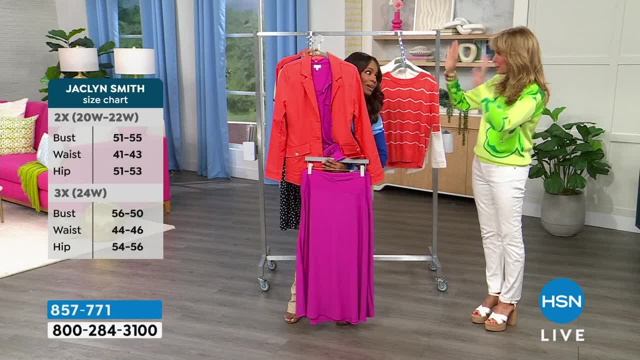 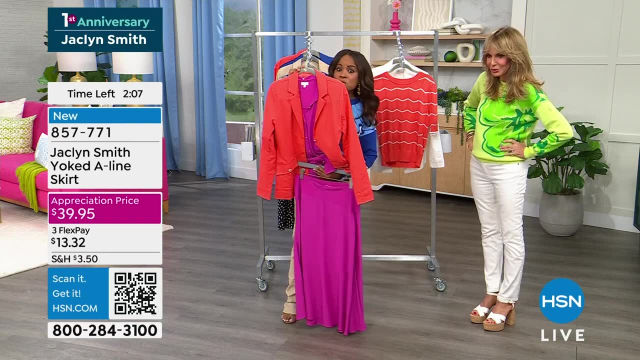 It's great. That would be phenomenal. It does look like a page in Vogue. That's how I would wear it Me. It's such a signature. Yeah, I love the color. with the color I do too. You wouldn't think to. 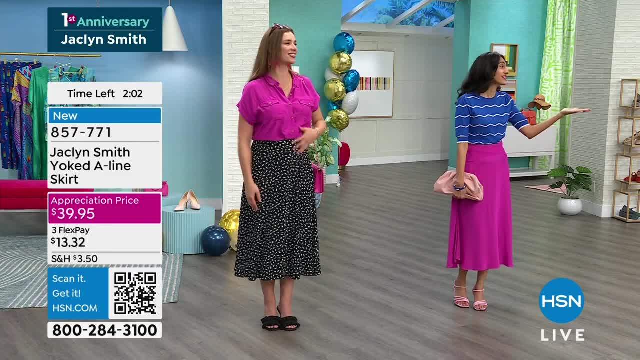 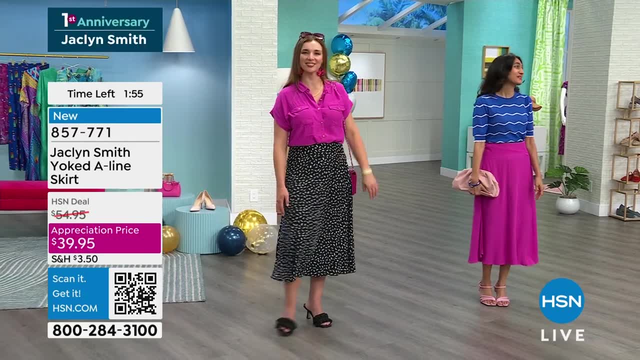 You love this too. I love it, I know, See, It reminds me of India. Yeah, Yeah, Where I just came from, Simi said it reminds her of India. Yeah, Isn't that phenomenal, All beautiful color there. 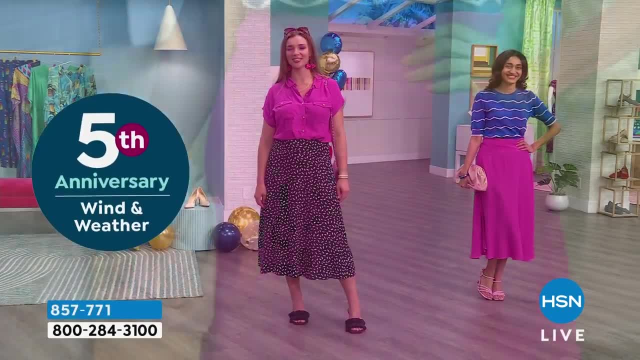 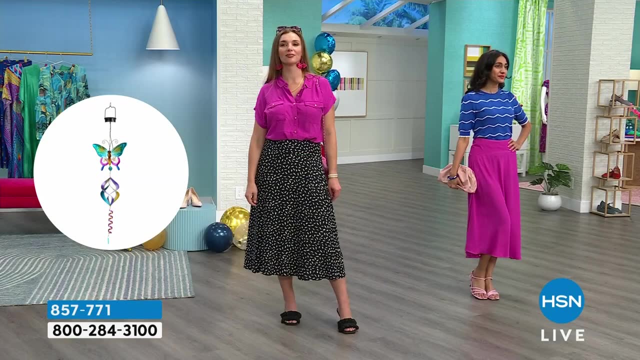 Yeah, And vibrant colors there. That's my favorite combination. I think it's mine too. Yeah, Thank you for that. Yeah, It's just beautiful together. It is, And any restaurant, An individual. You're not going to say, oh, I've seen that. 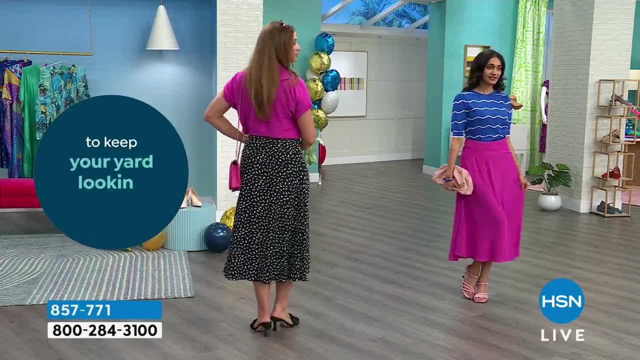 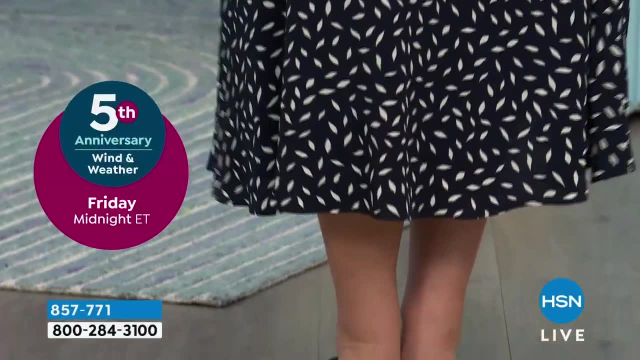 Exactly, Exactly. It's very unique and special. That's what Marlo, as your personal stylist- Well, you're very good, Marlo. I'm putting you into that one. Try it, You know, if you don't love it when you get it at home. that's why we give you the 30. 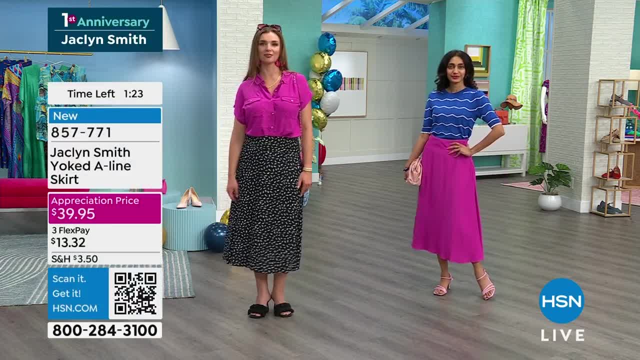 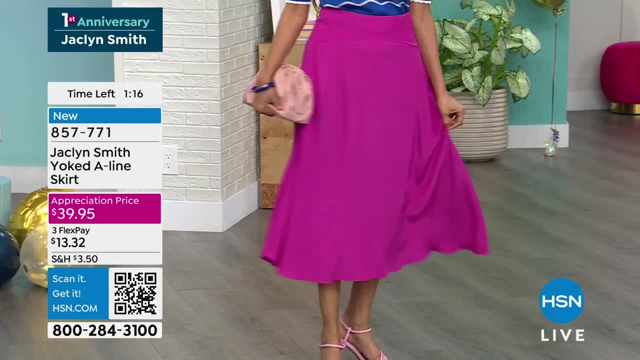 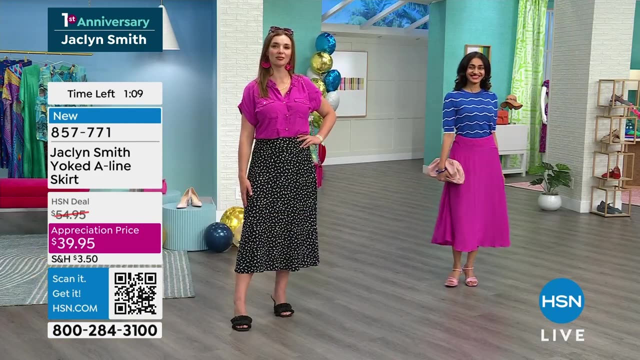 days. But I love that you have this fashion democracy, where we have these beautiful pieces that make us feel confident as we present ourselves to the world. wherever you may go in the world, And you're not breaking the bank, but you look. You look amazing in every space. 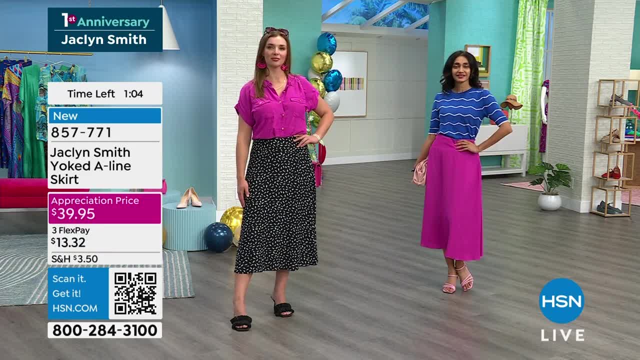 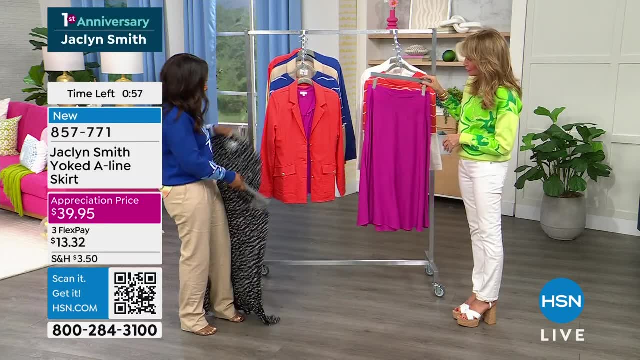 You look just as beautiful as the next woman, Comfortable in your skin, Yes, Yeah, Yes. Where you walk into the room with confidence, They're just beautiful. And the same thing is true even with this. Ah, I love this with the beige. 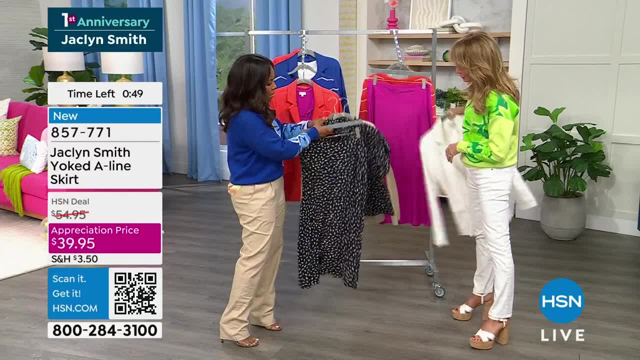 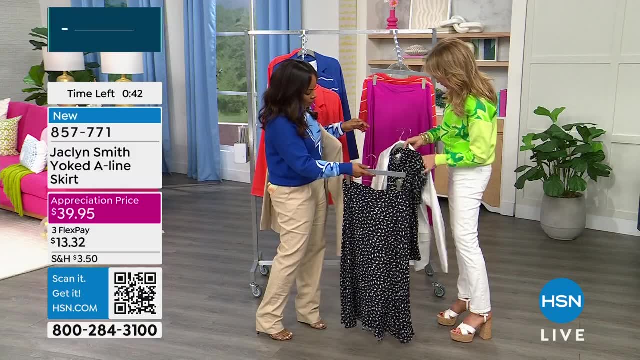 Yes, Or the white, Or the white, Either way. Either way. Here Let's do it with the white, I think, first because I think that pops. Yep, Looks great, So pretty, Yeah, And buttoned up. 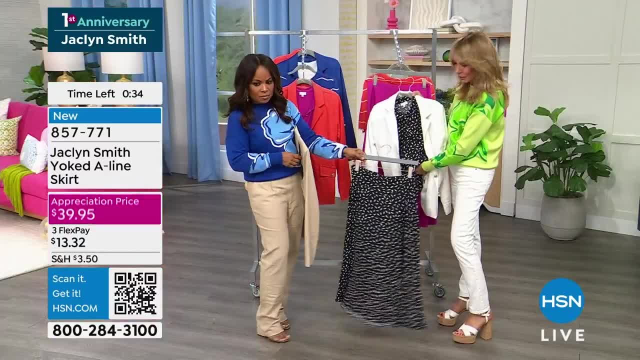 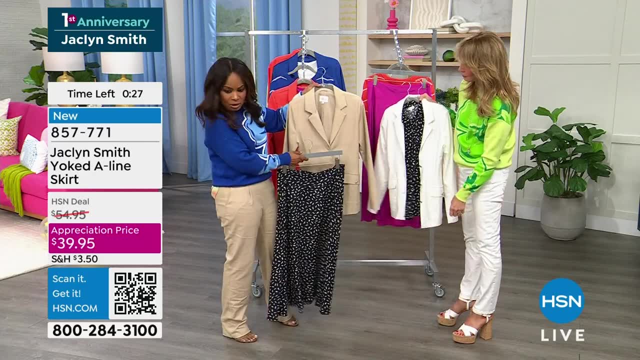 Look at, how great Doesn't that look? great, Looks, terrific. And then if you're doing it with this skirt, It's really a nice ensemble. You can do it. Or if you want to kind of pare it down a little bit, you could do a little bit more casual. 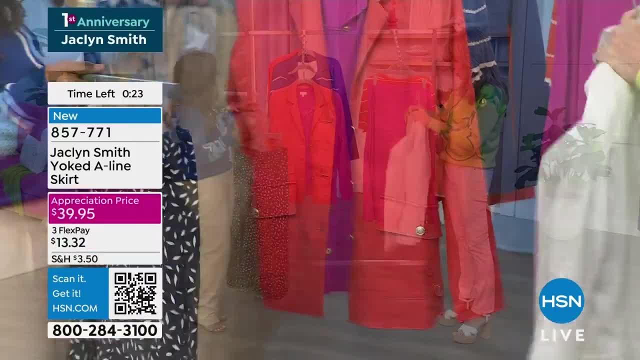 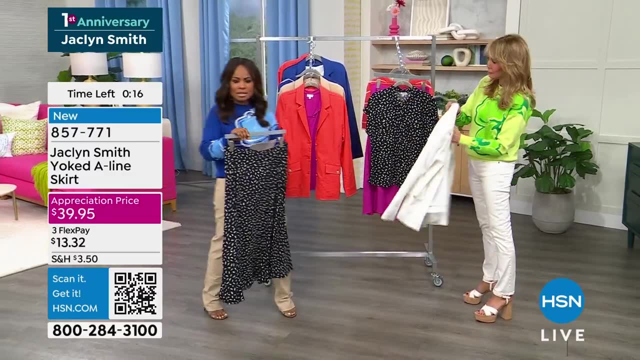 even with the beige. So totally, So many ways to go, which is what we want in a collection. Yep. The skirt, by the way, is 34 inches in the length. Don't miss it. That's a great price for this skirt. 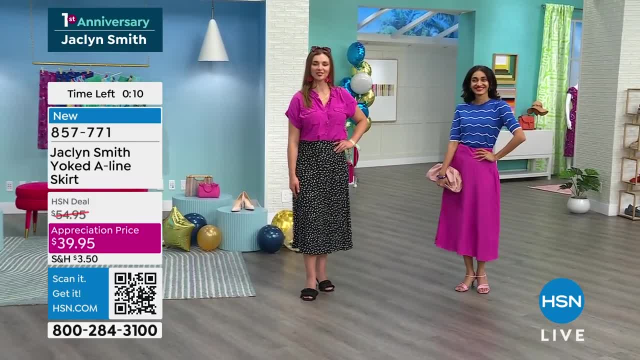 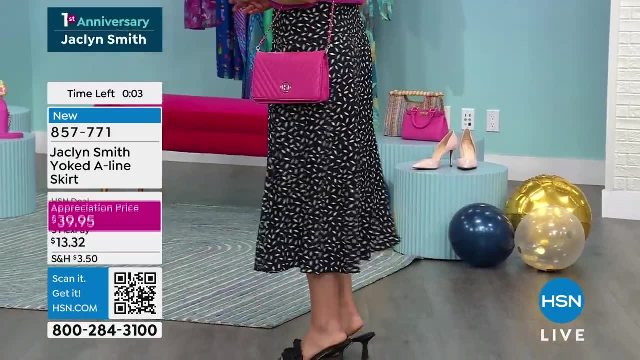 Don't you agree? You're looking at $34.. $39.95.. It's offered on FlexPay: $18.32.. Extra small through 3X And, of course, your opportunity to be able to shop. Hey, don't forget about the great savings that we're offering with the coupon. 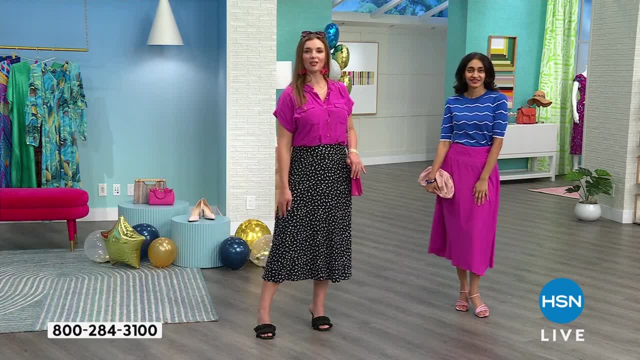 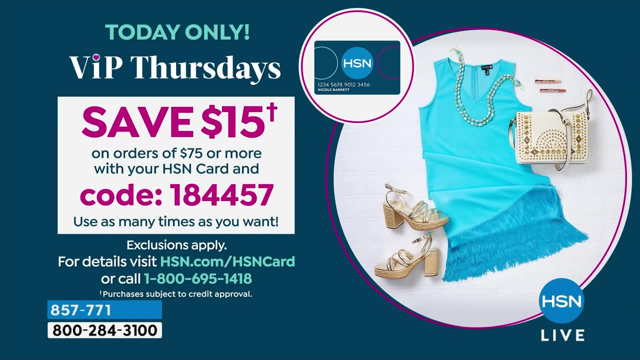 $15 off of your purchase of $75 or more When you use the HSN card And there's your code: It's 1-844-457.. And be sure to check out Every time that you get to that $75 threshold. check out and then start over. 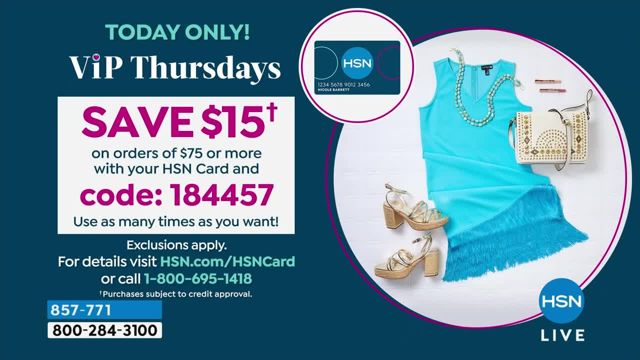 Again, because you can actually use that coupon as many times as you'd like today, Excellent. So you know, if you're like I'm learning a lot, Yeah, You want to, you know, kind of really get into it. 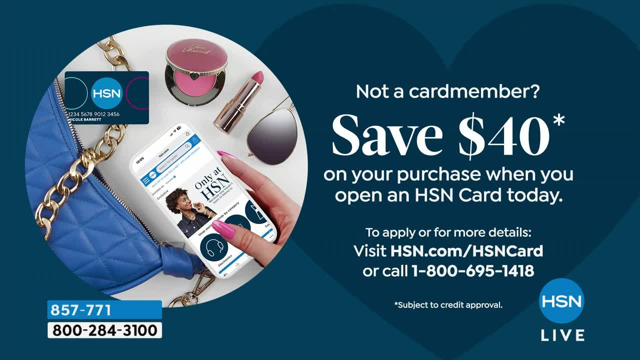 You can. You can use it, as you know, an unlimited amount of time. Also, we are offering you one of the most generous savings when you do open an HSN card, Because some of you are saying, hey, I don't understand the whole coupon thing. 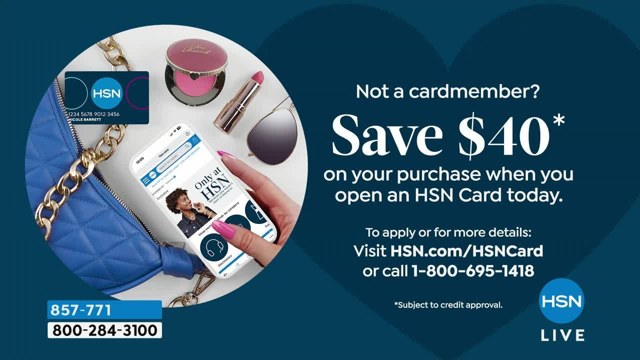 Well, the coupon is for those of you that have the HSN card. If you don't have the HSN card, Today is a magnificent day to apply for it, Because when you apply and approve, And most people that apply for the card will get approved. 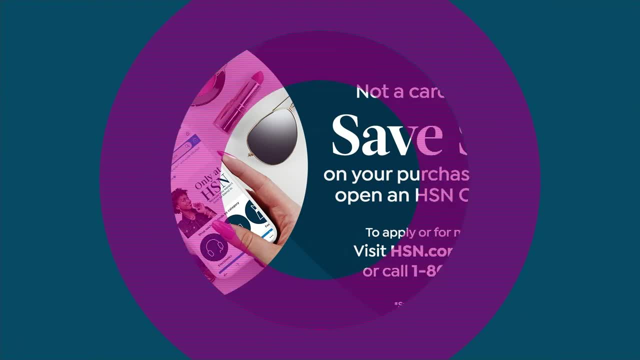 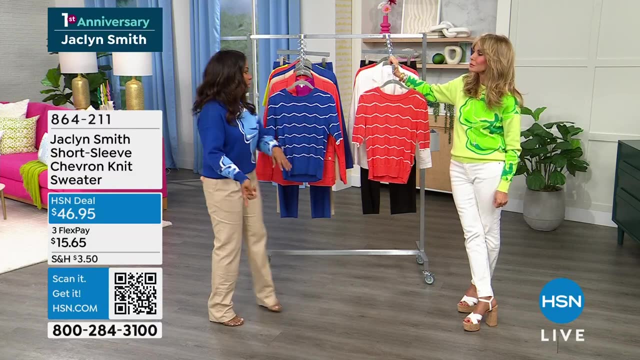 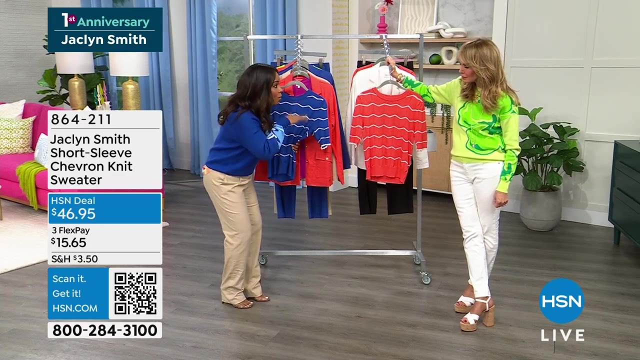 You will save $40 on your first purchase. So here's what that looks like. Amazing. You call or you go online. You apply, You instantly get approved. Now you save $40 off your first purchase- Interesting Right. But then you get to your $75 mark. 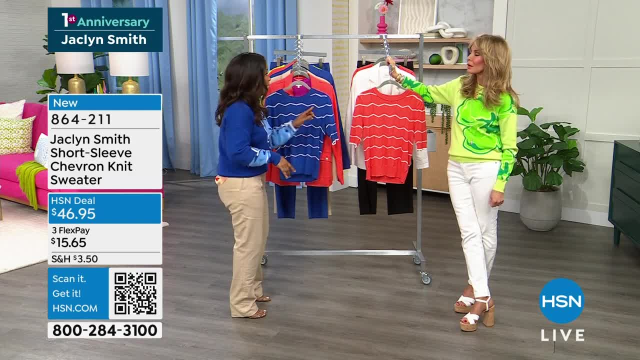 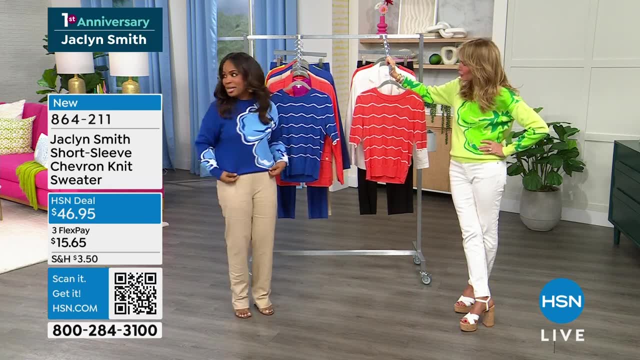 And then you check out Right, Then you go, And then you go back in. If you see something else, you can still use the coupon on the next purchase of the $15.. I know, So today's a great day to do some shopping. 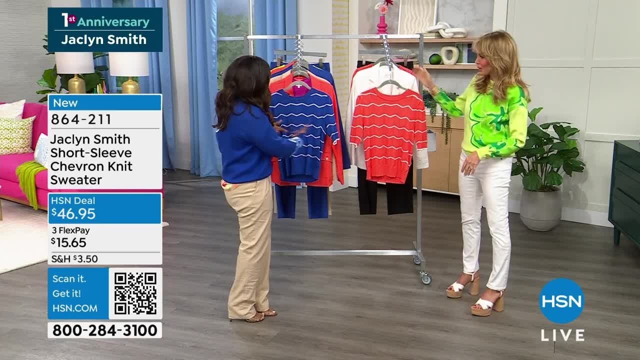 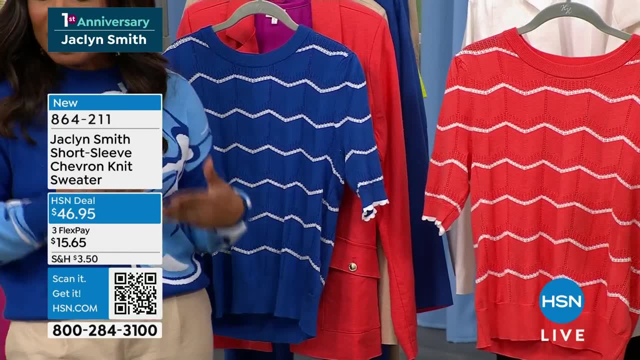 This is the day to shop. Today's the day. We would look so great in the sweater, So I think I'm actually going to take this one off and slip this one on. Oh, you're a mess. So here is our short sleeve chevron knit sweater. 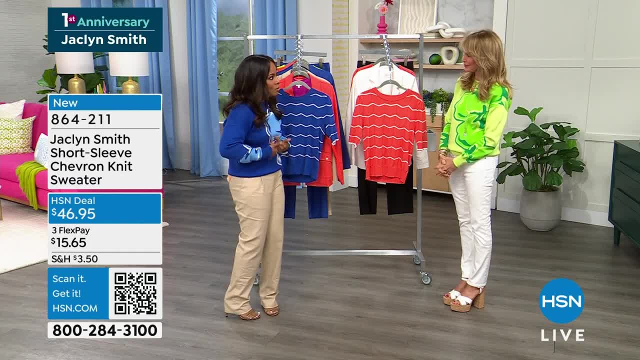 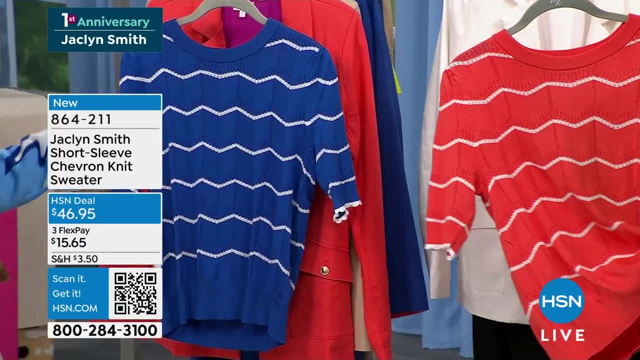 It's not the first time that you've seen this sweater, Because we've been giving you a little sneak peek of it underneath some of the blazers And with the skirt, And it's so much fun. It really is. This sweater looks like the French maritime feeling. 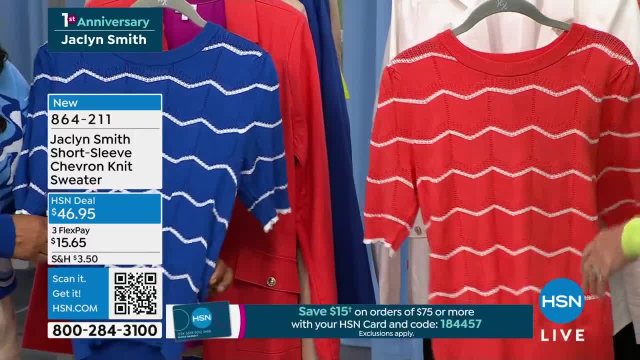 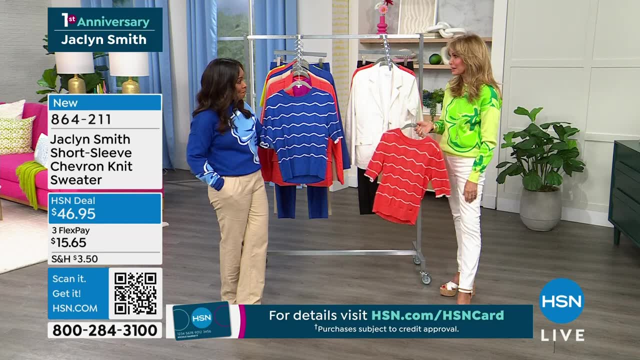 Yes, And it's part of French dressing. going way back, It was a sailor uniform And the chicest Parisian women wore this look. Think, go back to the 60s, Bonnie and Clyde. Yeah, She wore this with the A-line skirt throughout the movie. 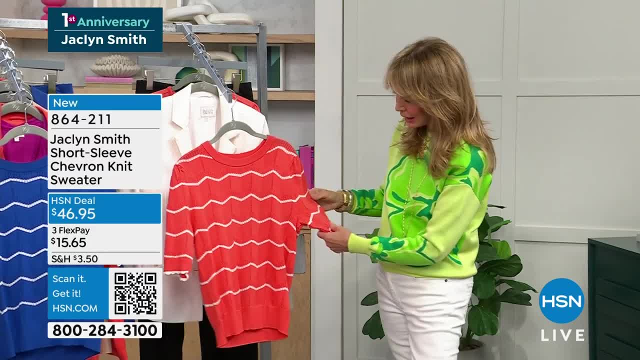 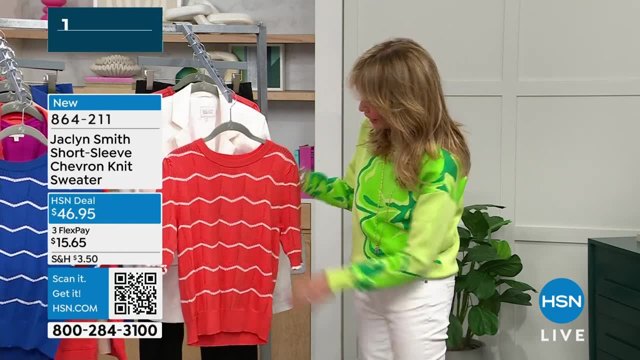 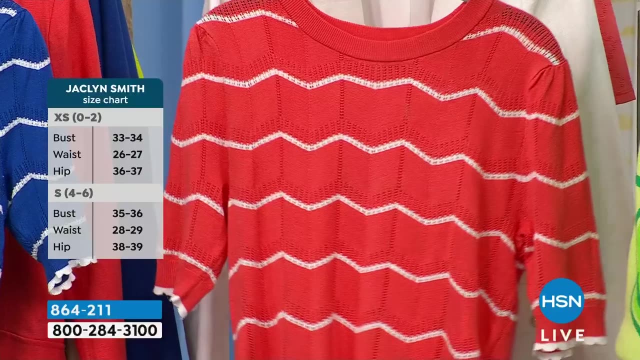 These are very classic, You know. it's a classic design that we sort of Updated with the chevron Pretty The wave that goes across the front in a zigzag. But there's one thing I really love about this particular sweater. 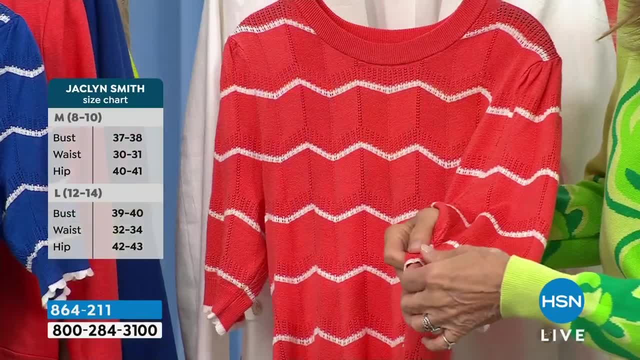 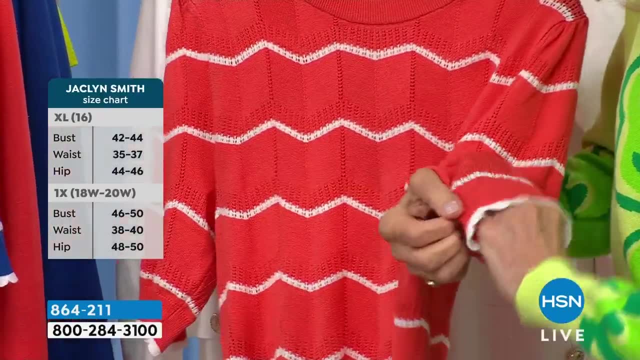 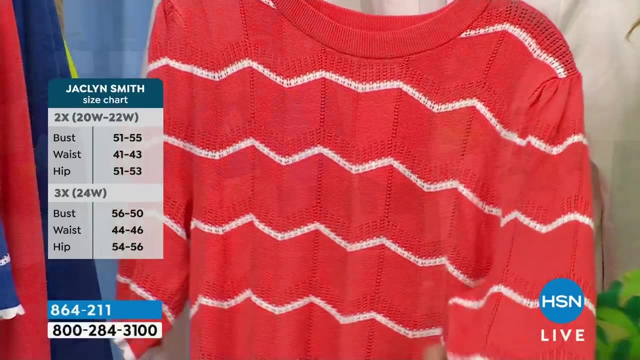 It's this beautiful scalloped edge Which is difficult to do. It's precise, to get it even, And when it's on your skin it is so feminine. That little scalloped edge, These little details, just sort of make the difference. 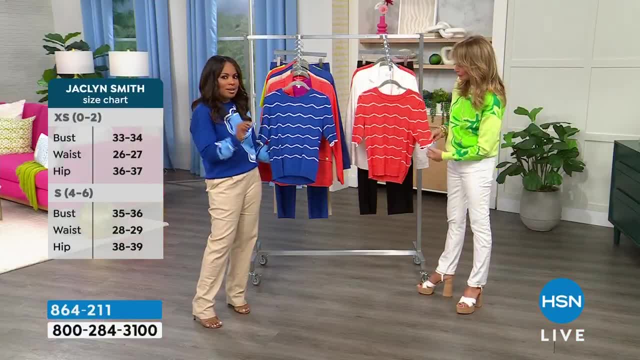 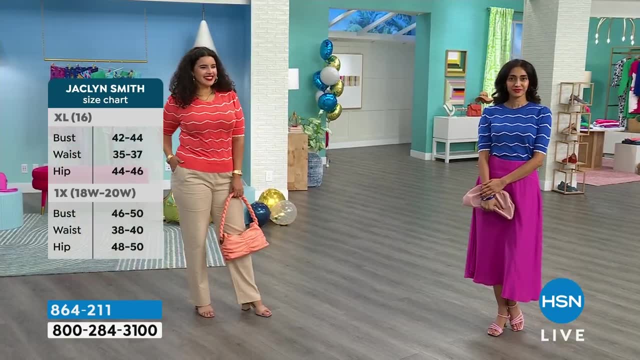 To me, That's one of the things that I think is so special about your collection- Is that you go the distance, You never leave any stone unturned, Giving you really the most beautiful quality And the fabric right Soft to your skin. 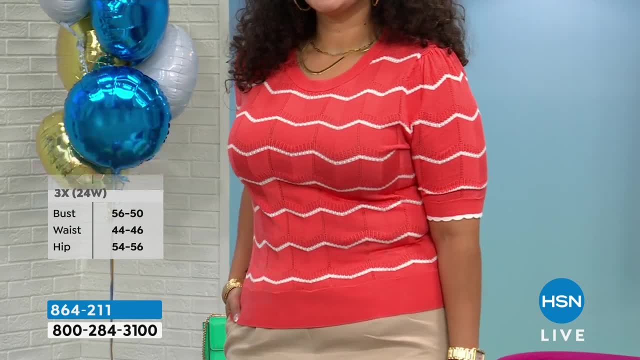 Look at the beautiful fit. Feels great on It, has bounce recovery. Yes, It's not going to stretch out. Oh my gosh, It's just so pretty. It's machine washable. So ember glow is going to be the orange. 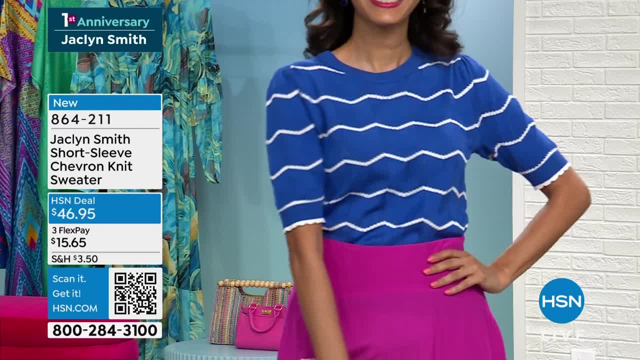 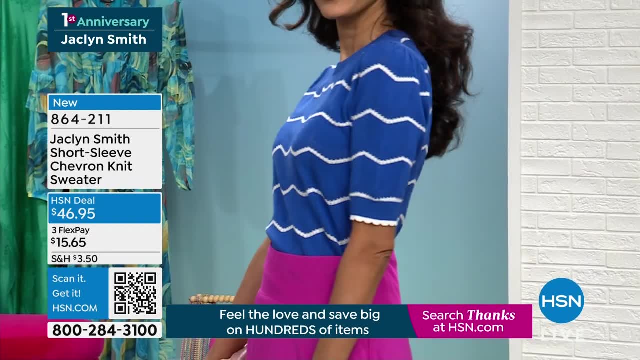 And then the blue. we're just calling our Our blue. It's 23 inches in the length. Whether or not you're tucking this one in Or you're wearing it on the outside- Extra small, through 3X, Also super popular. 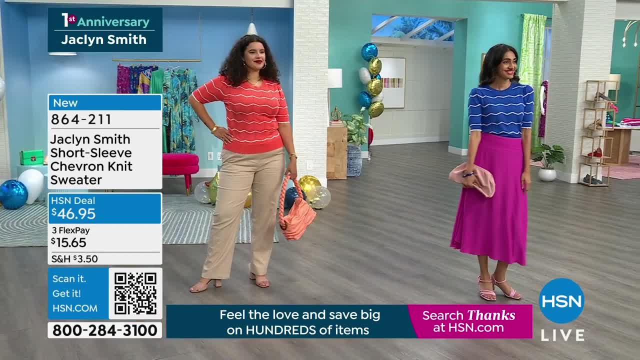 I am not surprised. I think this one, Such a great love, Tucked in worn out. I'm actually going to take that orange from you. You want the orange? Yeah, Okay, I am going to take that one. You're magic with these. 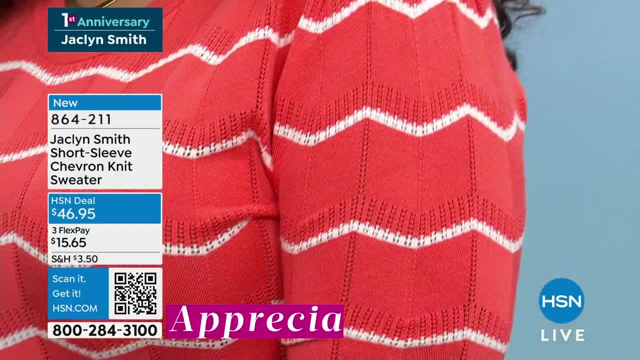 I love the way you do this With such ease. I don't really know, I probably don't look the best doing it. Oh, yes, you do, We're all friends. I am like I am really impressed, We're all friends. 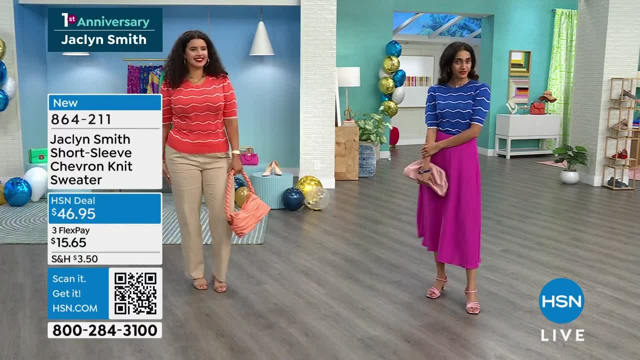 That's the back. Okay, That's the back. Yeah, All right, Perfect, Thank you. Yeah, I figure You know I'll be twins with the Well, even with your floral underneath it. That's what I was thinking. 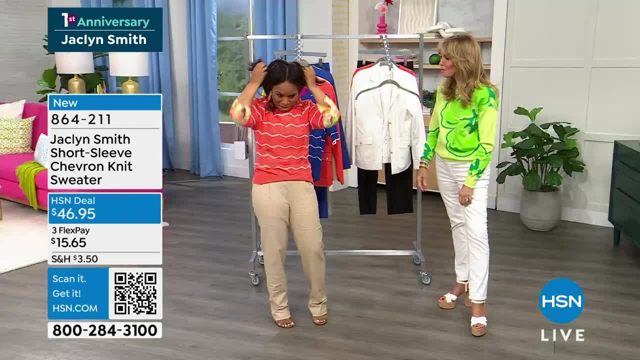 You know You're a master of the game. You are a master of the game. It looks great with the floral coming out. What do you guys think I think you could? You could definitely get away with it. You can even do your collar. 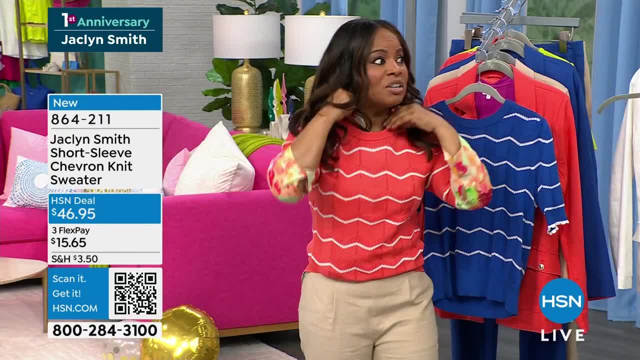 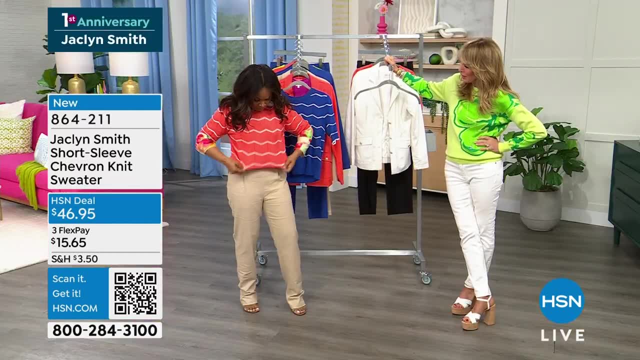 Yeah, I like, Oh great. I like the combination of the stripes and the florals. I think we need to add you to the team. It's fun to do that. Yeah, It really is. Look at how cute It looks great. 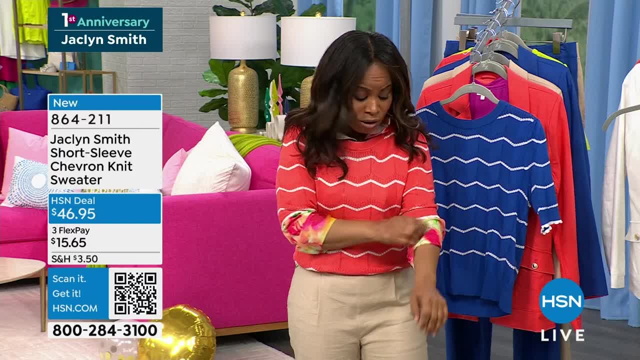 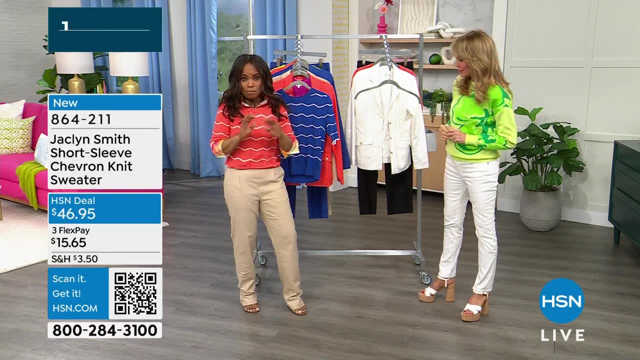 That's cute, I mean, it looks amazing. I'm telling You're, I'm telling Listen, I have been saying it- So versatile And going a million different ways, This collection, First anniversary. You're just discovering the Jacqueline Smith collection. 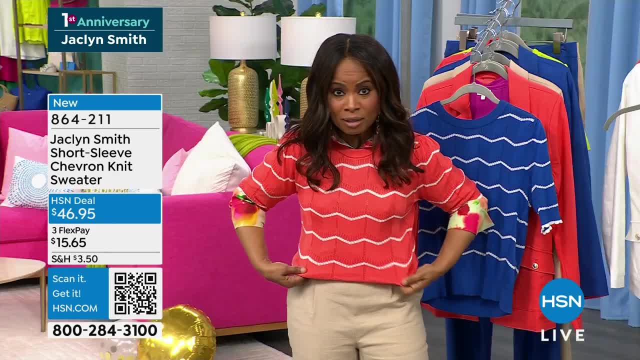 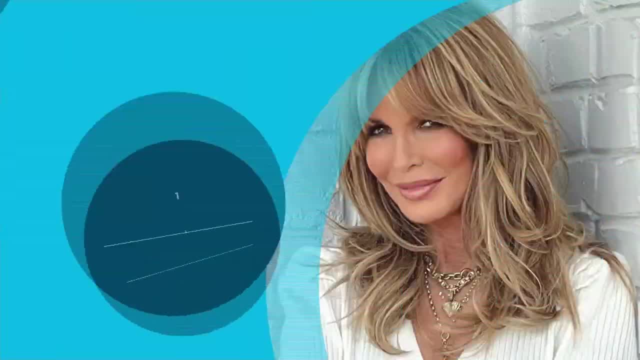 I'm telling you, Best kept one year secret ever. I hope that you'll go on to our website at HSNcom. I mean, look at how great that is. It is You look great? Yeah, It's such a great piece. 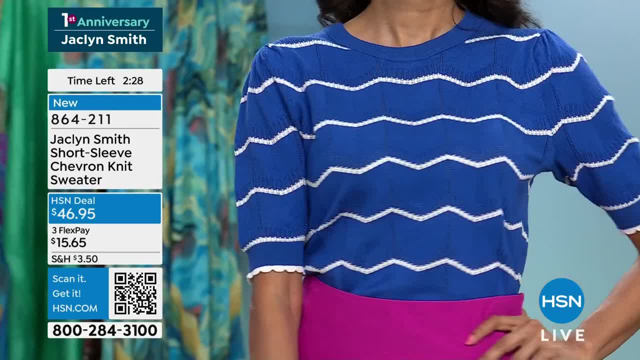 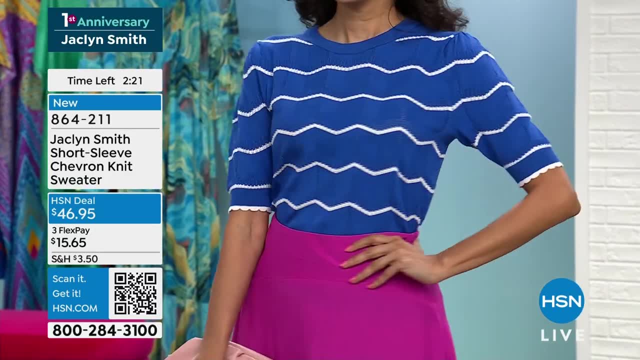 Feels good on. It won't stretch out. It has rebound The neckline After washing. It's great, Nice, rounded neckline. You don't have to wear undergarment underneath it. I'd like that every what you do with the sleeves. 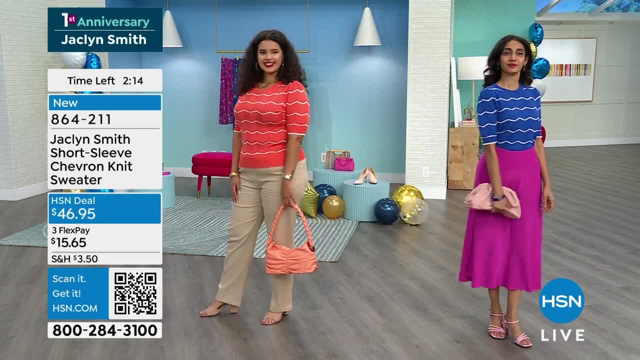 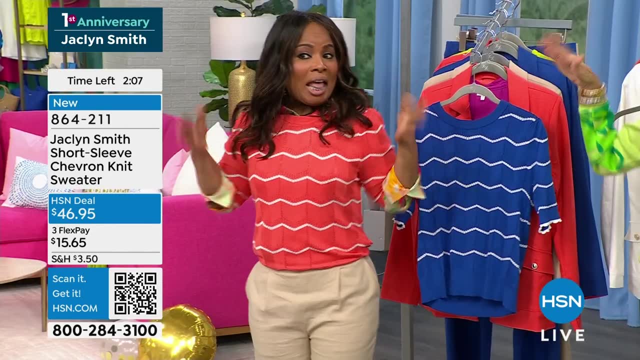 I don't know how well we can see the sleeves. Well, the little scallop And the little, And at the very top It has a little puff, Yes, Which I like that, because any time you have just a little bit It's slenderized. 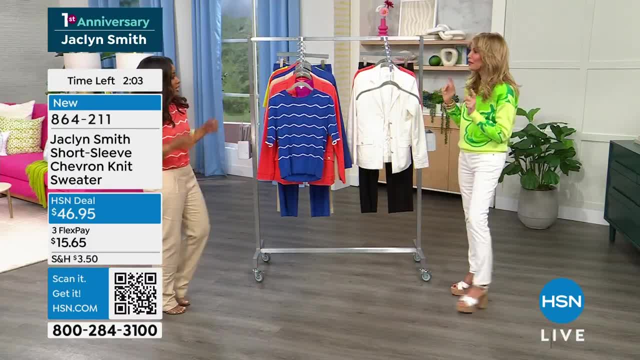 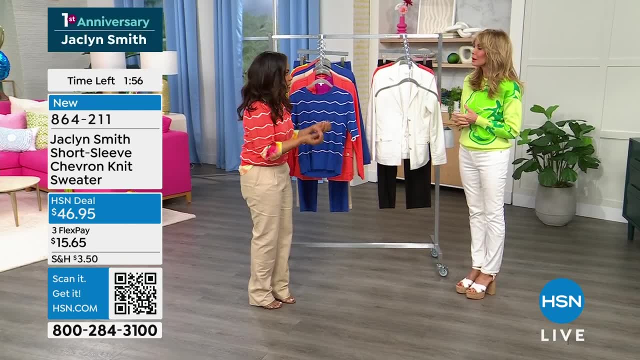 Yeah, The torso. Yeah, A little bit Shoulder show and waist. Yes, We need that, We need that. That's where shoulder pads come in. Yeah, You know And, but you could have easily. I will tell you 99.9% of the garments that we see. 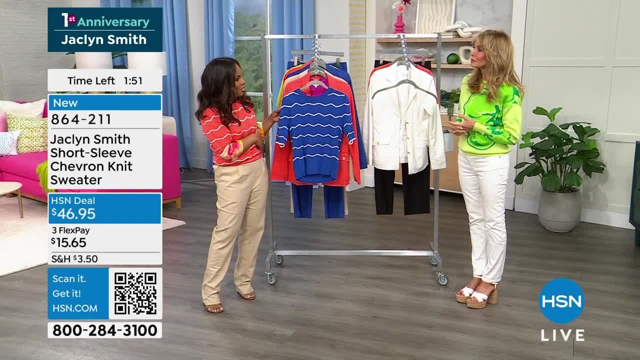 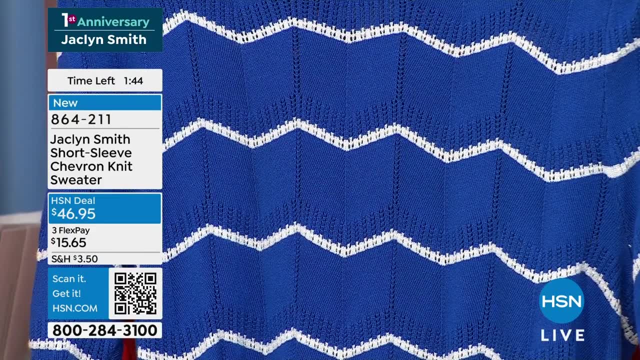 Like you know, most people just overlook that detail, Right, And it's, And it's an important one. It's important to be able to have those. Those are those little hidden secrets that we want, as women, to trick the eye a little bit. 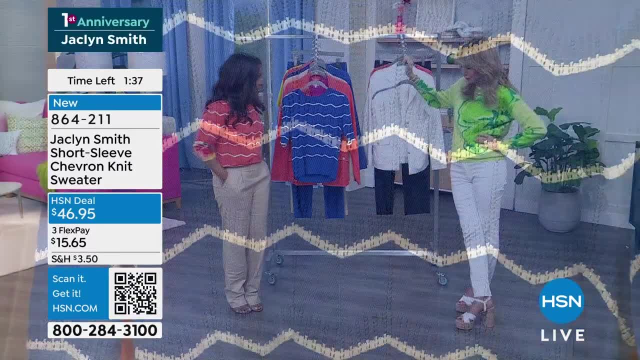 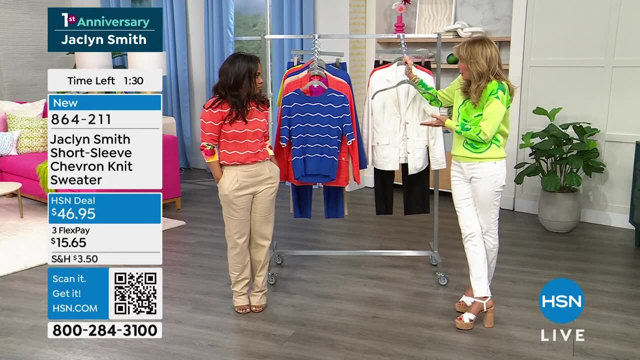 Trick the eye, You know, And have a sort of built in hidden illusion. Yes, it makes us look really pretty. right, when we put the garments on, we feel, when we feel like we, we are pretty. yes, yes, what's inside that comes out. light attracts light. yes, and how. how great both. 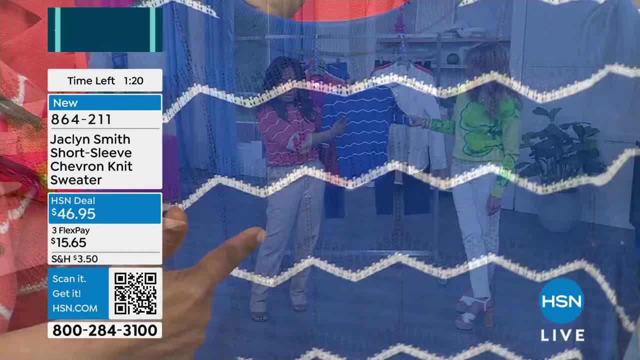 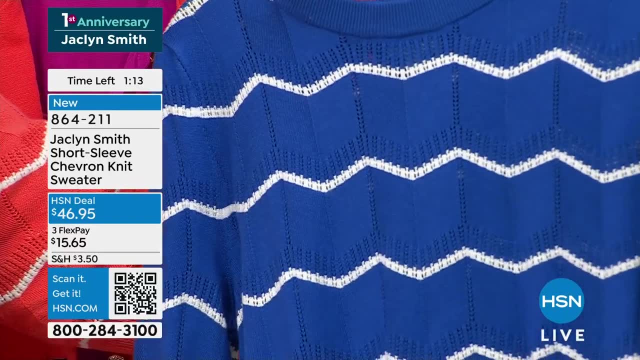 of these pieces. um, have that zigzag line with the white right, and so we talk. it is a point, point tail stitch in this in the chevron, and the weight is really beautiful. so you'll just let us know which one is your favorite. i'm curious, rocky, which one is more more popular? is it the blue? 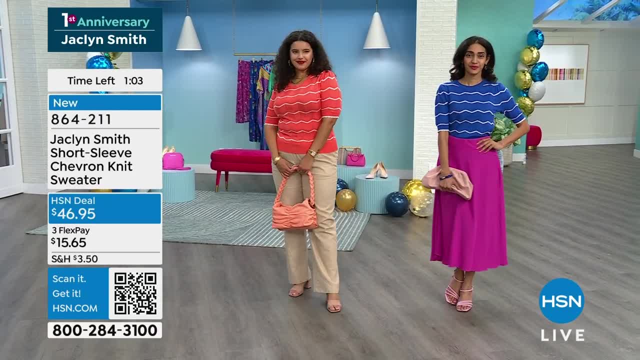 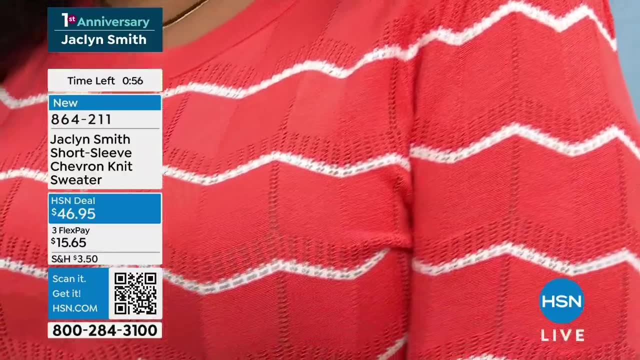 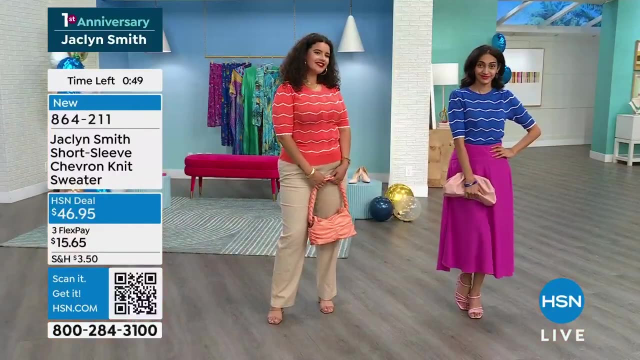 is it the ember glow, the orange? okay, so you're selling it kind of neck and neck. the ember glow is just a little bit more popular, but they're both. they're both, i think, a great choice. um, and i would do the ember glow back with the ember glow jacket, if you want the tone on tone. 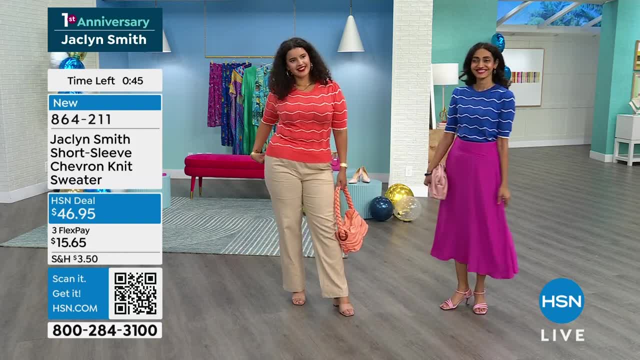 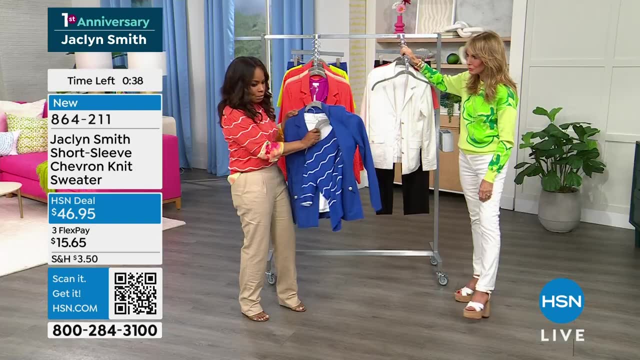 or you can go. really, you can do it with any of them honestly. yeah, yeah, yeah, so we do have coming up. we have our um blazer that will be coming up. so if you like more of a tonal look, you could go. that looks great, you can go. 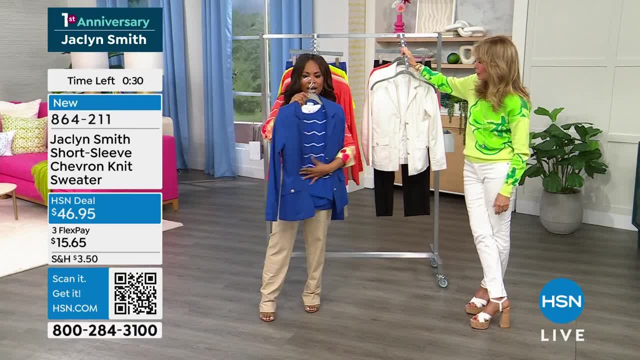 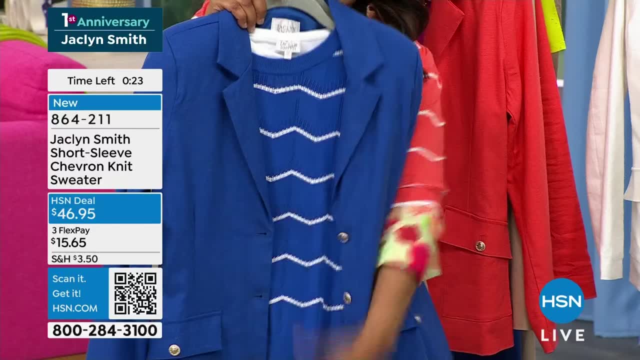 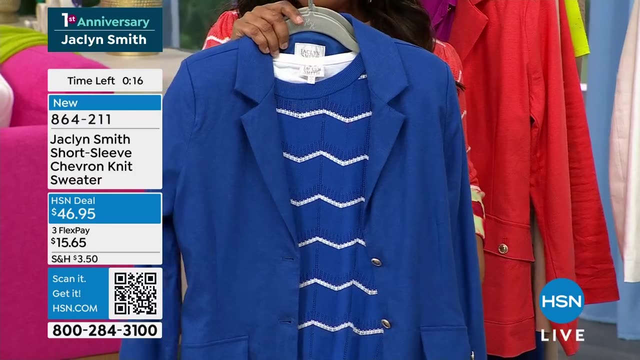 more. i mean so many things go with this blazer and i like the idea of breaking this up with a white jean. instead of doing the tonal, yeah, the all blue, i like the white jean just to kind of break the look. great really, i know, with a white jean i mean so absolutely, so easy everything. 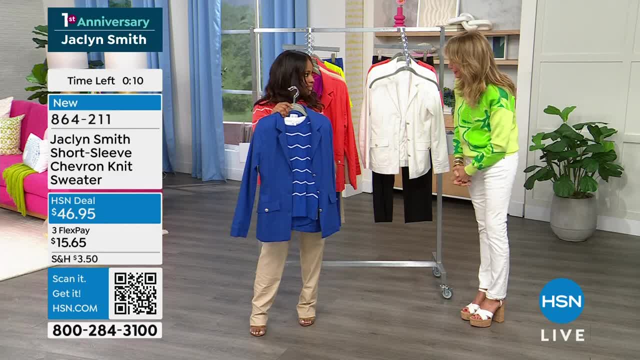 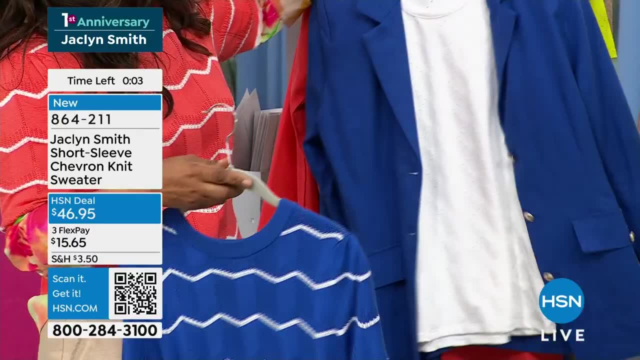 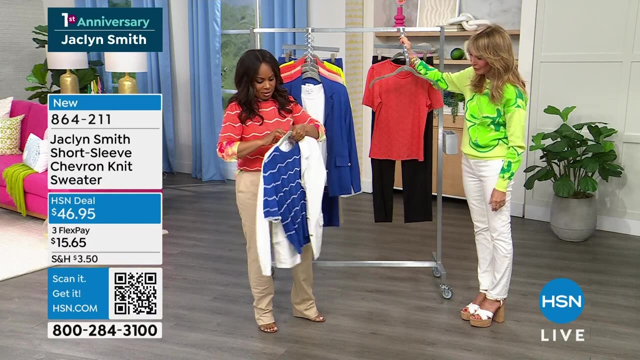 goes back to this linen jacket. the linen jacket is really the key that pulls everything together. tone on tone are shaking it up and doing the fuchsia. and if you're not afraid of white, i'm never afraid of the white. i just think it's gorgeous. yeah, look at. i mean because 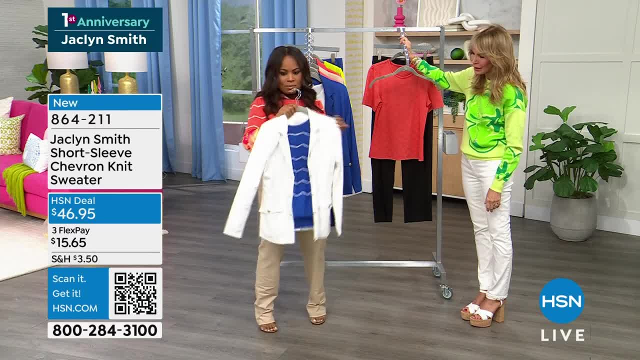 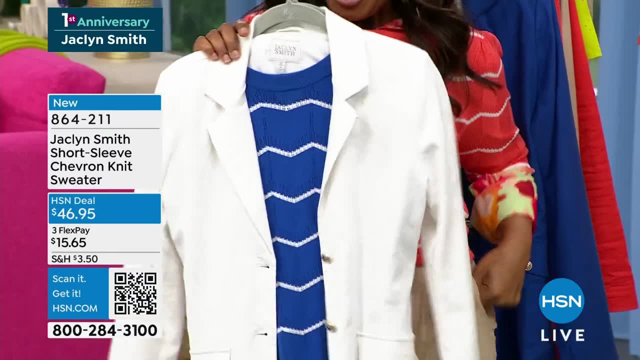 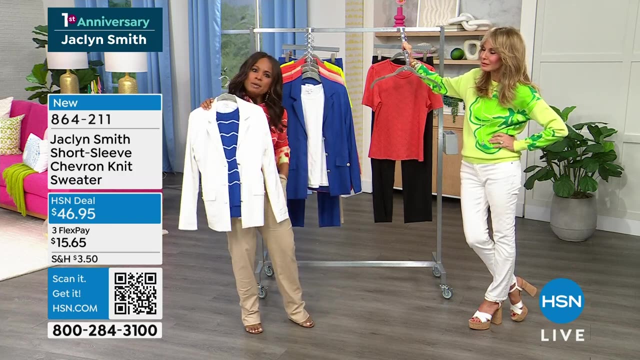 it has the white stripes. it looks amazing. so clean and summery. that is beautiful. you're gonna look so pretty. i think you'll join the team. you're gonna look so pretty. look at how great you're gonna look with that on phenomenal. wherever you may go, you know you're gonna meet your girls. 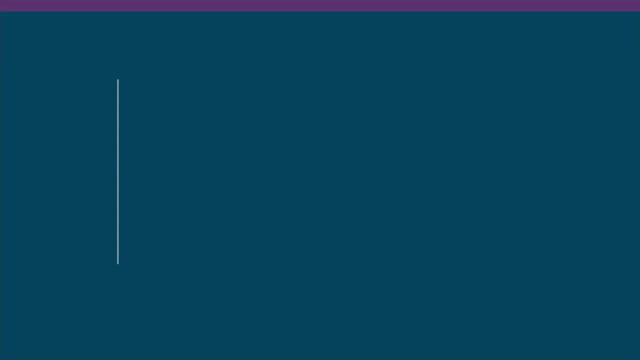 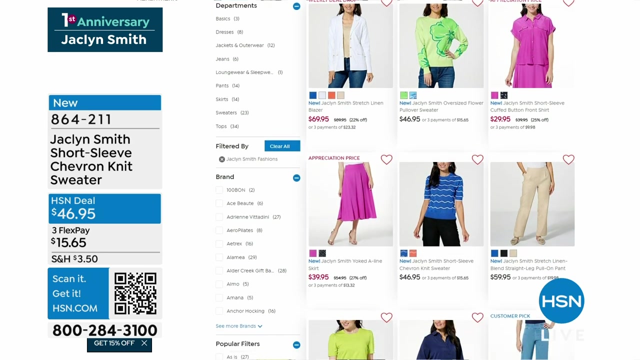 your friends that you haven't seen for a while. for lunch: yes, you look terrific. you'll have a dinner in the evening morning. it's like an effortless, chic look, um, that we all want. like you didn't try so hard, um, but you look amazing. hey, shop more of jacqueline smith's collection. 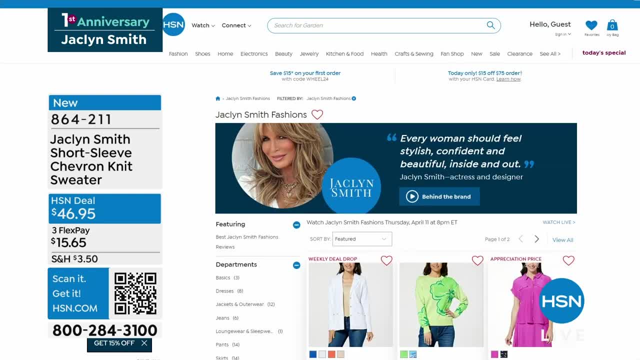 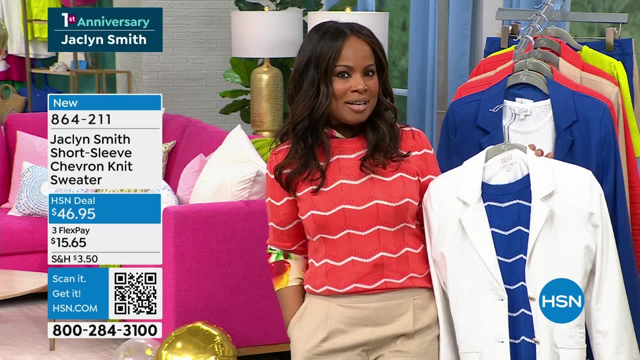 on our website at hsncom. all the pieces are there for you 24 hours a day, seven days a week, while they last. that's the trick. um, they're always in short supply when we come back. we're actually going to give you a little bit of a look at what we're going to show you in a little bit. 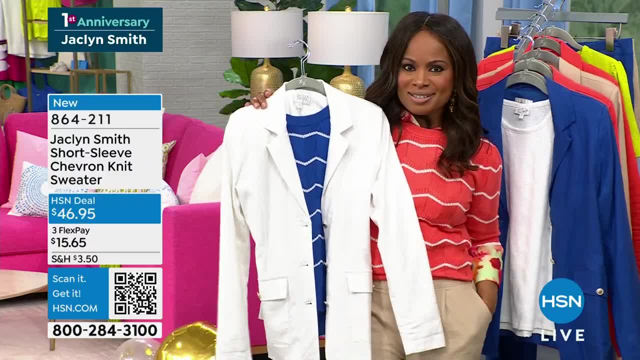 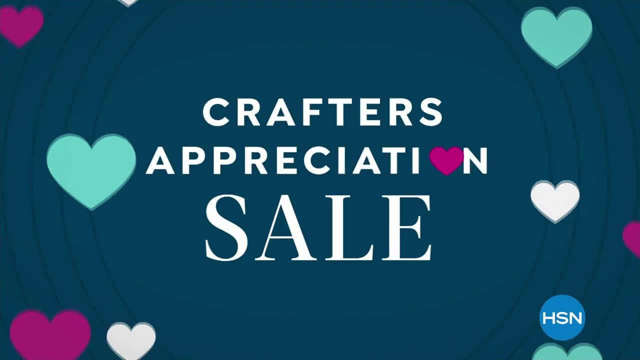 we're going to give you a look at the blazer, which is our weekly deal drop right after this. attentional crafters, get ready for an exclusive 24-hour event just for you. it's hsn's crafters appreciation sale- from scrapbooking to paper crafting and even home decor, and it's all on sale. 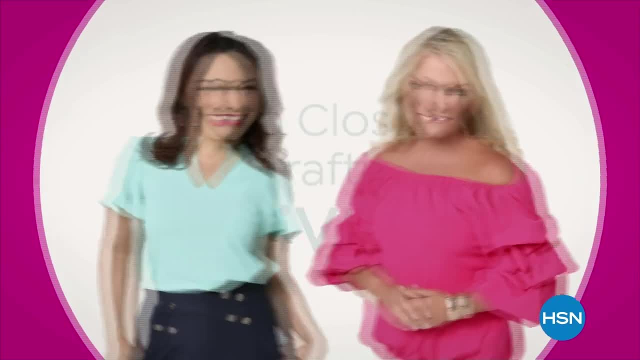 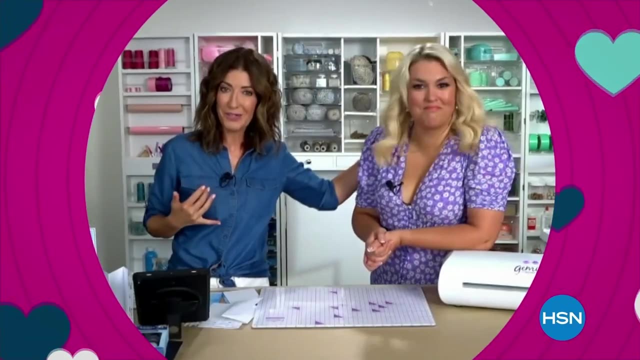 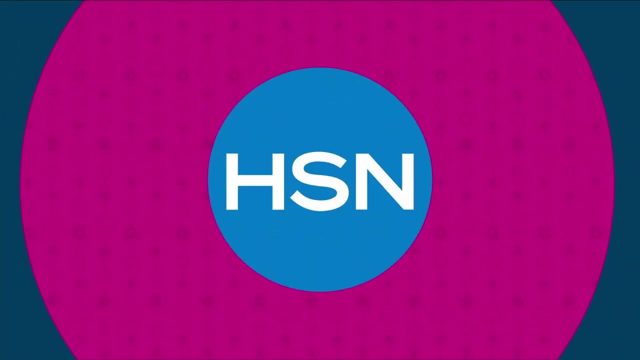 plus, join hsn's craftinistas tina and suzanne for the premiere of up close and crafting. live our first ever hands-on crafting event with your favorite crafting experts and lovers like you: 24-hour crafting extravaganza only on hsn. the hsn deal is a great value that we bring to you. 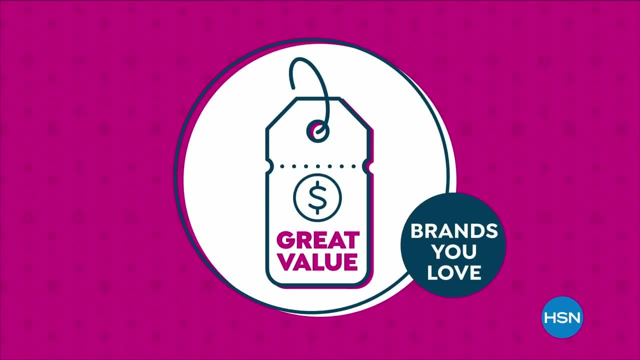 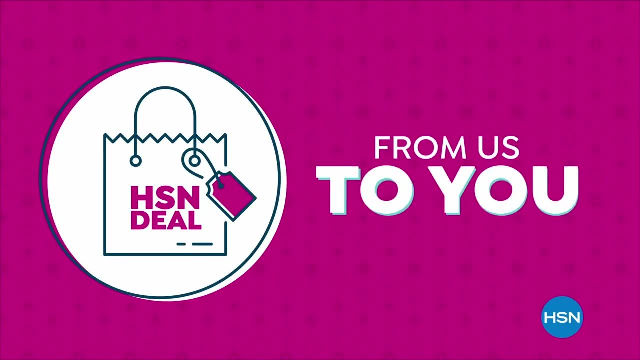 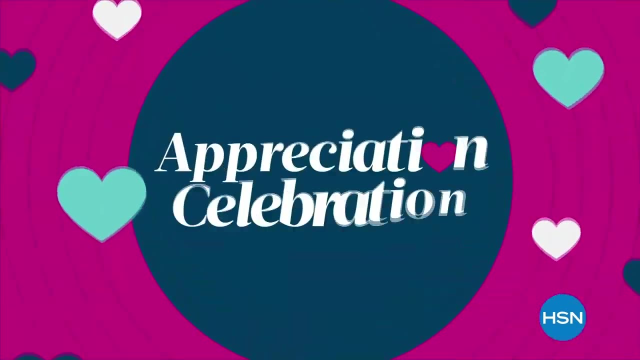 every day. thanks to our long and valued partnerships with the brands you love most, we are able to offer amazing products at great values. shop the hsn deal with confidence from us to you. we're throwing a special weekend long party to honor all you mean to us. join us for our 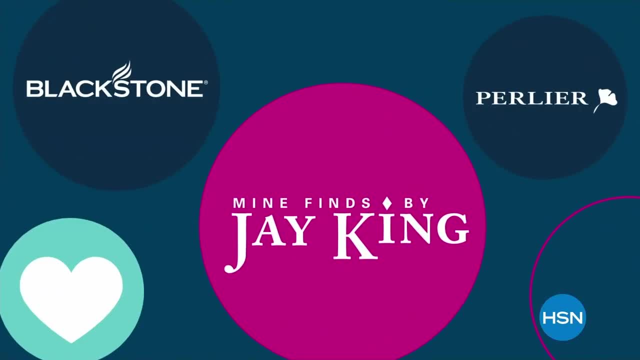 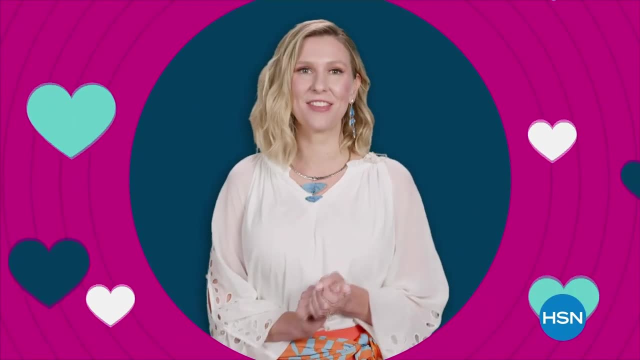 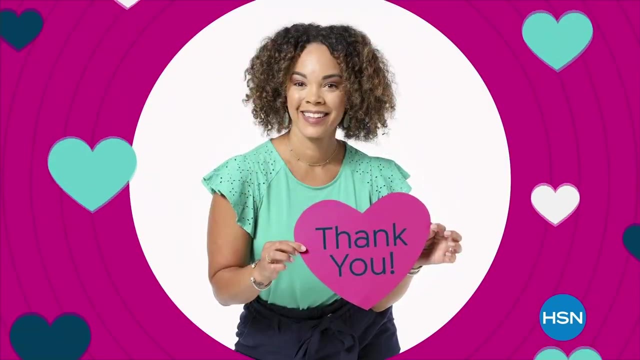 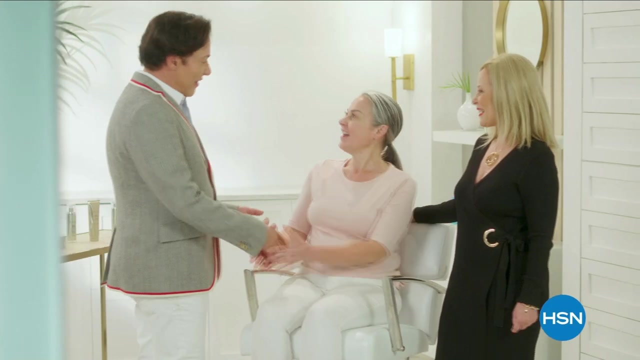 appreciation celebration complete with your favorite brands, products and hosts. enjoy special deals and appreciation pricing. we love our hsn family and that includes you. happy customer appreciation month. we're grateful because every day at hsn you are at the heart of everything we do. saturday at midnight. we understand every woman's skin is unique. we offer 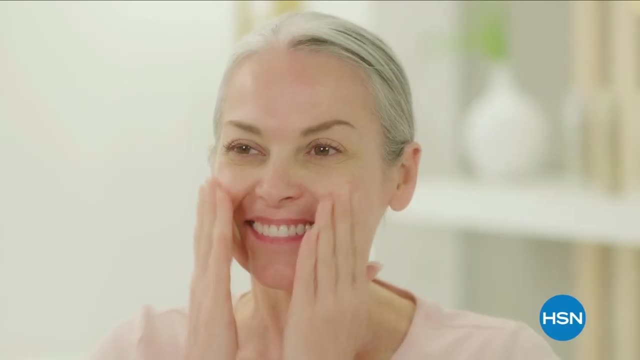 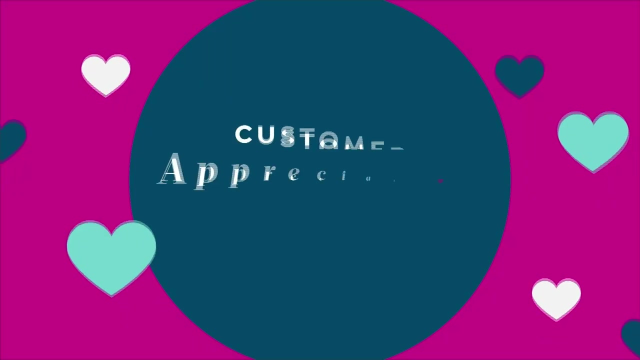 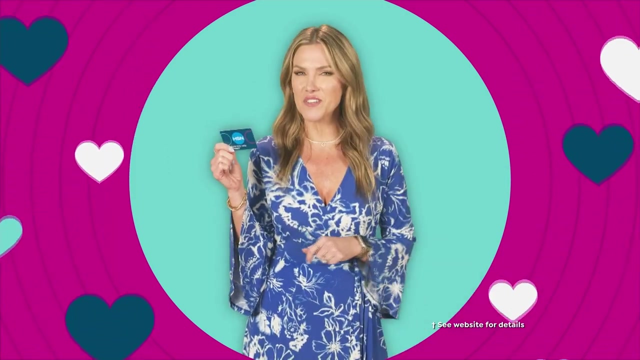 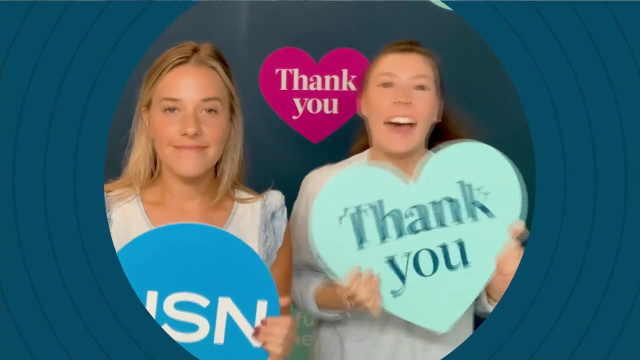 real beauty solutions, empowering women to achieve healthy, radiant looking skin. genuine beauty begins with skin. get rolling like a vip with your hsn card. today it's vip thursday and for even more surprise savings, you'll love join us tomorrow for flash friday. hi, thank you so much for being a part of our family. we love that you're a black belt shopper. 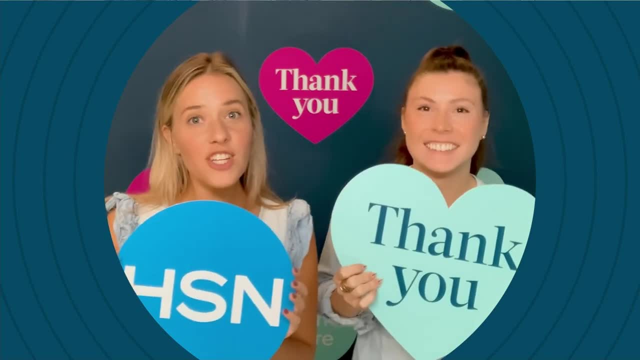 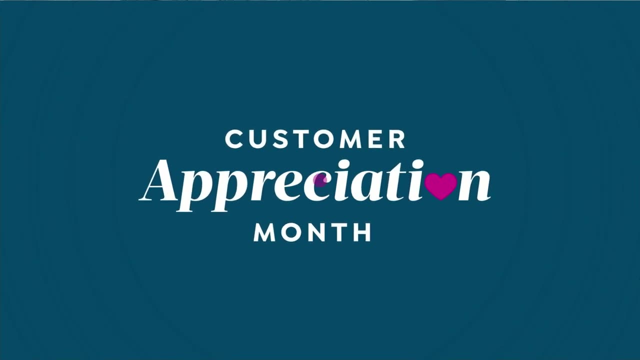 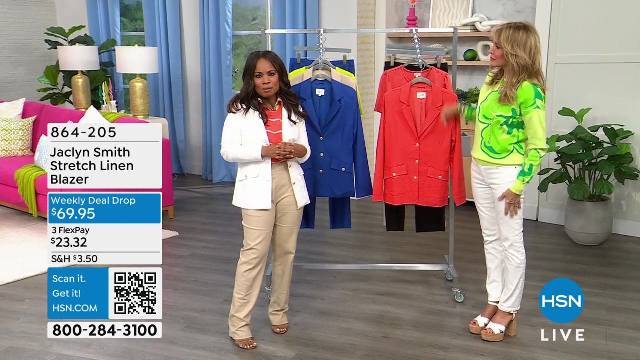 and you find exclusive products only at hsn. we appreciate you. we also love how trendy you are. how much fun is that? so we are celebrating you this month. all month long we are celebrating customer appreciation month and we can't say thank you enough for being an hsn customer. how 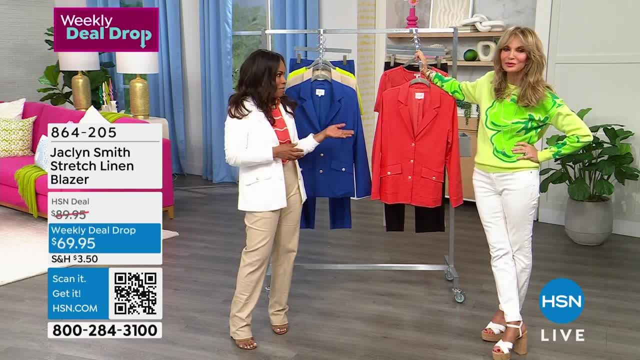 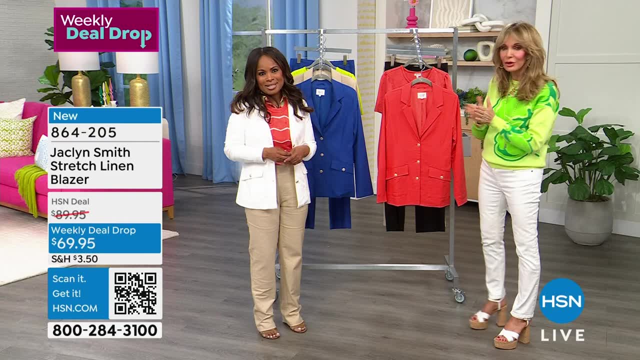 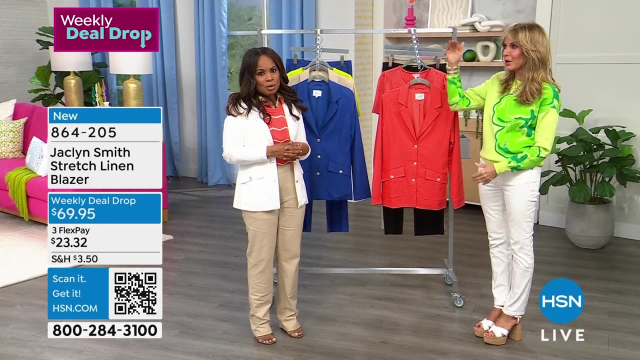 lucky are we to have you as a customer and i've me being a long time host here. uh, it's just with such gratitude that, yes, feedback is so great. yes, always hear your thoughts and what you love. that really helped me. yeah, you sure, open us right. you make us better, make us better, yeah, which we so appreciate. which we appreciate. 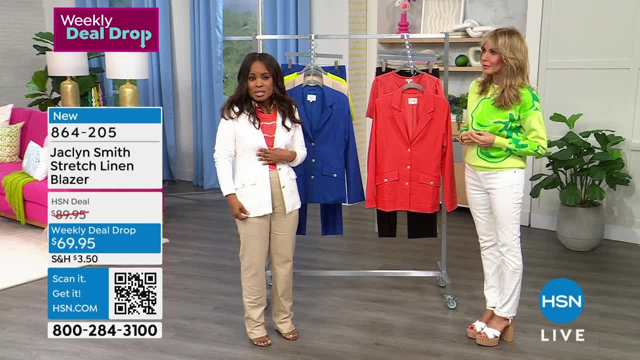 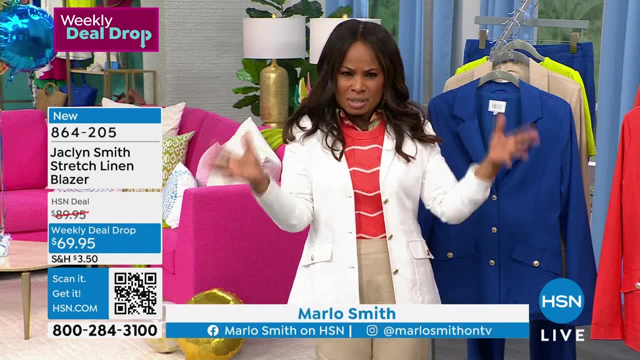 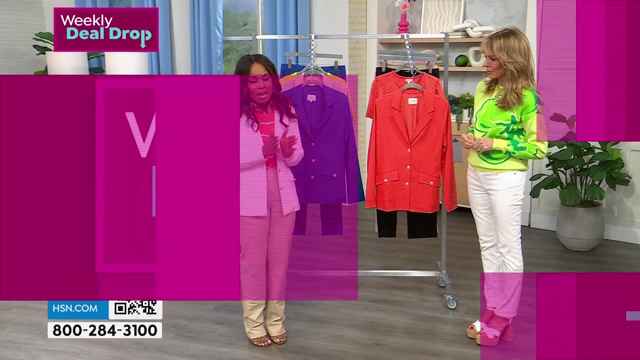 well, as promised, we're going to be talking about the blazer now. the blazer is what we call a weekly deal drop. so every monday we launch several weekly deal drops across different categories. this one, you have to admit, is rather beautiful. it's been very popular. we do offer it to you an extra small. 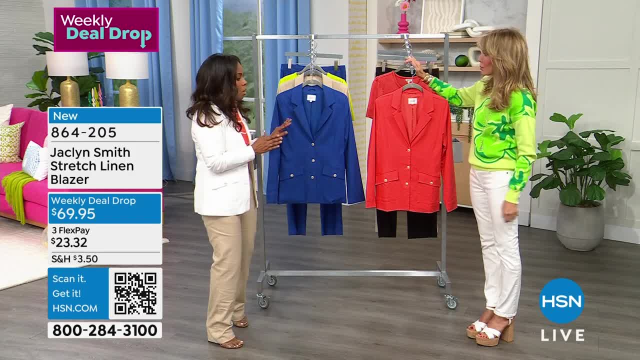 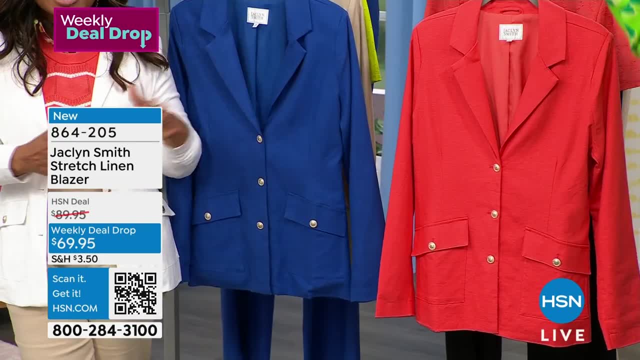 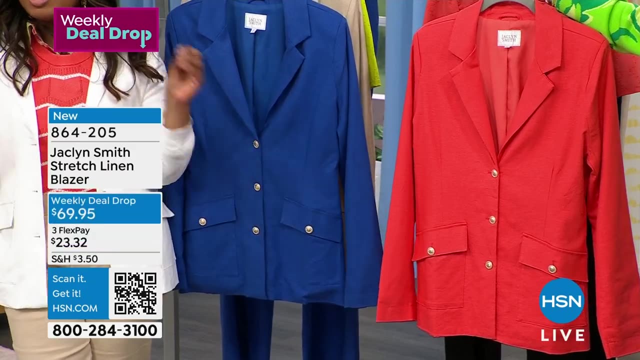 through 3x. i will say in most of the colors we've sold out of the extra small size. i know in the ember glow, in the blue as as well. okay, in all four choices the extra small is sold out across the board. wonderful, however, i have bumped it. i wore the extra small. i have it on. 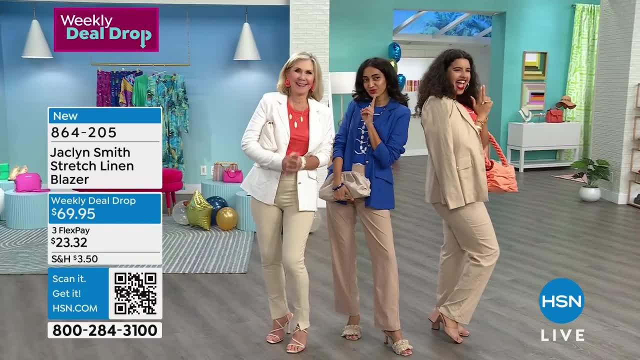 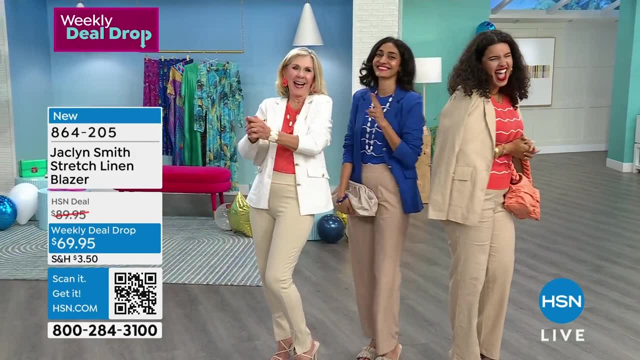 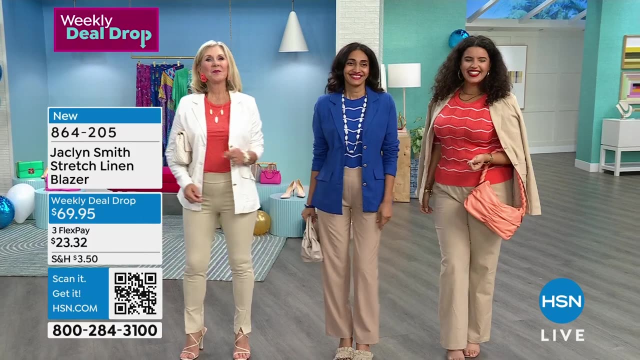 in the small. they're having so much fun. i have it on in the small and if you're my friends, i know we're all inspired by having you, jacklyn, here. yeah, i love it. so let's talk about this incredible blazer, this right it. you know it's a stretch linen, which i love- stretch linen lining. yes, so it wears really. 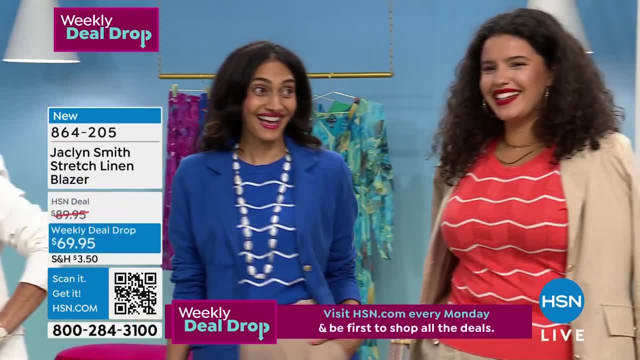 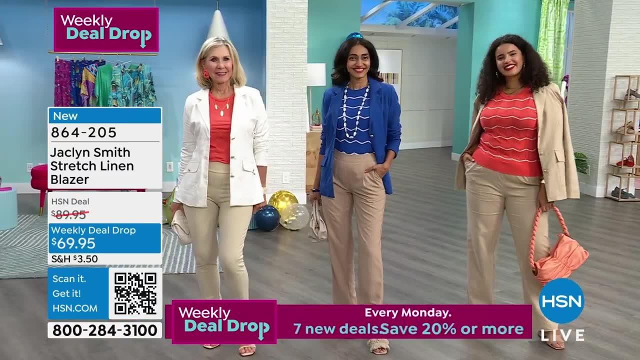 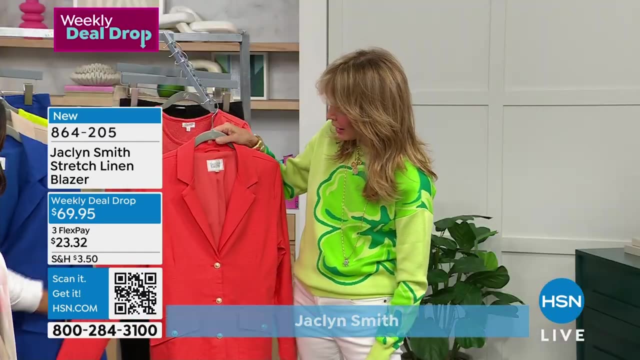 well, it moves with you. it moves with the angels over there. as you can see, they're moving around. nothing is out of place. uh, you know, i love it's a three button blazer. blazers are here to stay. they're never going to go out of style. and we have the little smart darts. 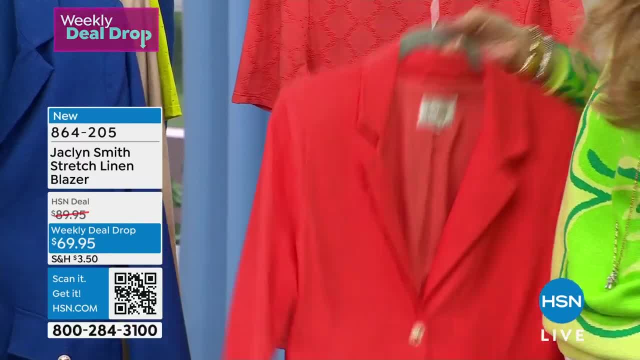 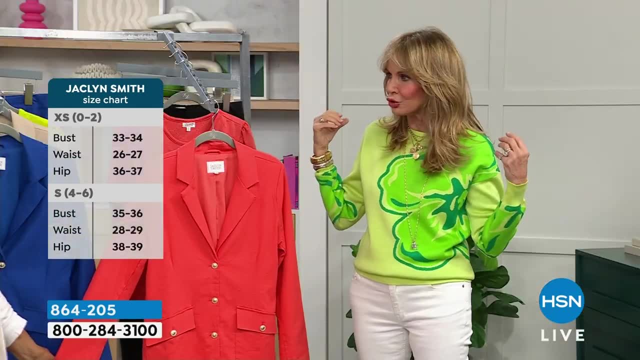 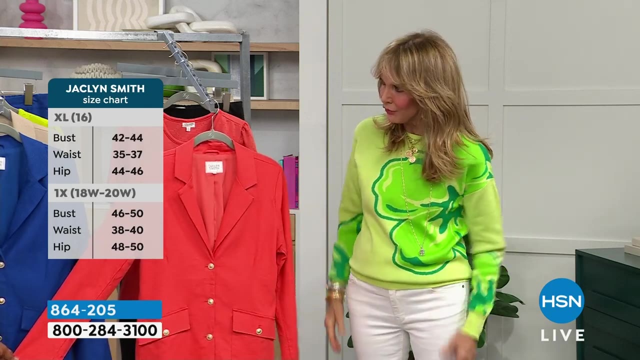 which give you a nicer silhouette: not fitted, but slimming, slimming. we didn't overfit this. it's not like in dynasty, where they had the broad shoulders and the nipped in waist, it's. it's an easy fit, but not a structured fit and it's so perfect. you know, when we presented this last hour, we talked 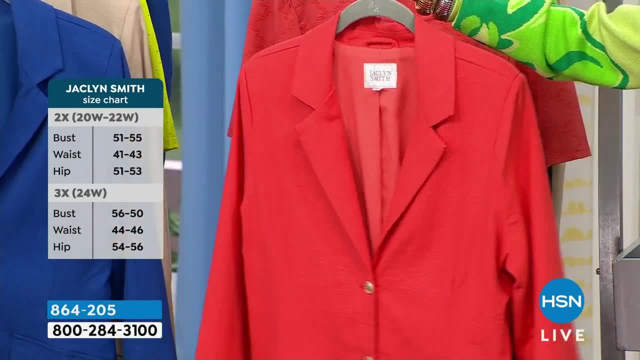 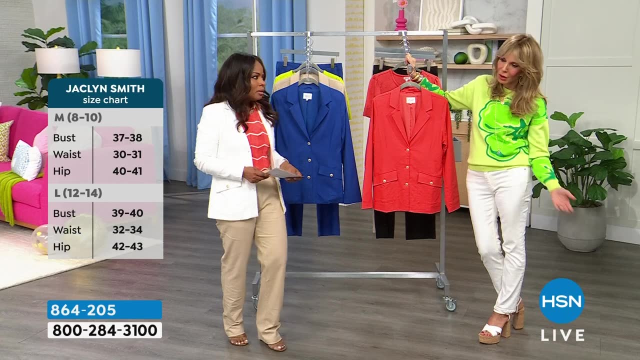 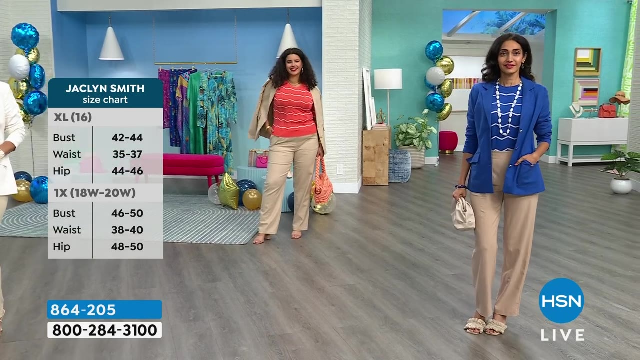 about how, because of the way that it's cut and the styling and that that stretch linen, it takes you every place right, you know whether you remember, to a party, to church, to a business meeting, you know an evening out where the temperature, you know, may get a little cool in the evening, it's just a great piece. the the price. 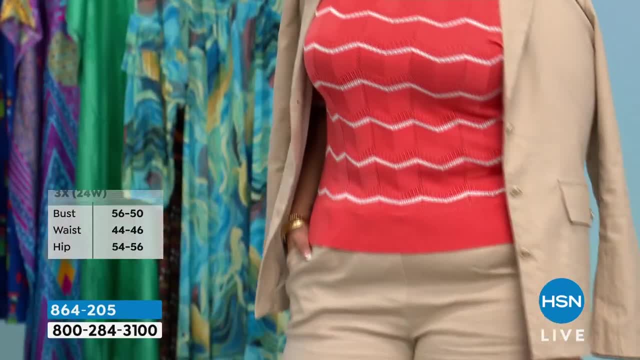 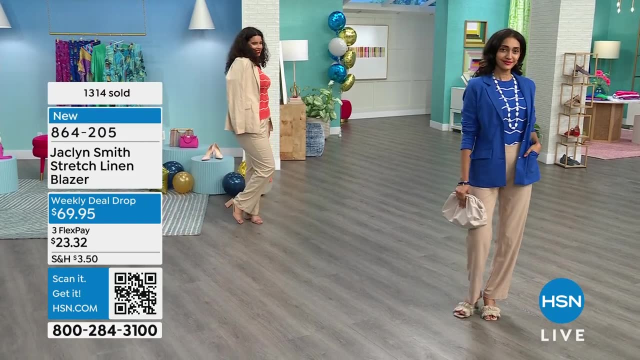 on. this is $69.95. we are sharing this with you on flex pay. that means you can certainly spread the payments out over three months. lengthwise. you're looking at 27 inches and the length over 1300 have been sold. i would not wait on this piece. we know that the extra smalls have sold out. if you needed. 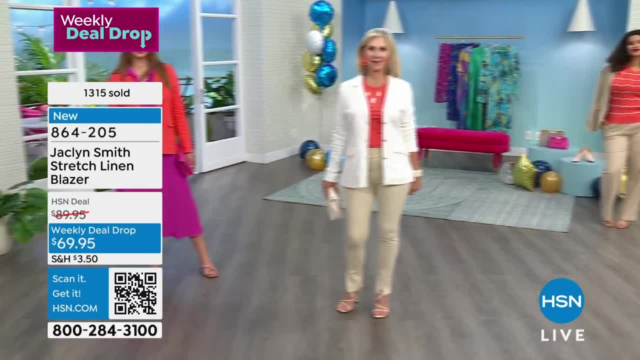 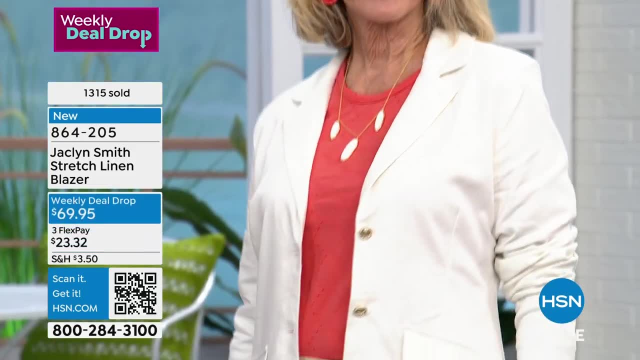 it as long as you have a blazer, if you do need it. it's just a little extra small. you know it's a little extra small. i definitely wouldn't. i would definitely. i would definitely go up to a small i had on because, yes, there i think you can wear with a blazer. you can go up a little oversized for sure. okay, yes, it's. 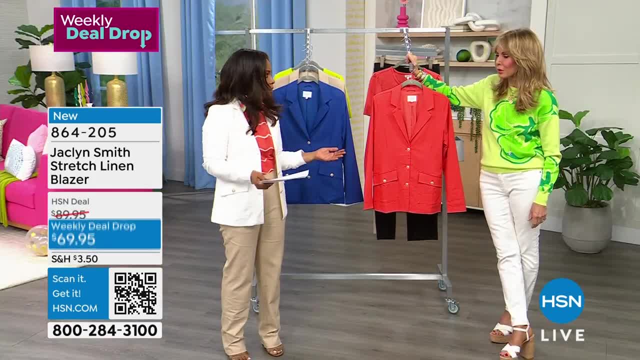 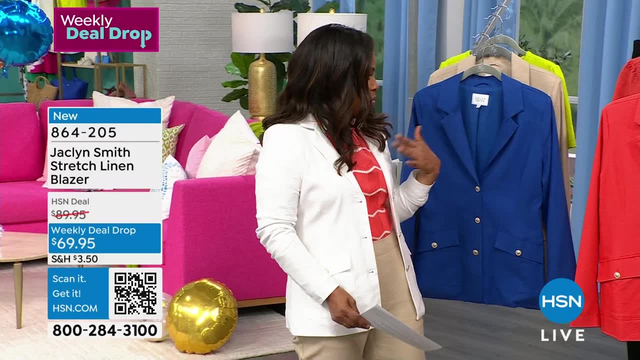 actually the kind of cool look that is a. i think this is a small nail and it fits my earlier- yeah, i was an extra small and that looks great. this fits great right for me. right, you know, because earlier i was in the extra small white. i don't know if we covered the colors white, blue, ember glow and then we also have it available for the rest of the day. 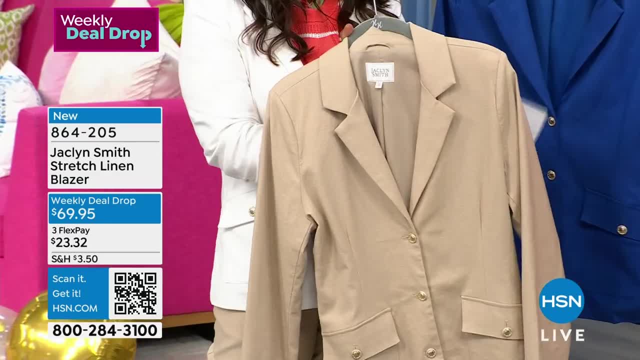 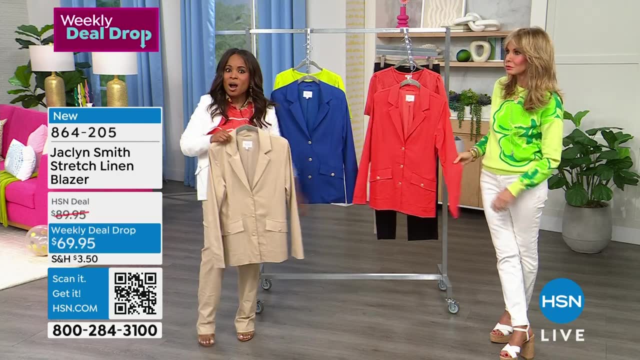 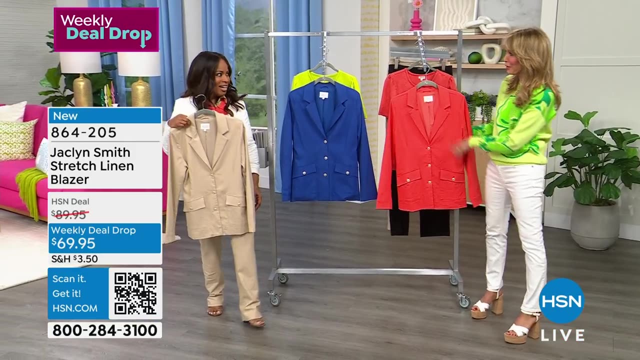 you in the beige, okay, ember glow is the most limited. which is the orange color? that, that orange, that's the most popular and the most limited, and i am not surprised by that. it's so striking. yeah, it's. everything goes with this. i mean from the floral to the maritime tea, to 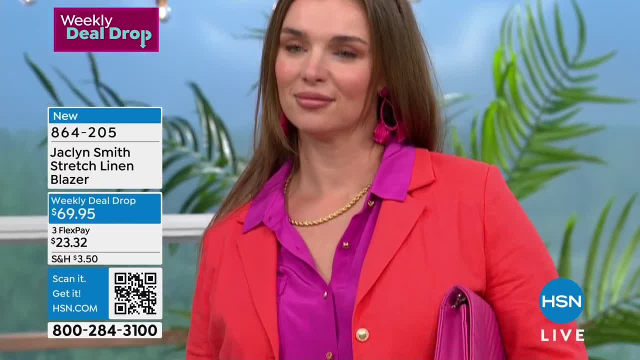 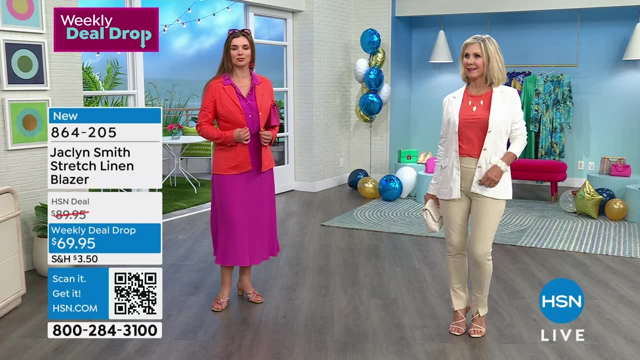 you know the a-line and the camp shirt. yes, all you know shaking it up and bringing in all these new colors with it. if you want the ember glow, which is the color, which is that kind of orange coral look, you'll need to order that one. that one of all the choices is the most limited, i'm so. 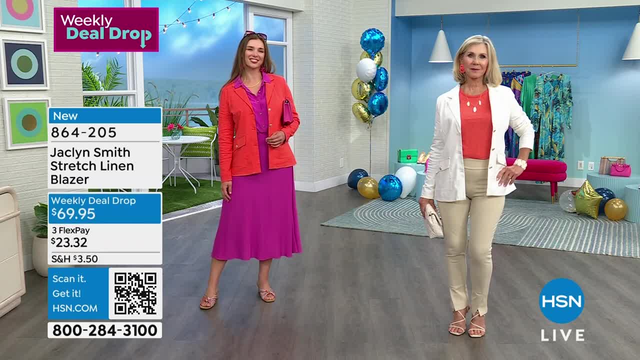 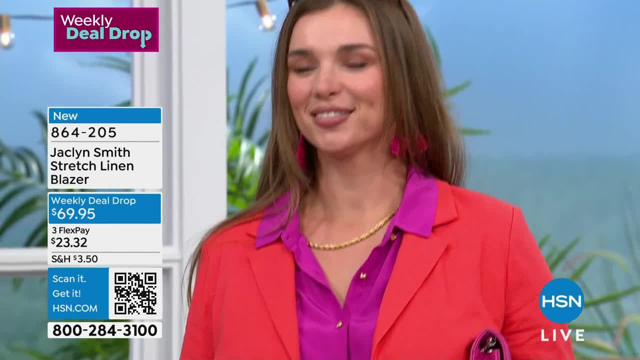 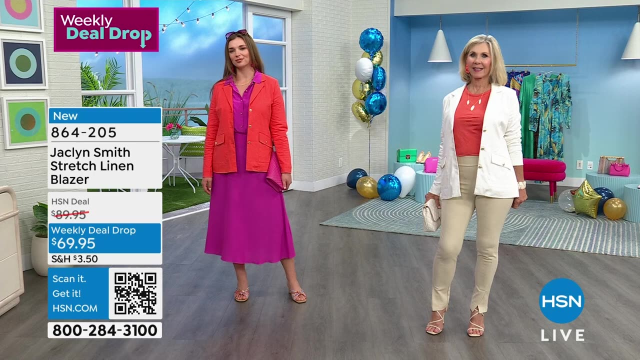 happy. doc mara is in that combination of the fuchsia and the orange and you can see just how gorgeous she looks in that, in that color combination. um, machine wash tumble dry with this. so a lot of times with with linen- remember, this is a, this is a stretch linen. so it has 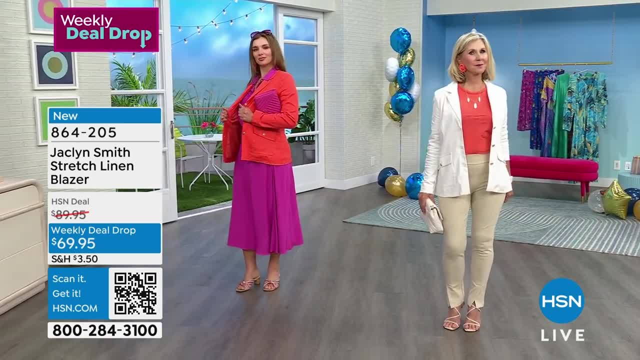 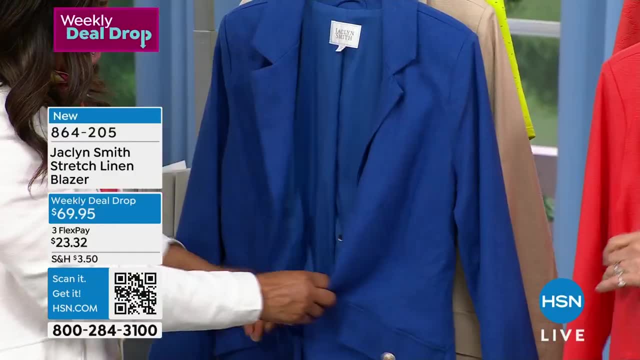 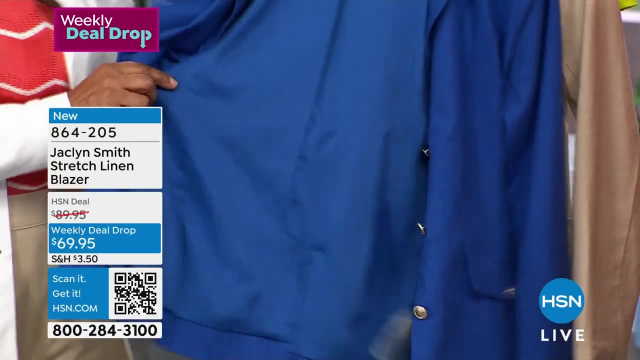 stretch. i want to show you the lining too. the lining and all these pieces are beautiful. look at the line: perfectly matched, color wise, and it moves with you. it's stretched because if not, it doesn't live. look at that. so everything is stretched. you all, we've all kind of ripped or torn a stitch or a lining because it 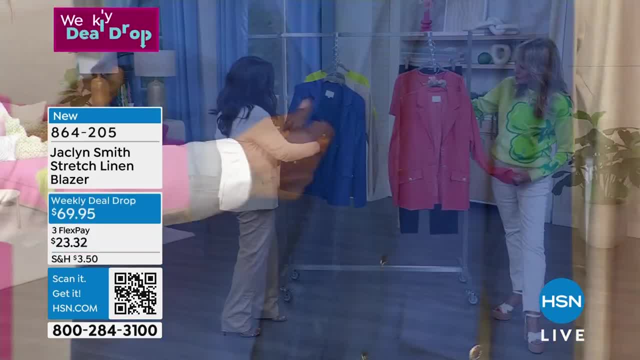 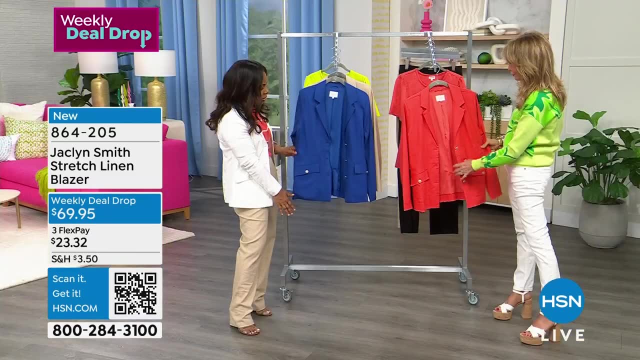 didn't stretch or it didn't give, remember. i think that's what's beautiful about this fabric is that it does lives your life with you and it gives and it falls beautifully, and it's that that casual, chic look that's so easy to wear. let's have some. 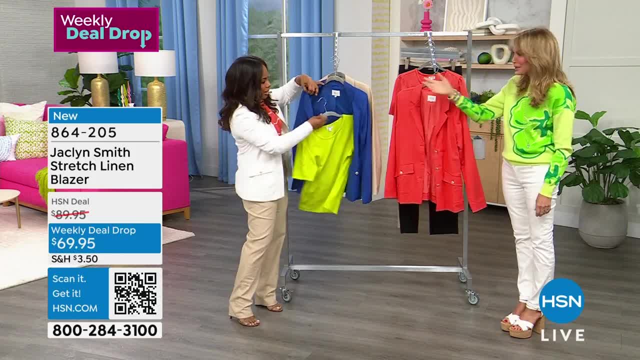 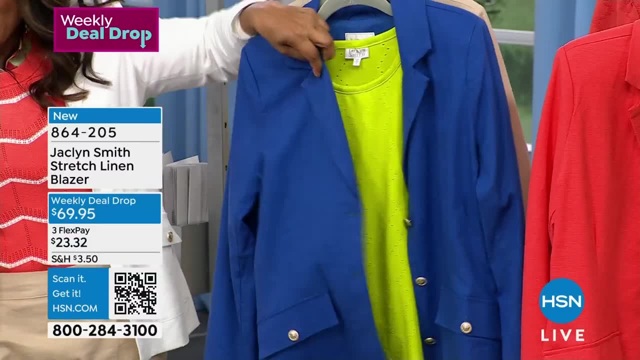 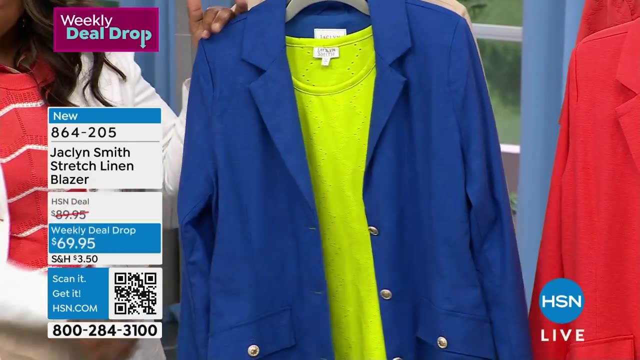 fun with some colors. so this pretty little. this is the one of color. yeah, it really looks great. look at that color combination, how it pops. how much fun is that right? yeah, isn't that great, right? look at how pretty that is. this pretty chartreuse top is coming up and for me, i just do. 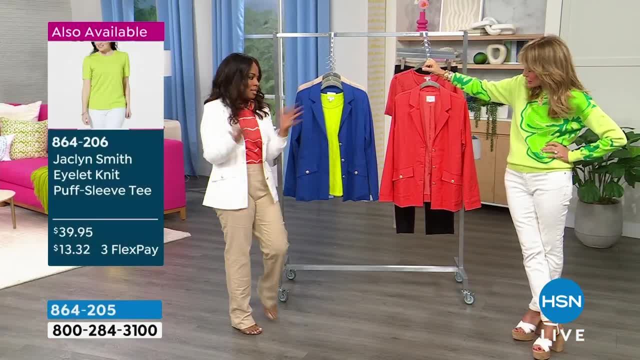 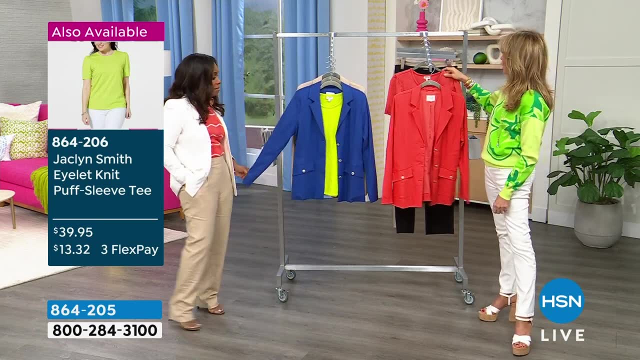 a white anything at the bottom, and then i'm going to go ahead and i'm going to go ahead and i'm going to put one on the bottom, or right, that's it i mean. or just with the with the um wide leg jeans that we had and we do have, um, we do have matching. i don't, we don't have it out on our. 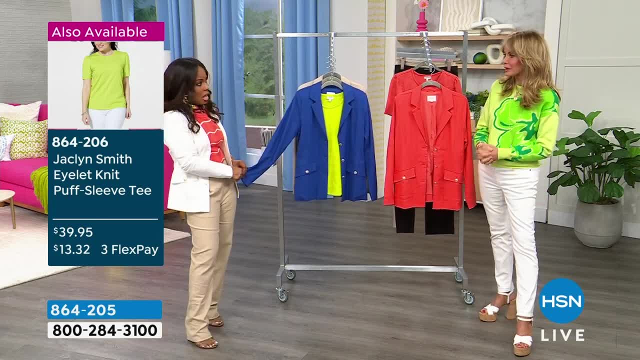 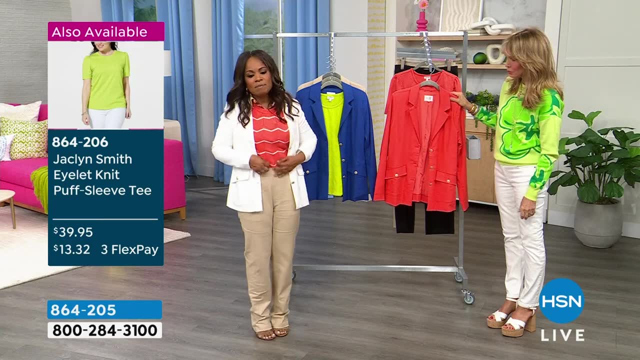 rack. oh, actually they're matching. we have a man painting to that if you want, so you wear it together. our, yeah, separate. we have that look, and even with the top- i have on so many tops right now, you do, how many tons do you? i do? i have on this one, i'm, i'm almost like the, uh, the of the mug right there. i don't care what that looks like. it is so pretty left and shoulder height that one she's gonna bike out of here. she's going to JUNE her own walk up in the retirement home. look, she's going to look like a. okay, you don't really need to try reality. it's all about hot dude. i just move around, you know we will. 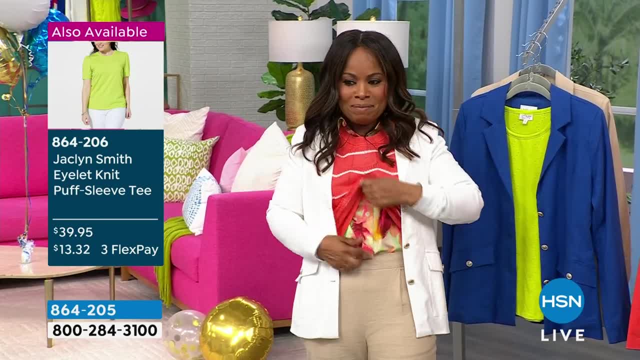 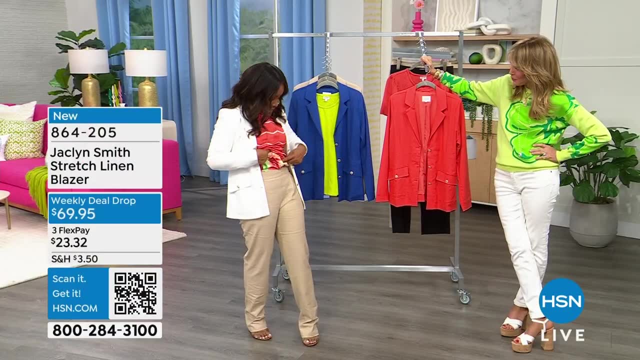 It's almost like the bug where the clown, like I've layered quite a bit. There's a scene on Friends where they just keep adding the clothes, Oh, quite a bit of clothes. But I was thinking how pretty this will look, this floral top. 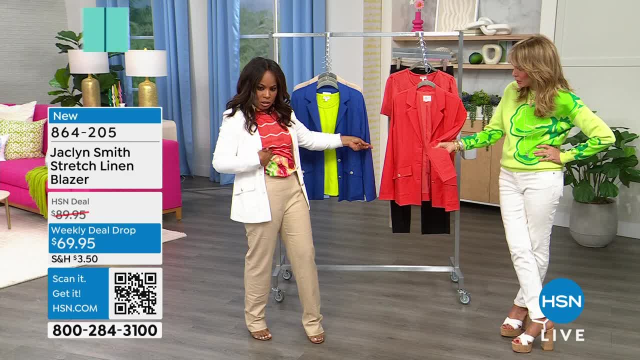 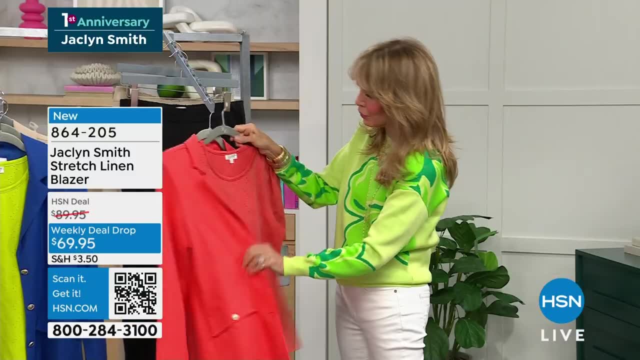 I think we're calling this one. Oh, it looks beautiful With this particular, with that particular ember glow that we had a little bit earlier. I mean everything goes. I mean you can do the tone, You can do it, you know, with a white tank. 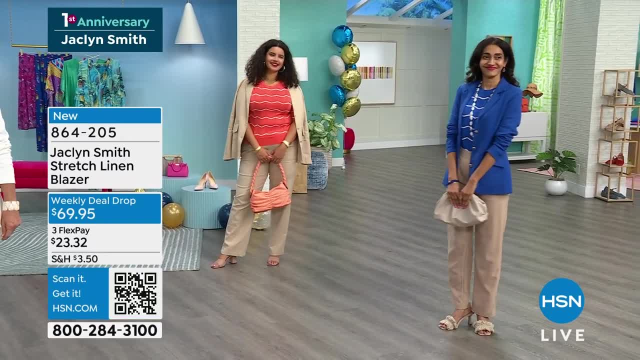 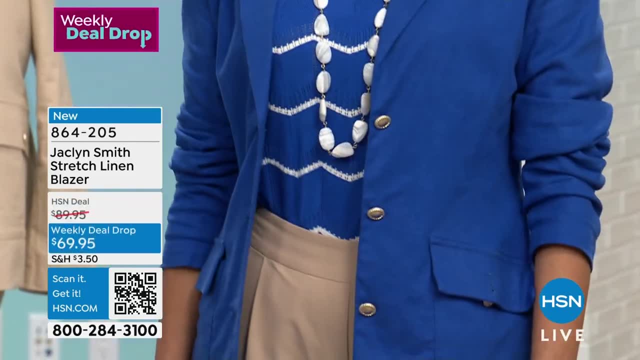 It all is interchangeable. Well, if you'd love to shop, come on in, Take advantage of it. Remember our weekly deal drops are only for a limited time. Let's talk about model sizing. Let's encourage you to choose your size early on. 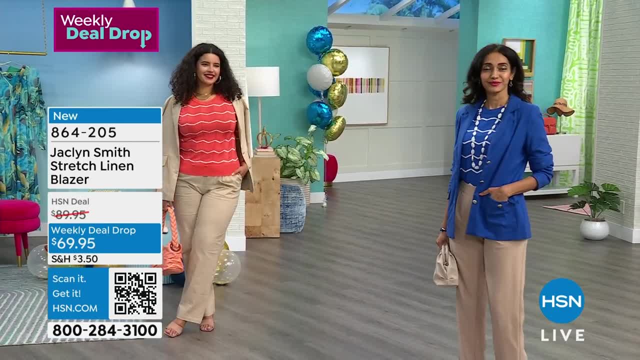 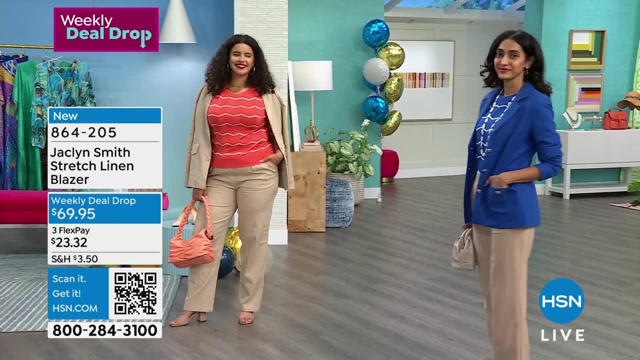 We're looking at Simi. Simi is wearing the blue. Simi is 5'7". Her numeric size is 4.. She's wearing the extra small. She's wearing the same sweater that I am wearing, along with the beige pant. 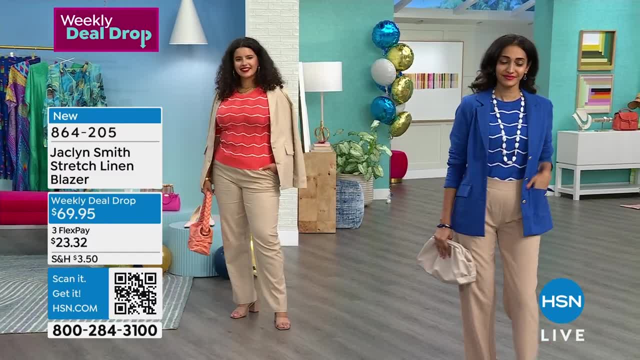 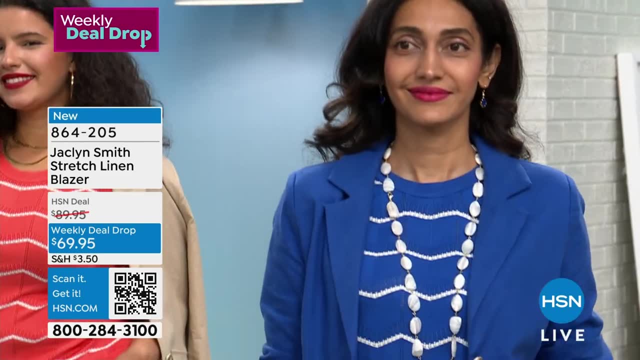 and she looks great that way. But that blue jacket, imagine that, just with the white front, a white cotton button top that you have at home, right Right, a white cotton shirt, Yeah, shirt. It just looks great, And you can put that on with a pair of jeans and flip-flops. 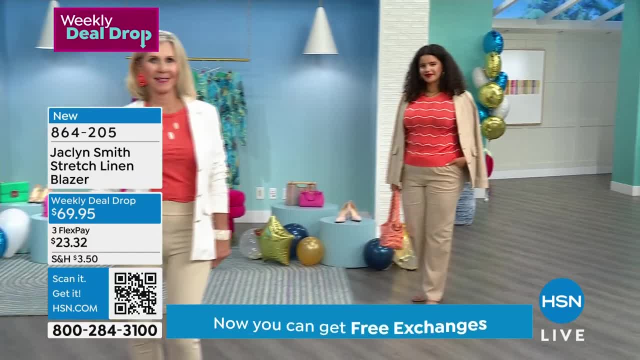 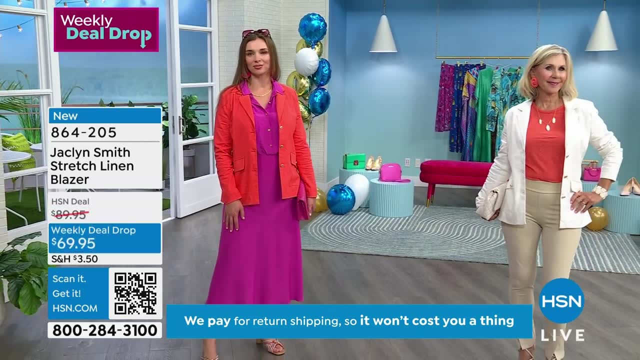 Believe it or not, Tennis shoes, whatever Sneakers, You dress it up, you dress it And you look great, Right? Because that is really the benefit of having a blazer, no matter how casual. You talked about your daughter wearing this with her yoga pants. 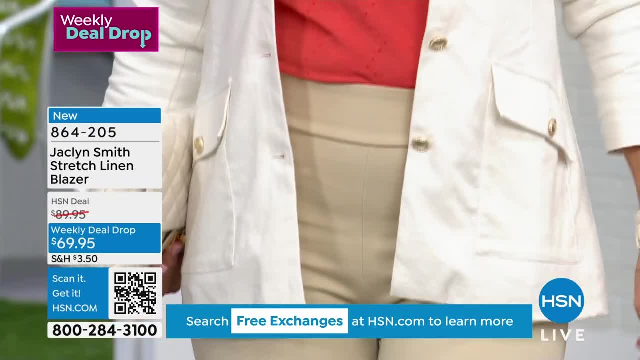 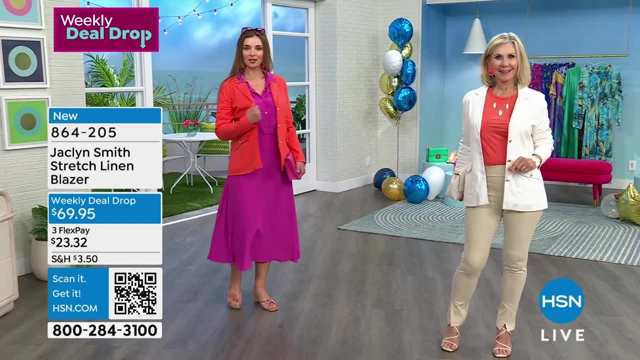 Yoga pants. just because she's always cold, like me, She puts it on and it's sort of a look. She makes it work. Yes, I mean, I love the beige with black too. Yes, That's a great look. 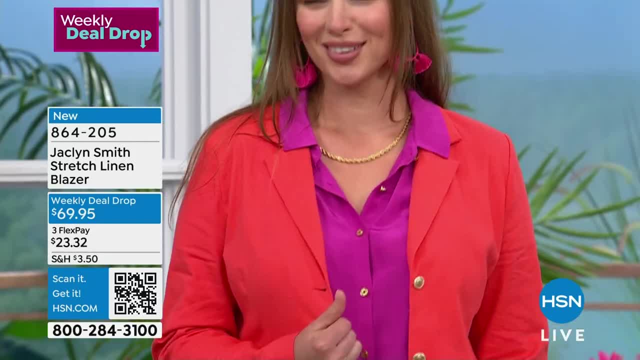 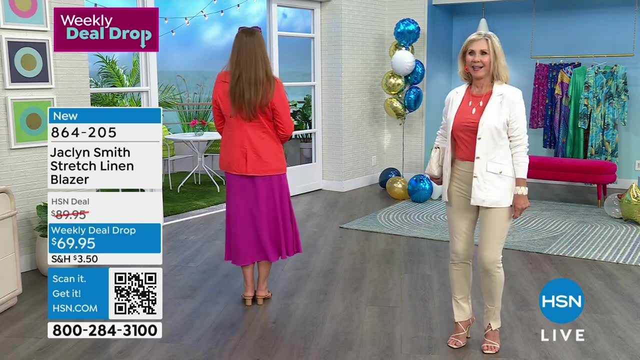 Very sharp look. That is a very great look. Yeah, that's great. And then you go back to what's in your closet, what your favorite pieces are. I mean these linen blazers. I love you, I want to show. can we show Jacqueline with the white? 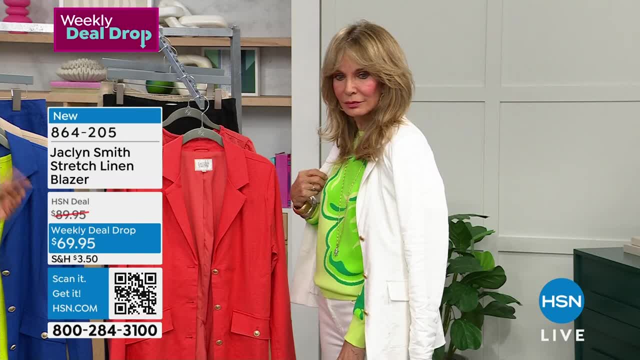 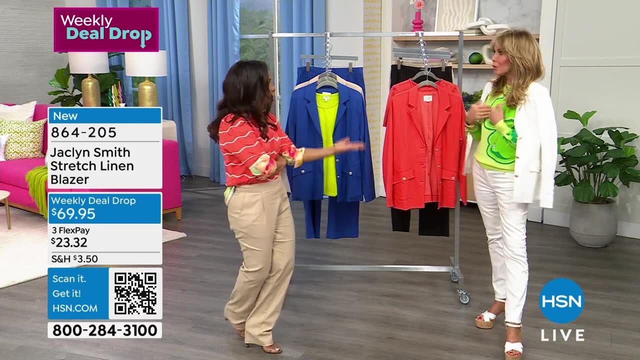 So she now has on the white blazer and look at how great this looks with the sweater and then in the jean. Isn't that pretty? So if we were going to meet for brunch, that would be so pretty. Yeah, You know. 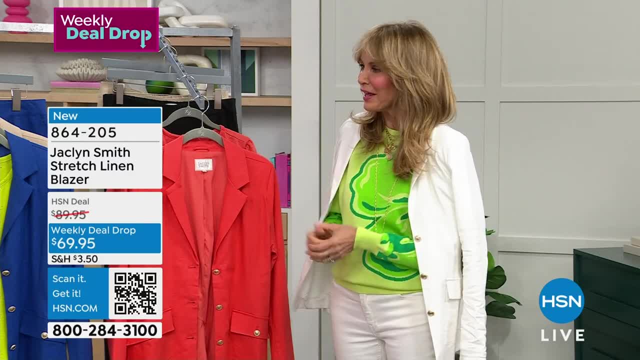 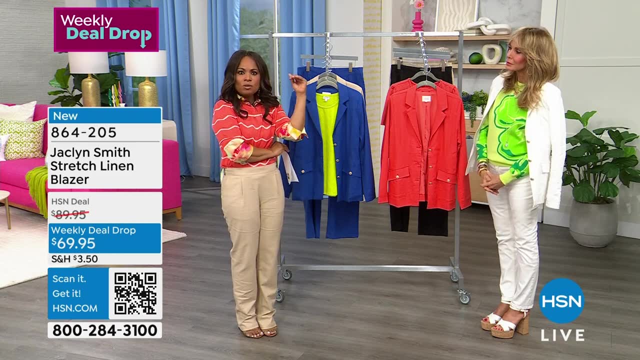 Absolutely, It's perfect. You feel feminine and pulled together and fresh and perfect for the season. Yeah, and it's the blazer with the gold buttons. You know it just scales your look. Yes, And you know you look really chic and very elevated. 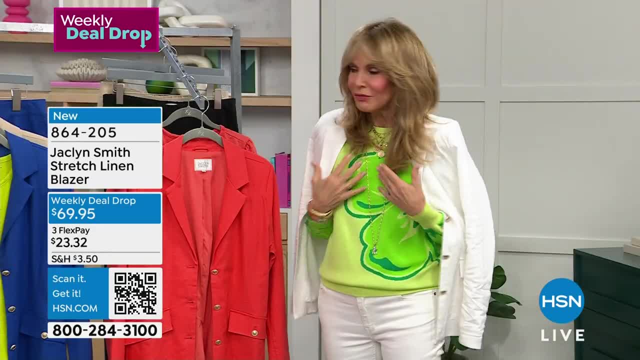 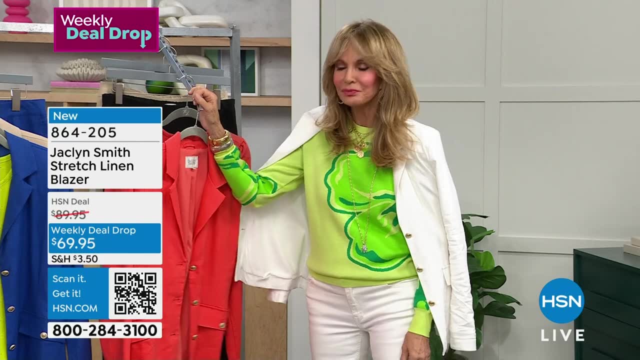 Well, this third, this steps this up. Yes, I mean, even though I feel great I'd go to lunch in this, but you add the blazer and it's that third piece that finishes your look. It almost makes you get a little bit. 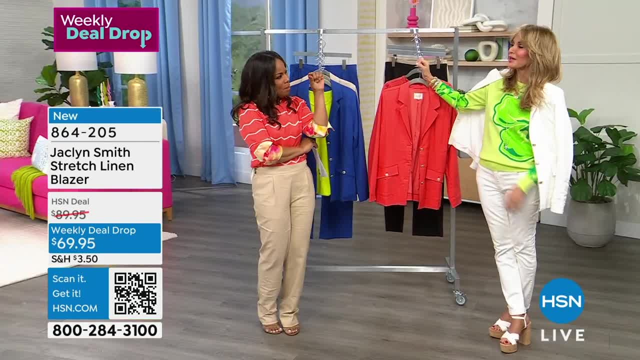 makes you look a little kind of, you know, kind of unimportant. Right, There's something about it. Right, A little step up, A little step up, It steps up your game. Yeah, it really does, and that's why they're so valuable and so important. 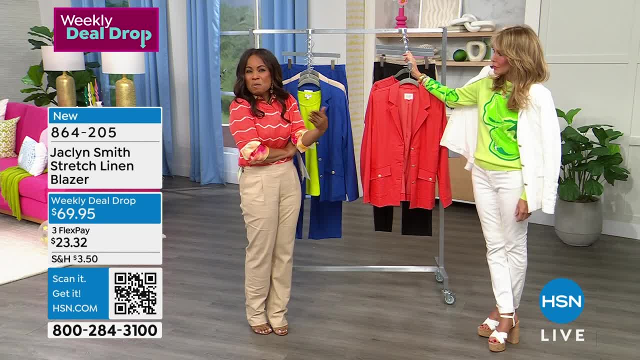 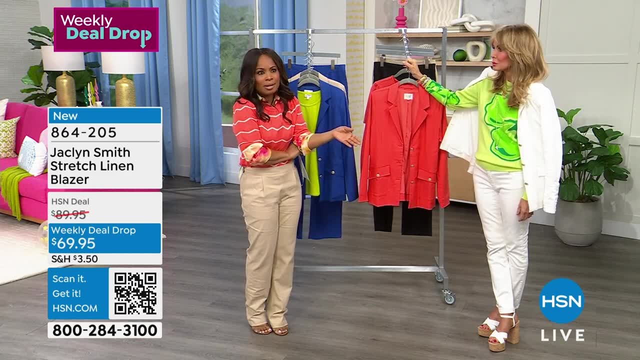 You know we talked about, you know, from a job interview, just out to dinner, or even casually, pairing with a pair of shorts. As unusual as it sounds, it looks so cool together. Right, Let's get you on board. It's a weekly deal drop. 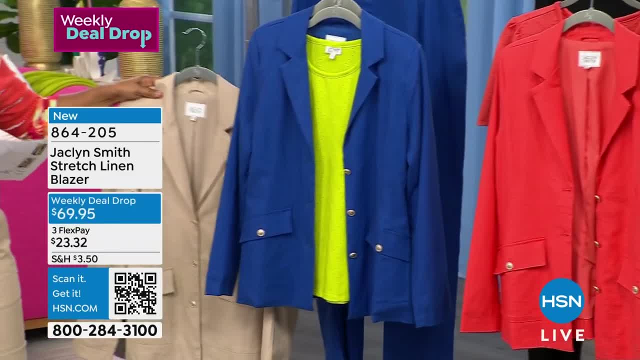 You have all the colors. Here's your beige, There's your white. Let's show you all of our models and their heights. Let us know: Extra small through three. Well, extra small: 3, 3-6.. Well, extra small through 3, 6.. 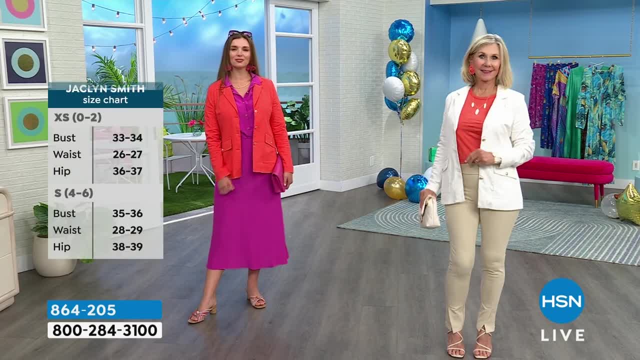 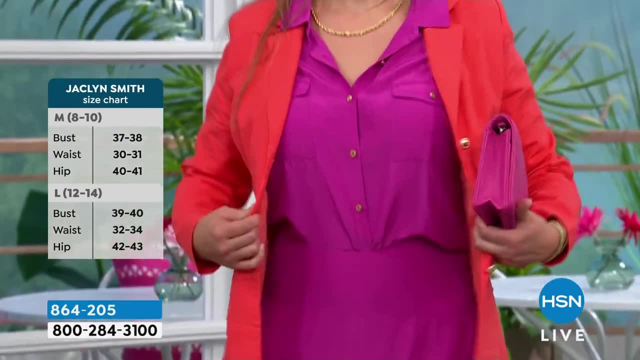 Well, extra small is sold out in all the sizes, but we have sizes small through 3X available. Let's show Dogmara. Dogmara happens to be 5'9". She is an American size 8, and she is wearing this in the medium. 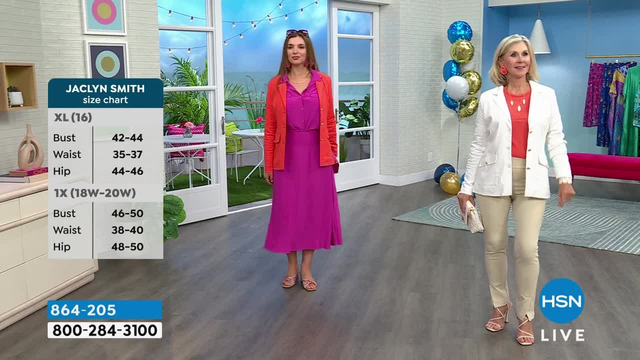 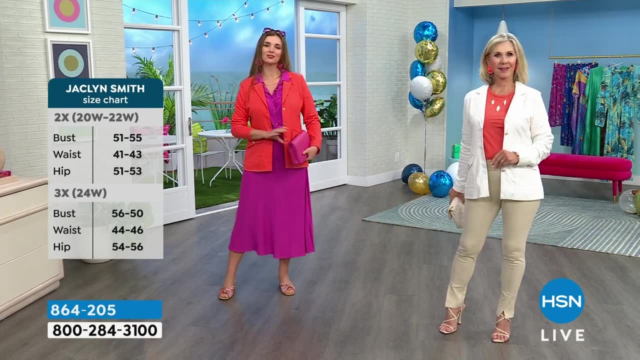 and she's in the number one best-selling color, which is that ember glow. So if you love that orange, don't wait. I would place your order right away. It's available on FlexFay. Don't forget that we're offering you $15 off once you are using your HSN card. 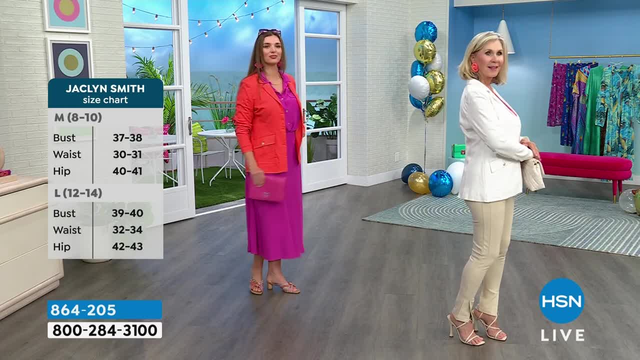 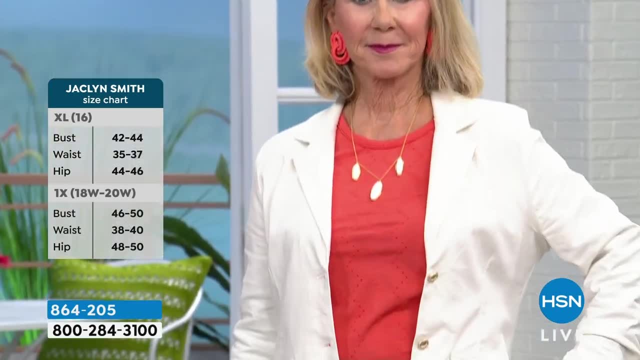 and you have purchased $75 worth of merchandise. Be sure to check out, but don't miss out on that ember glow. Here's white and Vonda is wearing the white. That's another one that I've had. I like them all. 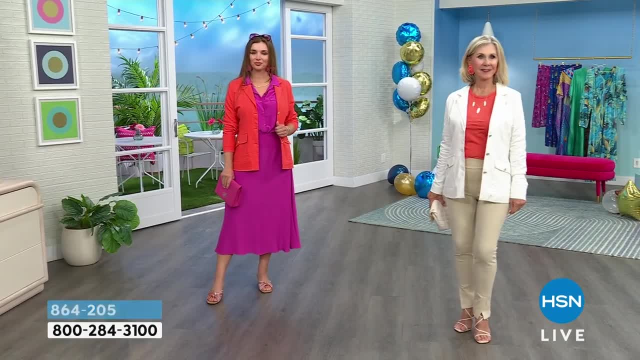 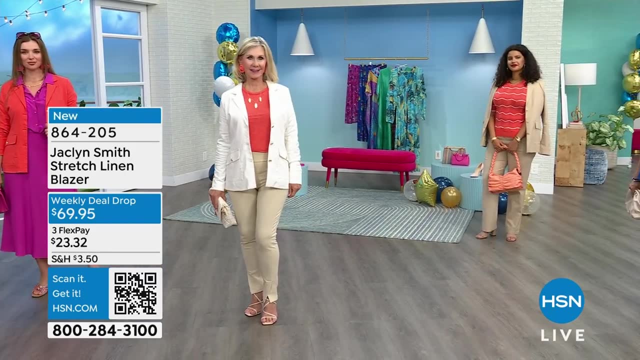 It's hard for me not to. I like them all. The white is spectacular. Vonda is 5'6" and she is an American size 6, and she's wearing it in the small and it fits her beautifully. On Vonda you'll notice the slanted pockets. 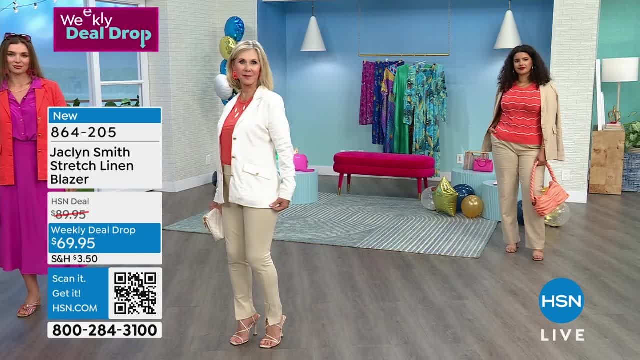 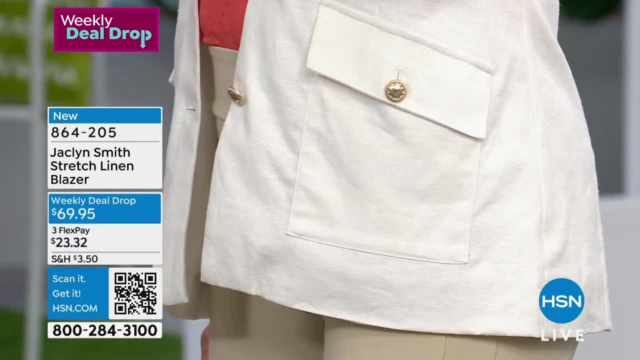 I don't think we get a chance to talk about it this time. Very slenderizing: We did it at a slant so it didn't add bulk or punch out on your hip line. It makes your waist look smaller. It makes your waist look smaller. 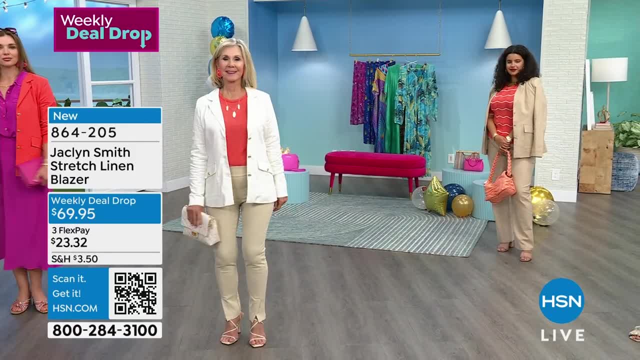 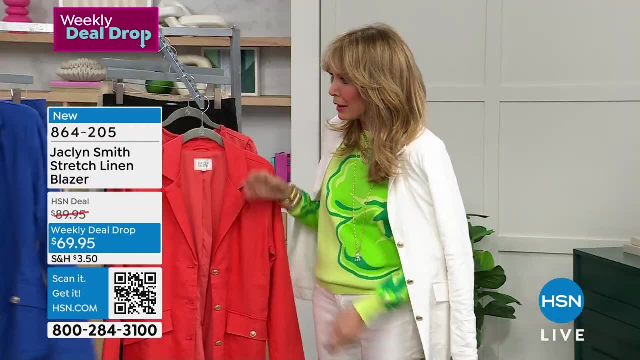 It gives you the illusion. There is a shoulder pad here. Yes, nice Subtle shoulder pad, notch collar and the gold buttons. Well, they're not really gold, They're sort of a mixed metal. look that you can wear gold or silver with. 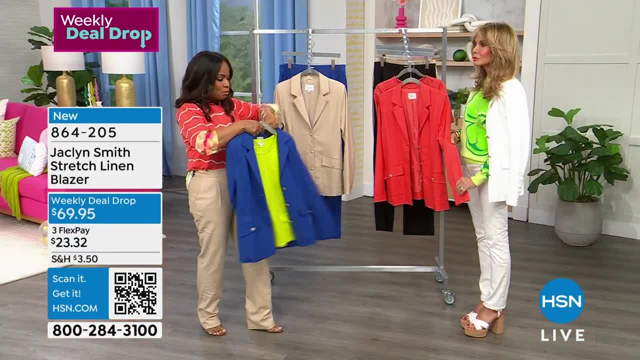 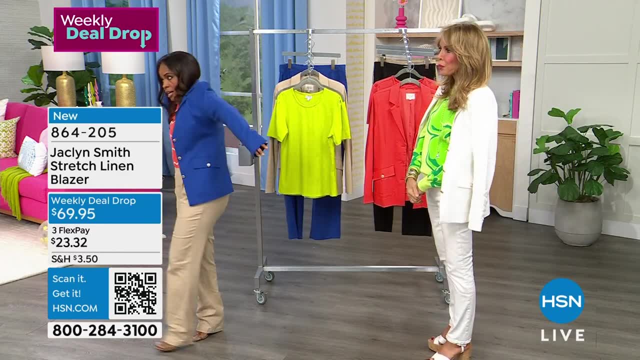 I think it's beautiful. I'm going to go and I'm going to stop next to our models only because I am 5'4". I have two, so I am the petite one in the room, if you will, and I am wearing this in the small. 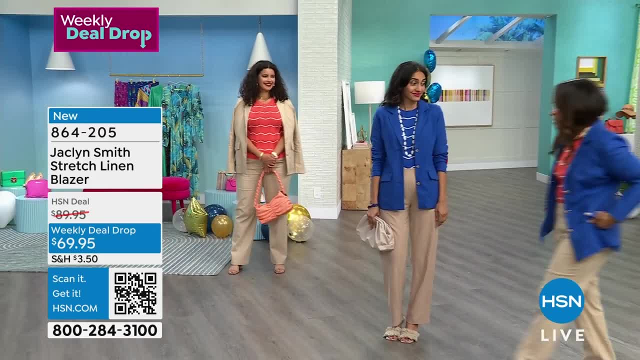 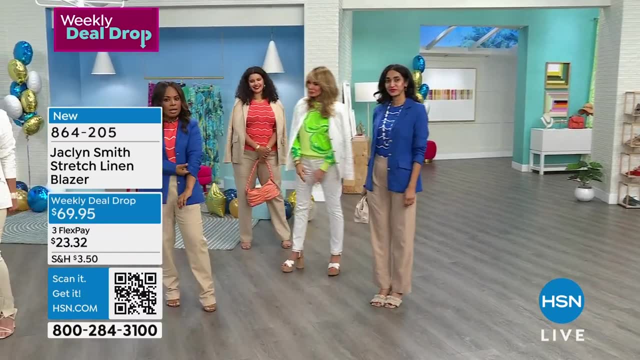 Earlier I had on the extra small. I like the idea of being able to wear either one. I'm going to come next to you, Miss Simi, but just so that you can see, I have on the small in the petite. 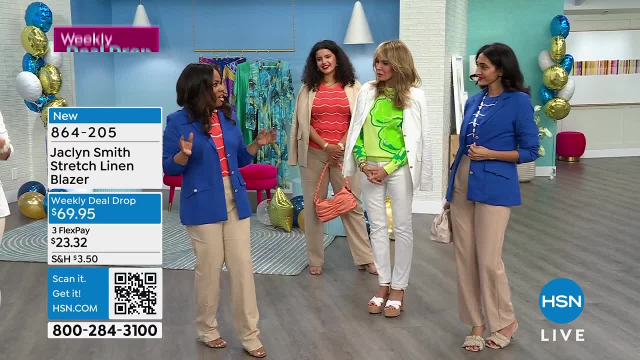 but just so that you can see the length and where it hits me, Isn't that just? you're right, It's that third piece that you put on and it's just so yeah, and very just kind of It's so comfortable. 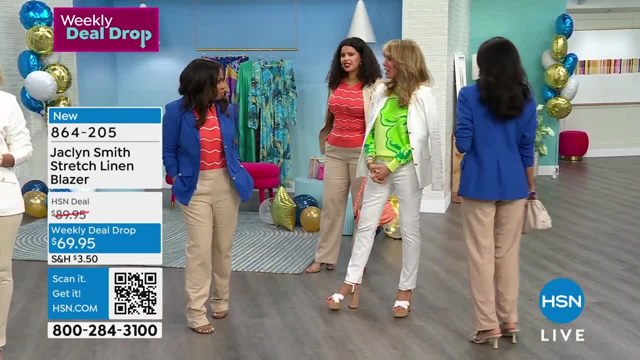 It's kind of casual chic and you just look, I don't know. You look pulled together, Pulled together, Right, like we've been styled Just a little bit of a blazer wherever you're going, right, Right. 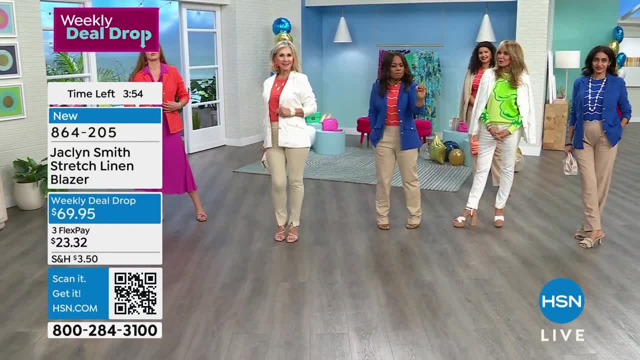 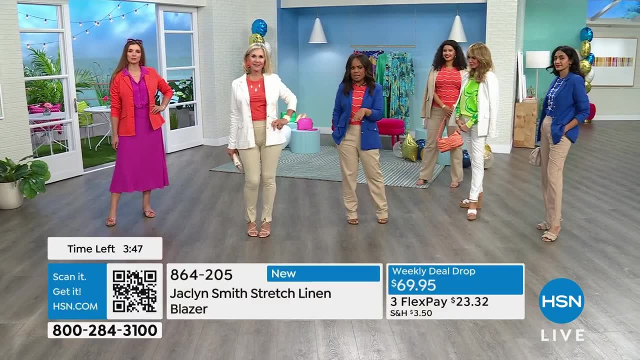 You just look, just that, that's. that's the. if there's one little takeaway, I think, from tonight is that a blazer is such a great investment, whether you're buying this one or anyone in the future- how it really just steps up your look. 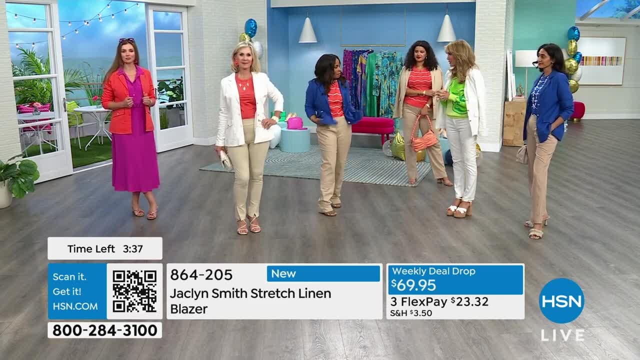 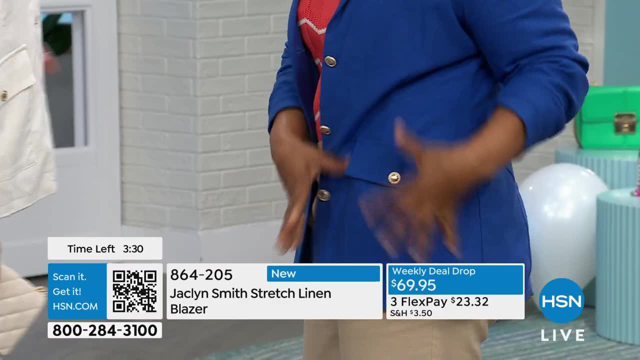 Yeah, a blazer's here to stay. Yeah, No doubt, No doubt, No doubt. This one is so easy because it's it has stretch. So when we say a stretch linen, most of us think of linen that's stiff and wrinkly. 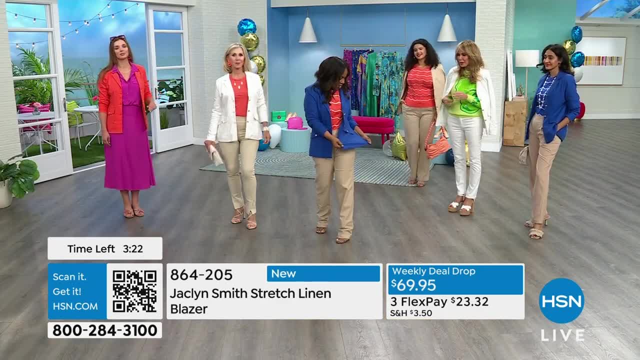 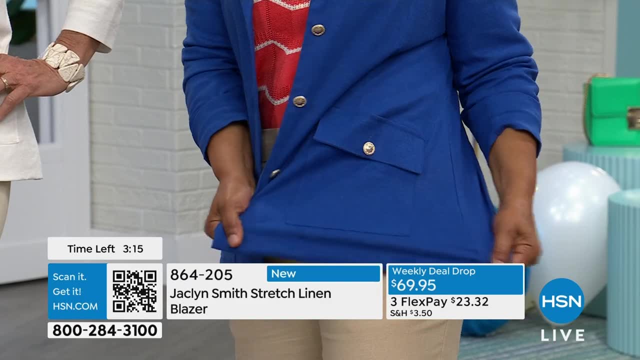 And sort of scratchy And wrinkly And by the end of the day This is, I mean, a lived-in look is. This is almost like a fabric. Right, It's because of the stretch in it. You can see there's a give to it. 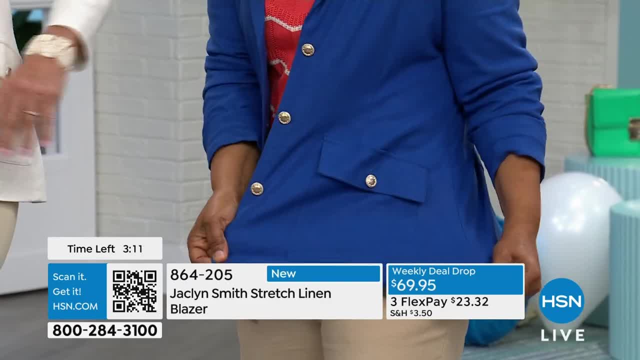 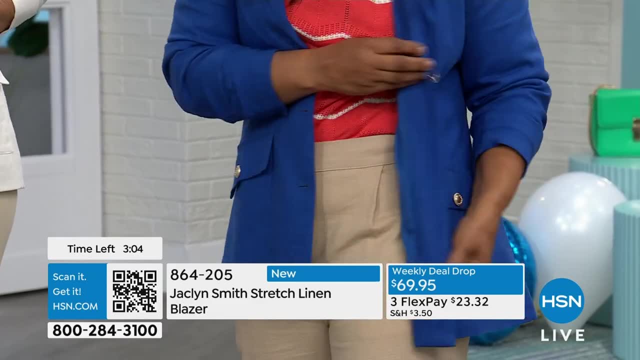 and it's even in the sleeves, just throughout the entire body. So there's a stretch and you can see how the fabric doesn't work. It doesn't wrinkle like traditional linen, And what I love, too, is look at how beautiful it is in the inside. 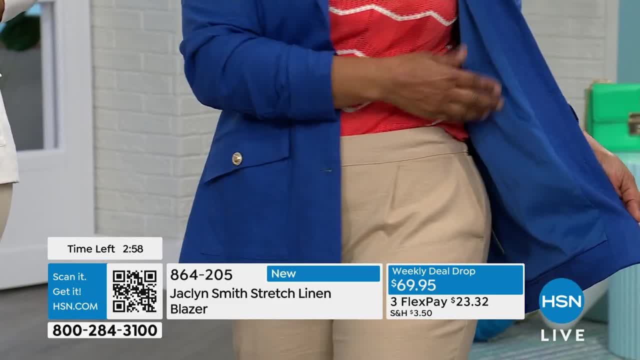 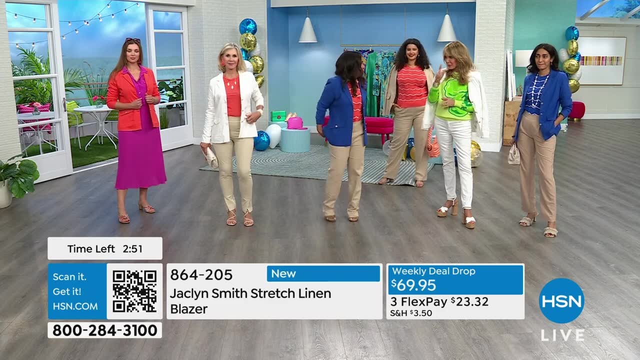 Yeah, Stretch lining. A lot of designers cut corners where the inside lining would be a completely different color And not stretch And it wouldn't be stretch. Well, that's my customer out there, Your good advice for the stretch lining. So I see you on a cruise where you know. 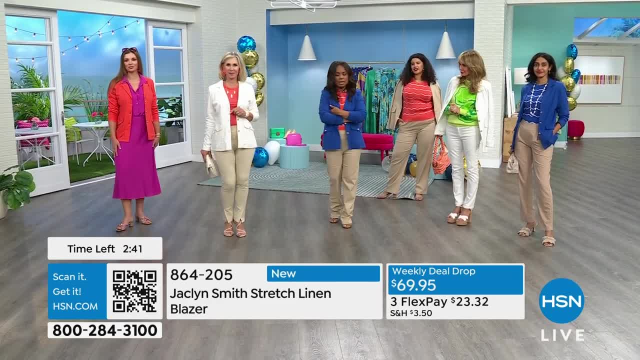 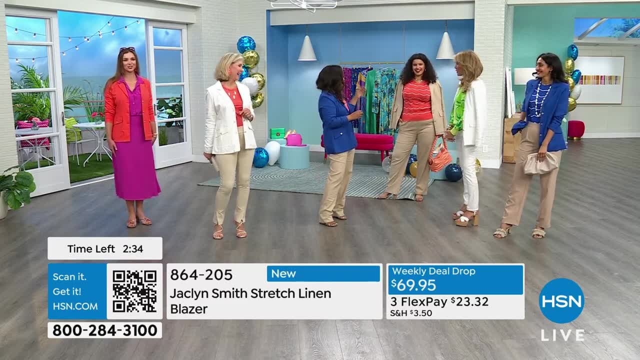 you might be going to the captain's dinner or you, you know you maybe, maybe you can do a little casino thing happening on the cruise. I think they do that on the cruise. She's got a lot of fun. Yeah, a little happy hour is great. 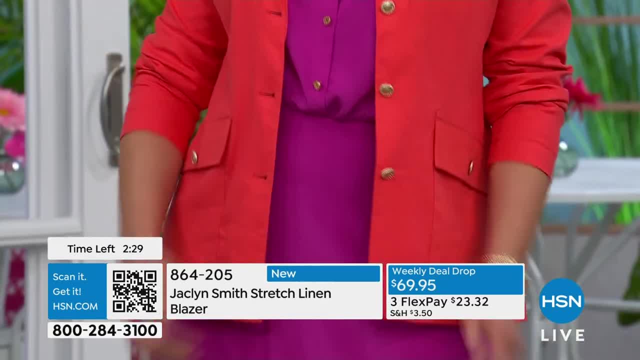 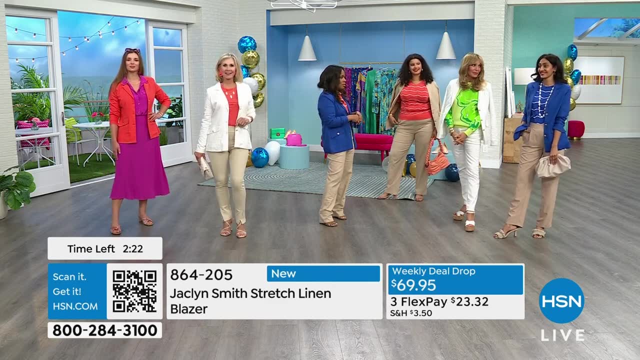 I love a good happy hour, Yeah, But when the sun, when the sun sets, it gets a little cool out. You put it on. I wore this all over India. Yeah, I had it in every color. It's gorgeous. 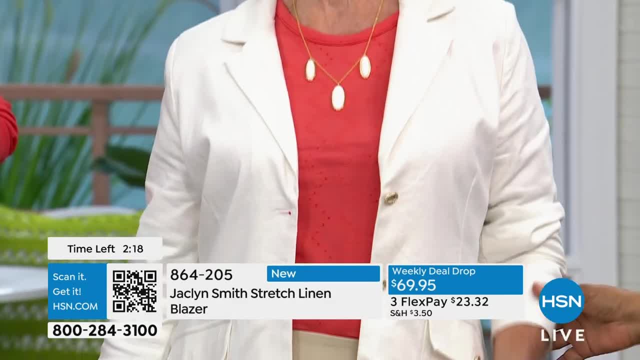 Yeah, It's so beautiful And the feel of it is very elegant. I love how you've ruched up the sleeves a little bit. Oh, we did the throwing of the colors, You know, and I love Doc Mara's look is one of my personal favorites. 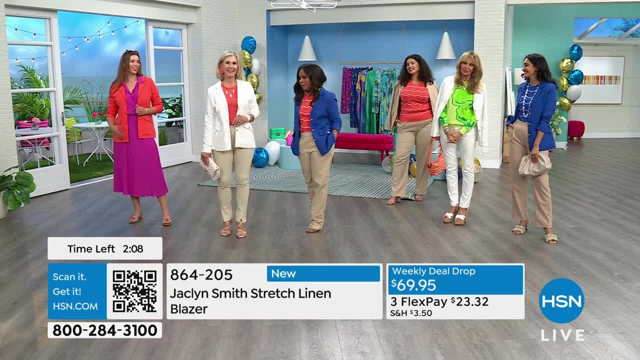 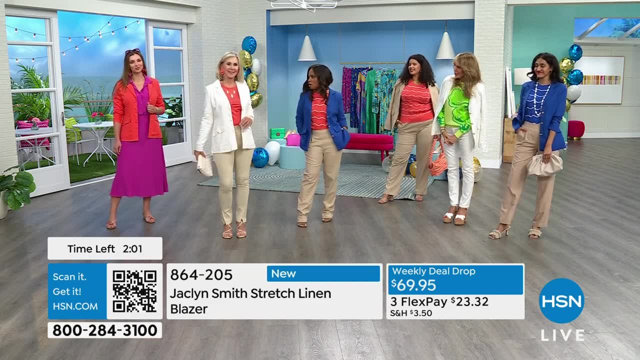 I'm going to buy that whole outfit, girlfriend. We're going to be twinning So beautiful, Beautiful people. I'm buying that look, That color combination I think is stunning. Yes, Yeah, You know, and so, and if you like the look that Doc Mara has, 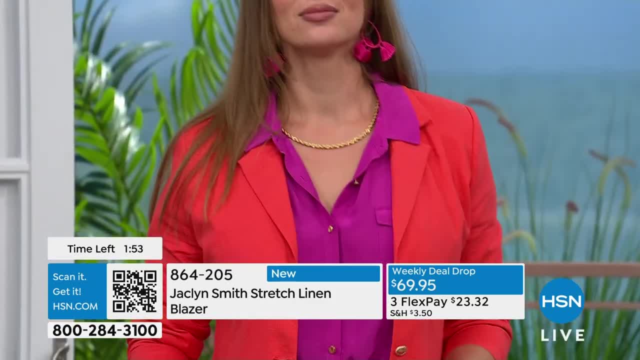 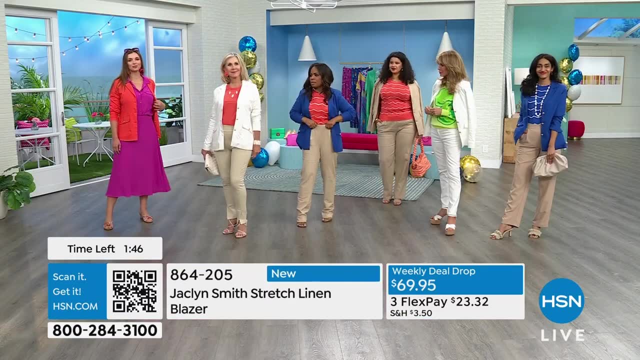 she is wearing the fuchsia top and skirt And those pieces are what we're calling customer appreciation price. They're so affordable, So be sure to go online so you can certainly recreate that look. But any of the choices I think are terrific. 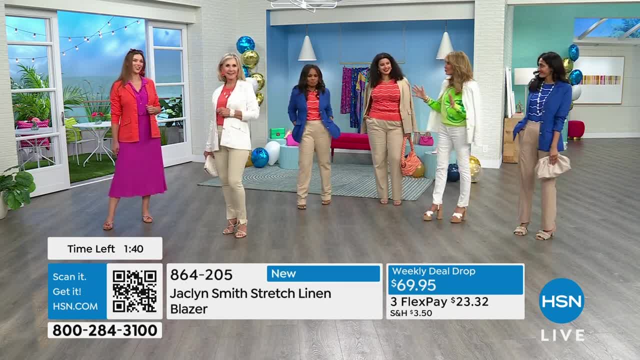 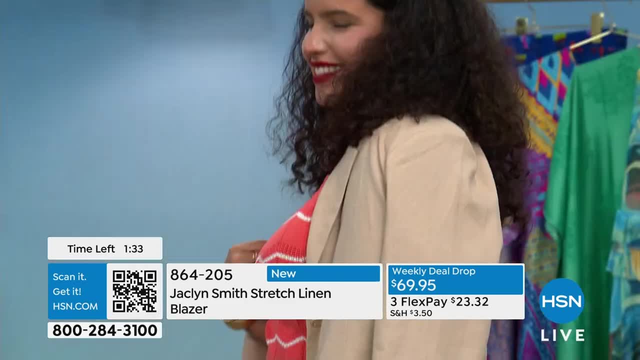 They're all great And everybody has made it. Thank you Made it look so beautiful. Yes, And you can see the beige over the shoulder. So, from the office, think about wearing these to the office, because why wouldn't you? 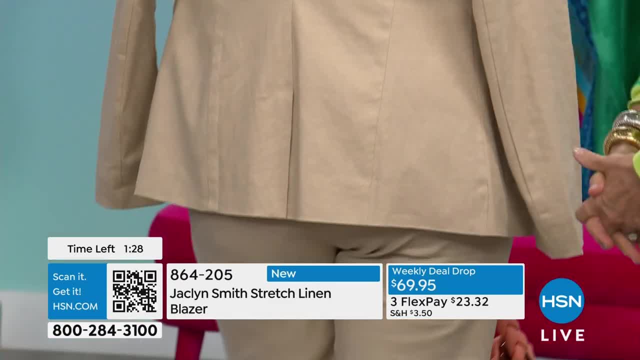 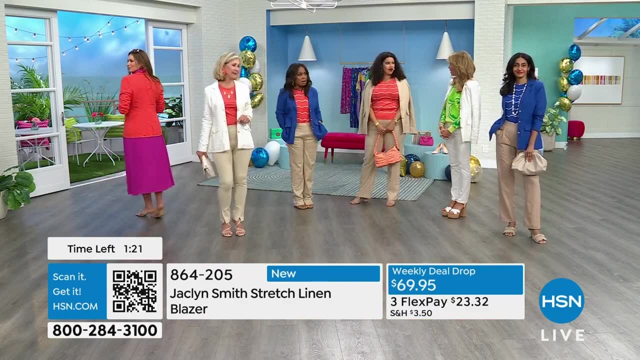 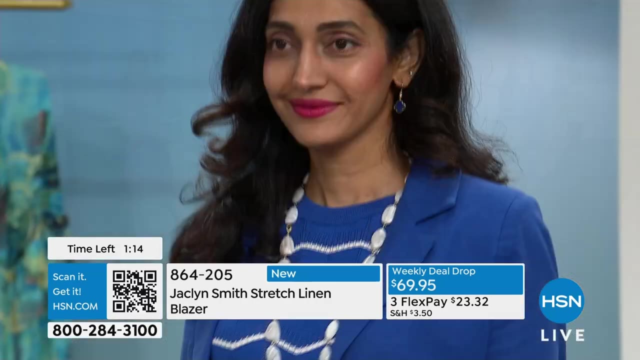 Many of you have workplaces where you do need to wear a blazer. They say: dress for the job you want, Right? Have you heard that before? I think that's what- I certainly have. I think it's important. I try to tell a lot of the young people that I work with like, listen, some things never change. 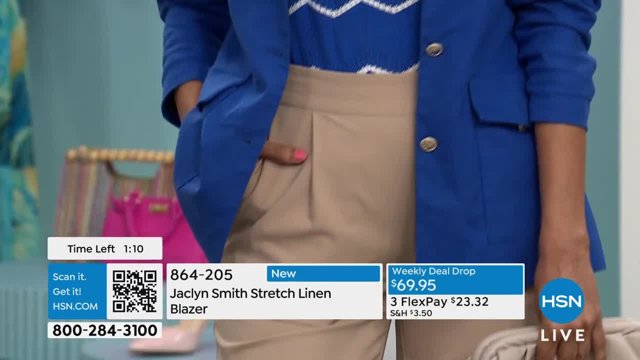 That's right. That's right. You, you, yes, Dress it up. You know I'm- I'm telling you that, Yeah, I'm old school. Listen, dumb, things never change And old school is the best school. 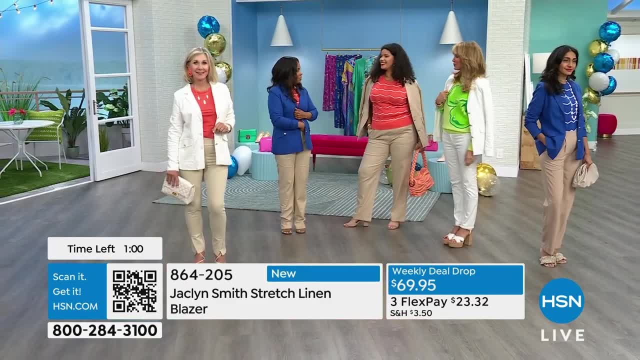 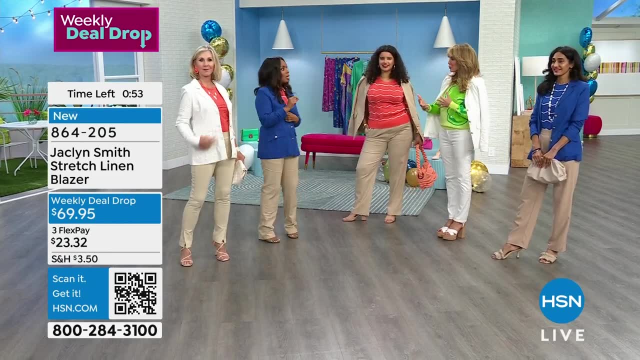 It is the best school. Yes, Dress for the job you want. I think a lot of times the young people just come in casual and- A little too casual, A little. yeah Right, You need to dress-. Let's respect the situation and the job. 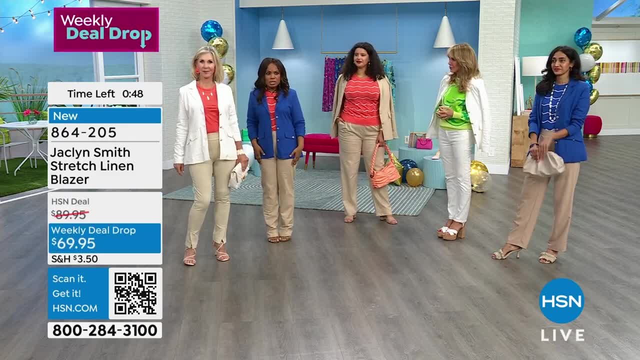 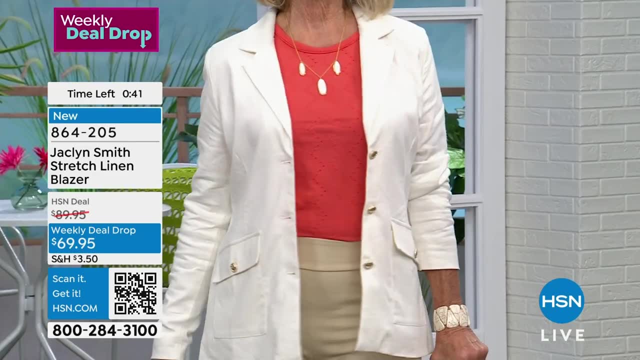 And people notice. Even if you're gonna pair it with a pair of jeans, even if the environment is more casual, you still wear a blazer because, guess what it's going to do? It's gonna make certain that you get noticed and people will notice. 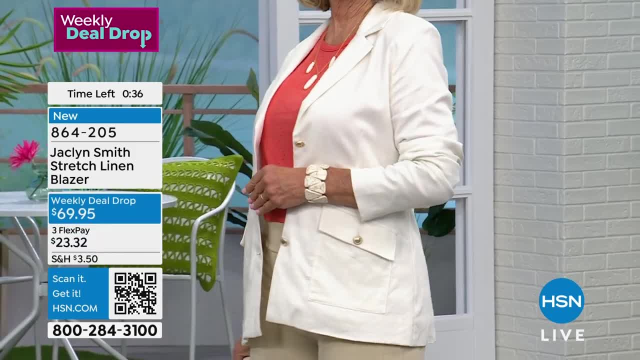 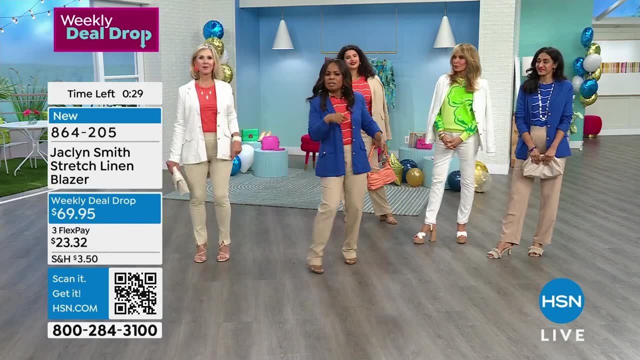 They may not say anything Right, But they notice That you folded together and showed respect. Yes, Yes, First impression is because before people even know your name- they may not ever know your name- they'll say: you mean so-and-so, that always wears some nice blazers. 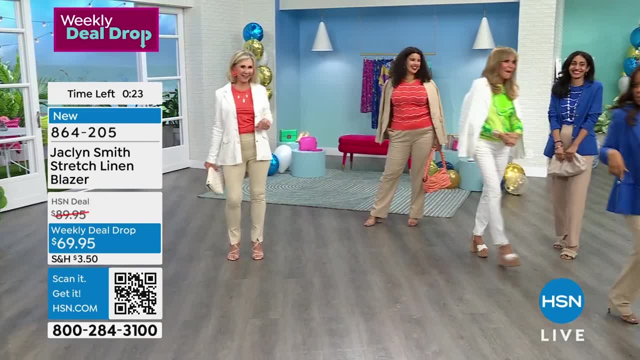 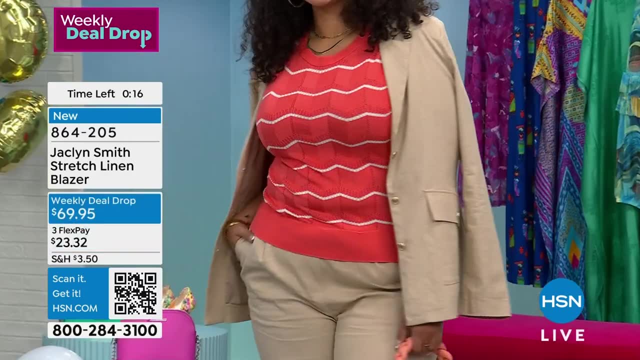 That's always well dressed, Mm-hmm, See, The one that's always well dressed, Right, Am I right? Yeah, very right, There you go, Very right, Yeah, Yeah. so these are, these are really- and the same thing is true for us- that people. 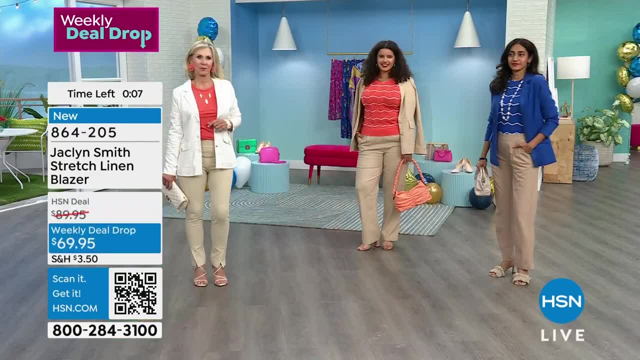 will notice us Right. The one that's always well dressed, Setting an example, The one that's always pulled together with the blazers Right, Always looks so nice. It is Always is dressed so elegantly. Who is that? 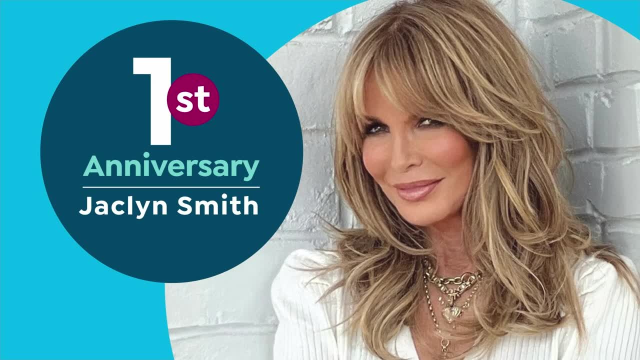 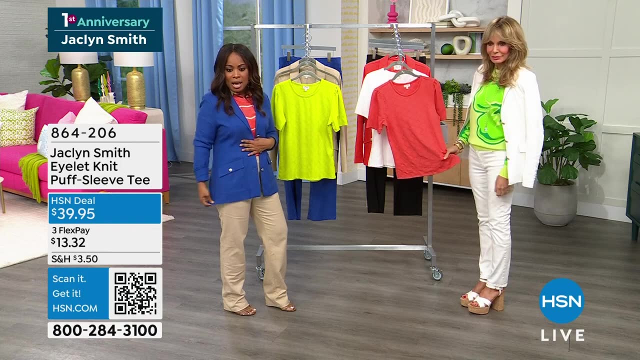 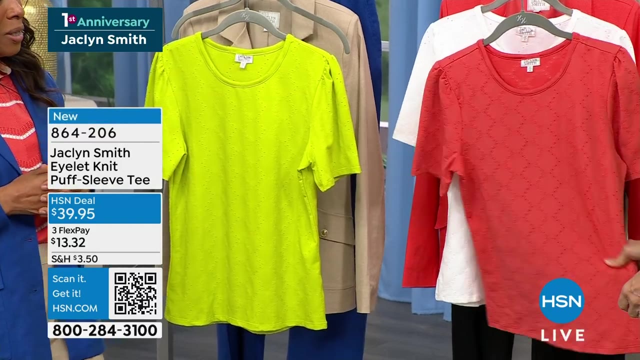 Is that you And these blazers, Mm-hmm, You know, go such a long way with that. so choose the colors that you love. They are weekly deal drop and especially if you want some of the brighter colors. We are going to talk about this great puff Sleeve T and we are so excited to share this. 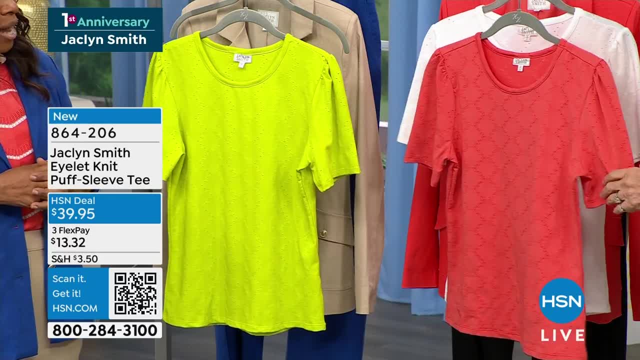 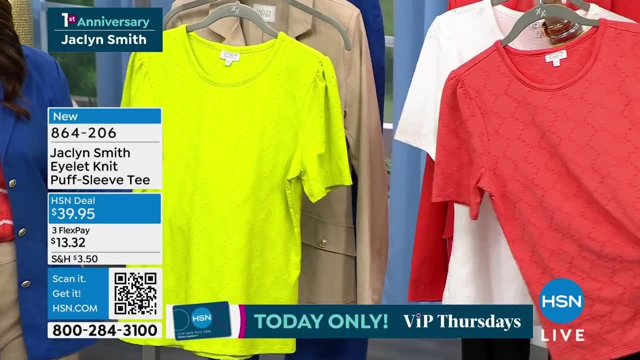 with you. You're next to the Ember Glow and we have it in white. This is the famous color today. Yes, it is. And then I am next to Chartreuse, which is kind of that bright kind of combination of yellow green. 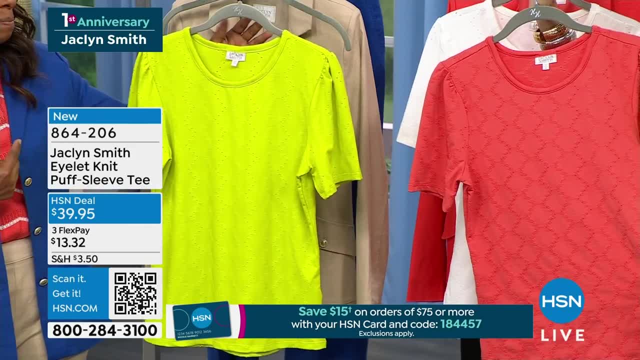 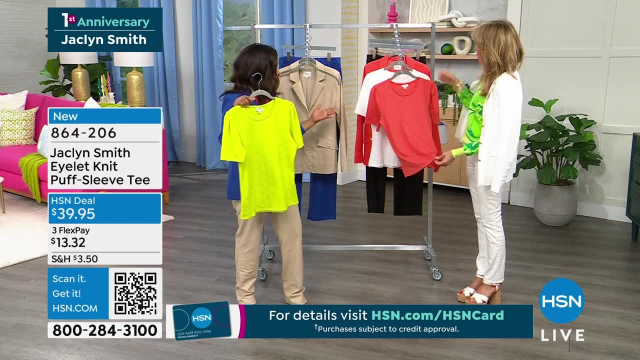 Yes, Which is so pretty and beautiful Wakes you up. Yes, that will wake you up. Sunshine, It's terrific And, if you wanted to- and, by the way, the Chartreuse is half gone- Great. All of them are. 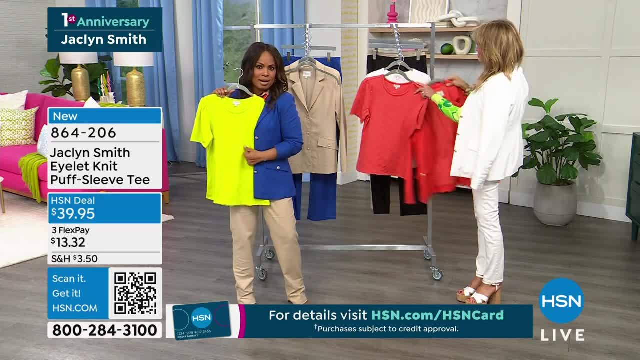 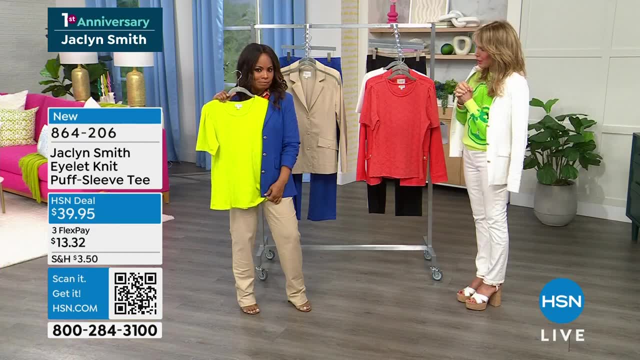 Oh, wonderful, Yeah, Which is great. It's so pretty. And if you want to pair it down, the blue and this Chartreuse together. Winning combination: Again, the unexpected wins the race. Yeah, Gorgeous together, Yeah, If you can put those two together. 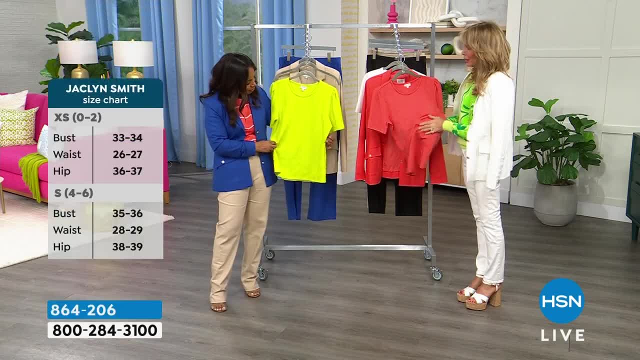 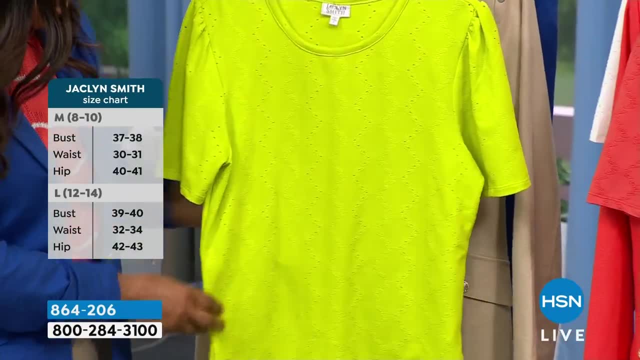 Let's talk about some of the details on this one. Well, this is not your common tee. It has this beautiful eyelet pattern that looks like a honeycomb and it has the little puff sleeve- Yes, So when you take your jacket off, you still this stands on its own and lives on its own. 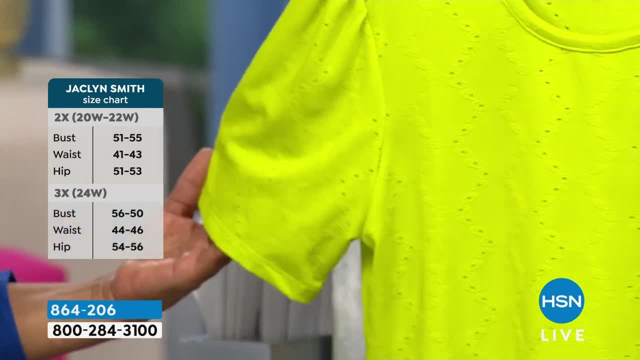 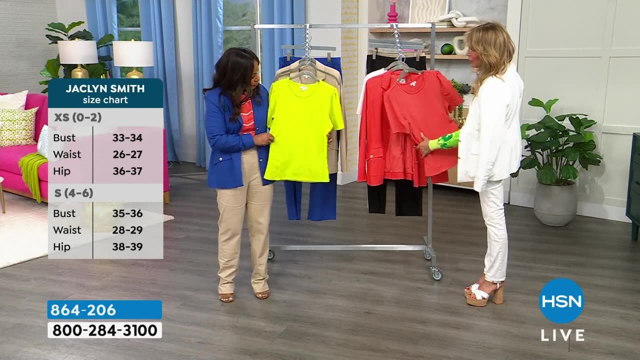 It's pretty, It's feminine. It steps up the game of a t-shirt. What I love is the stretch in this, but it's not too clingy. It drapes on your body and it doesn't grab areas you don't want to. 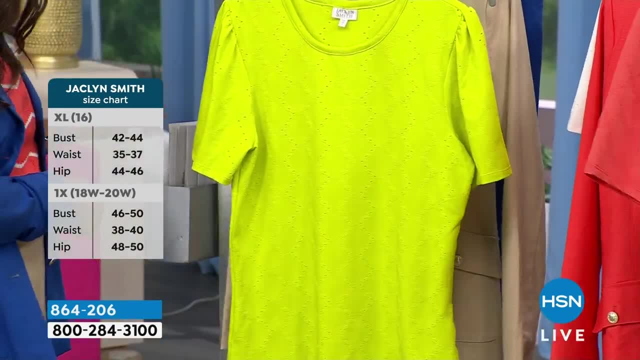 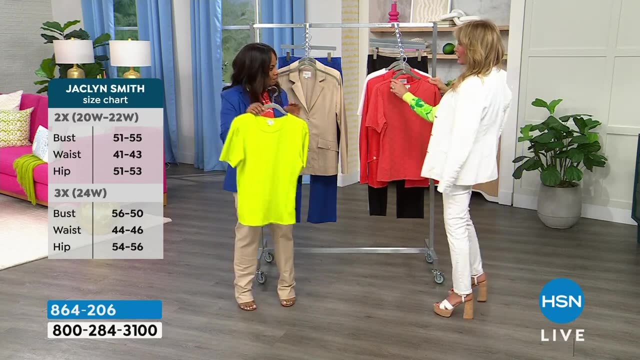 Machine washable. It has rebound. It won't stretch out And the fabric goes around the neckline- the same fabric, So it's not banded in something different. The fabric is carried on the jewel neckline. Yeah, It's such a great piece. 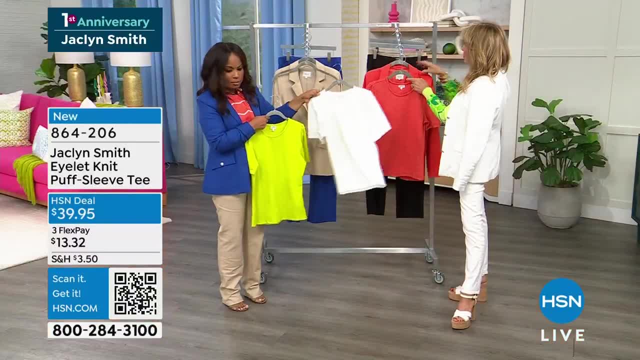 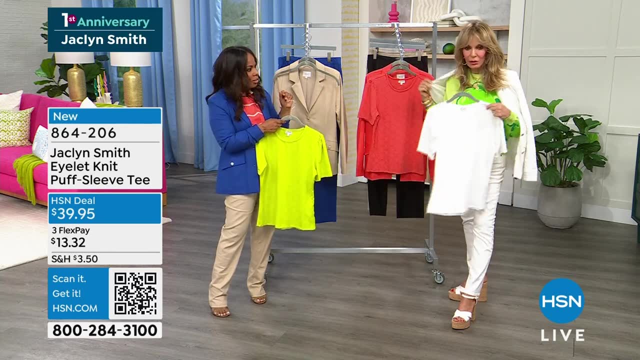 We do have this in an optic white. That's always a wise investment, Mm-hmm, Right, We need a pretty optic white, A classic, Right? Even if you bought a white top- a classic. I even love white on white. 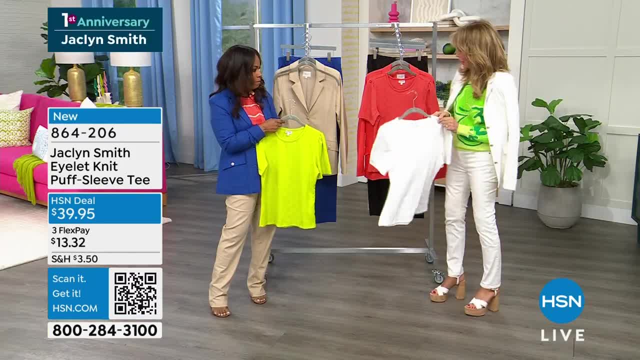 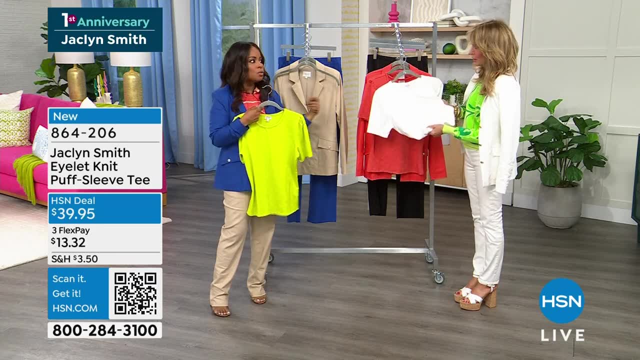 Me too. You know I love white on white. It's beautiful Absolutely. It goes with anything. That's a great, I almost say. I mean I do love color, but if you can swing it, try to get two, because you can't ever go wrong with a classic white. 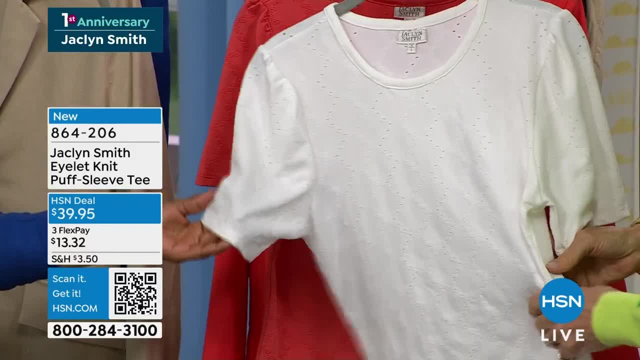 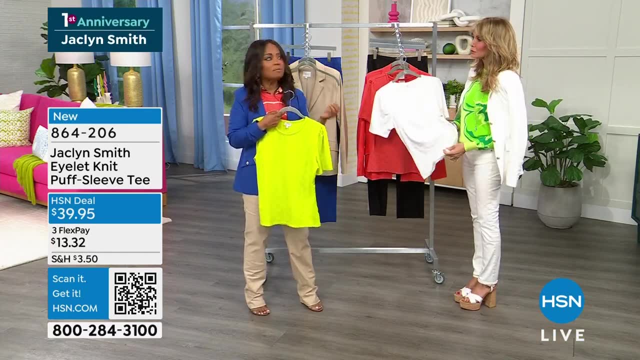 With a white Right And it feels good. Yeah, It wears well And that's gonna take you through with everything And you're looking at $13.32.. Yeah, And what's lovely, if you're new to Shopping With Us, you can use FlexPay on every single. 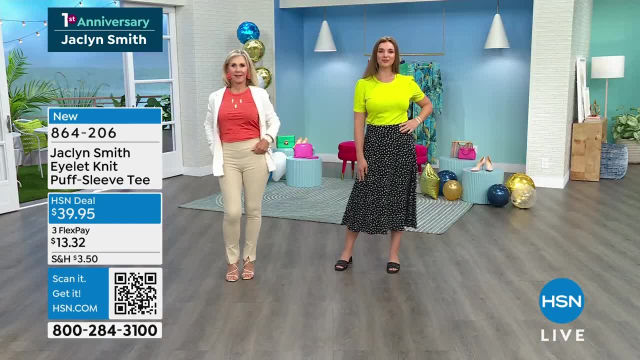 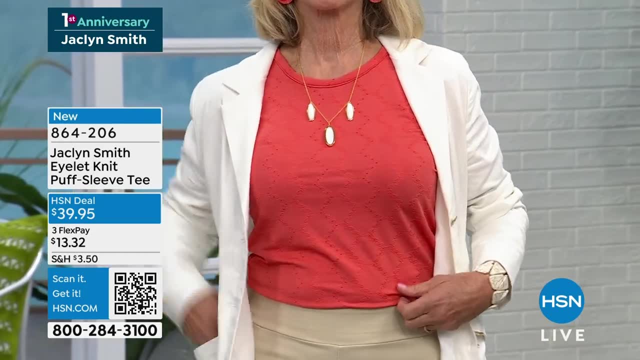 item if it's offered Right. So whenever FlexPay is offered, you can take advantage. There is no you're not limited to the number of times that you can use FlexPay on the day Amazing, Which is really great. It's a gift. 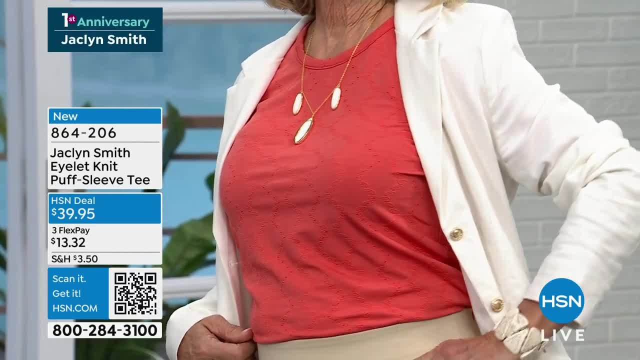 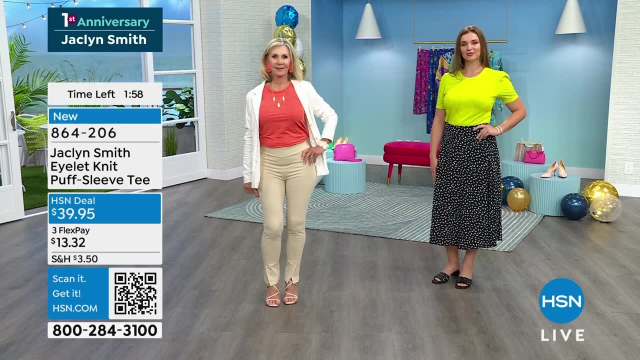 Yeah, What a wonderful offering. It was so cute. I'm gonna tell this story really quickly. So this was a while ago. I went to a bank, There was something going on with my banking and I remember going to the bank and the teller. 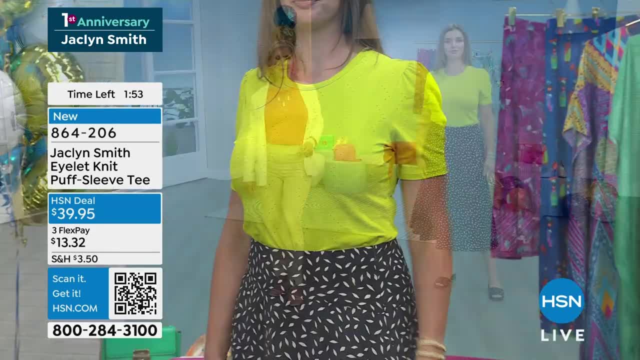 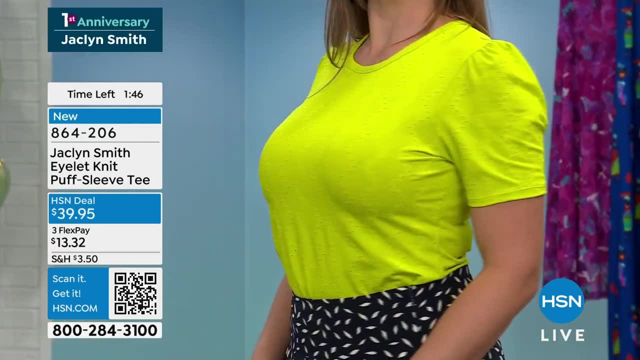 was like. She was like: I see all of these charges on your account from HSN. Oh, I love it And I'm like: well, they're all correct. Yeah, They're all right. No mistake is made. No mistake is made. 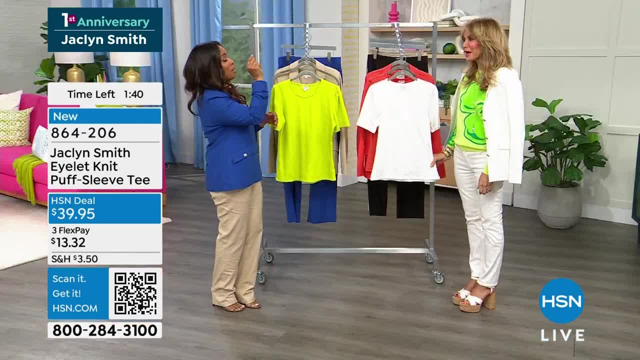 I work there. All of those charges. I love that. It's because I had used FlexPay, FlexPay, FlexPay, FlexPay, FlexPay, Yes, So she saw all of these FlexPay charges Right? She said: is this a mistake? 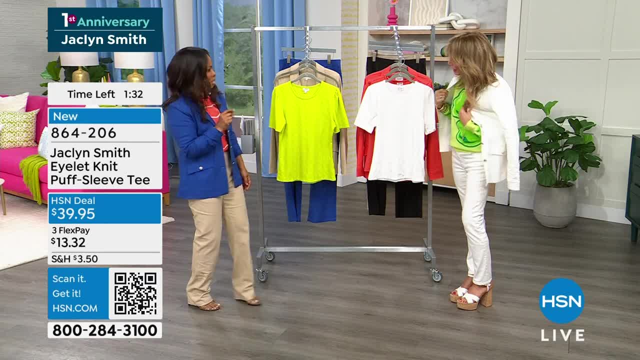 She's thinking: Are you sure? Yeah, So I'm here to tell you that you can. you can go to FlexPay heaven if you want to. Yeah, So I'm here to tell you that you can. you can go to FlexPay heaven if you want to. 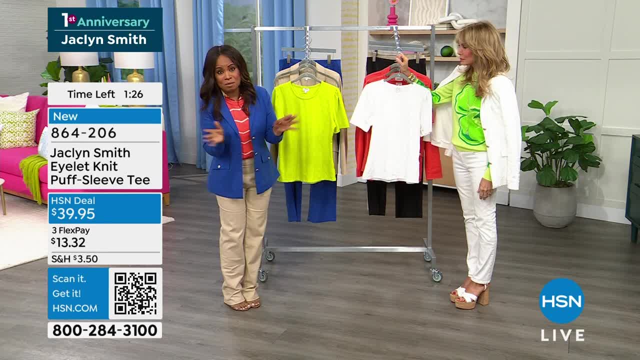 Yeah, So I'm here to tell you that you can. you can go to FlexPay heaven if you want to. That's right On the day. It's really a gift, Yes, To be able to shop that way. Oh for sure. 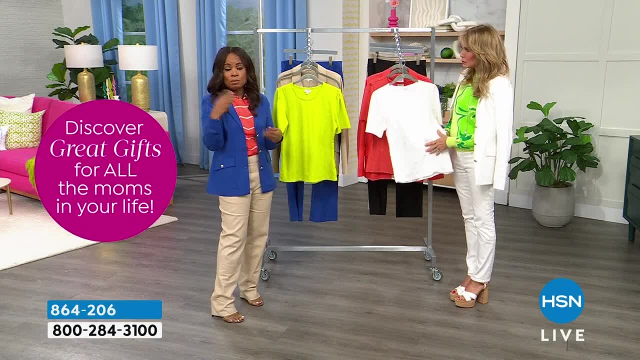 It's interest free, Right, And as long as you're paying it, you know it's off on your end. We don't charge you any interest and you'll get the extra payments every 30 days. So it's a nice way to get those garments that you want. 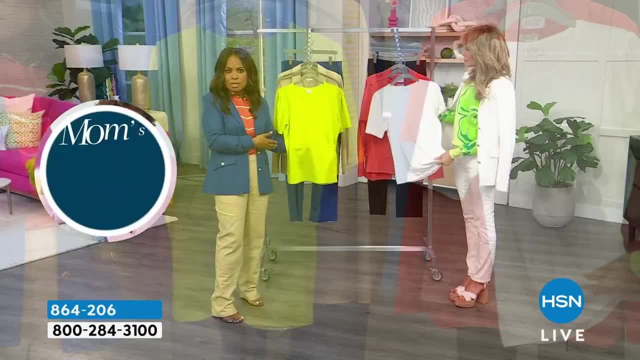 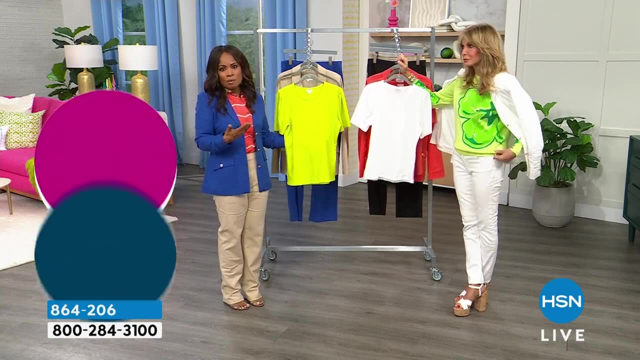 You know that when we're showing you the merchandise, that it's in short supply and it's while while they're available, And then once they're sold out- like the sweater that you're wearing, I know is sold out, Yeah, But these garments we you know you'll have to buy them while they're available. 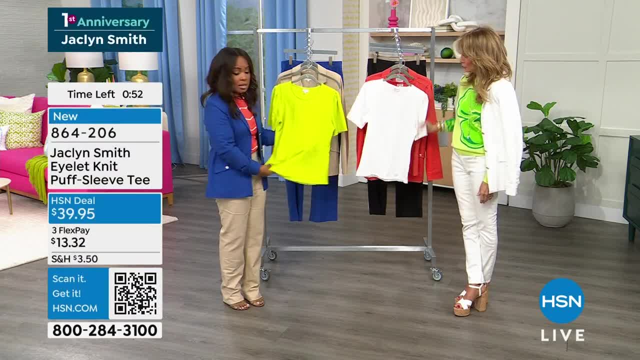 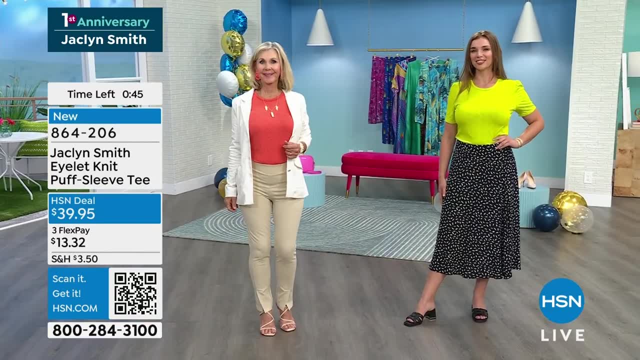 While they're available, Otherwise you'll miss them Right. And this, this particular blouse, is more than halfway sold out. It's $39.95.. I did misplace my card, I can tell you. let's see if I can find it really quickly. 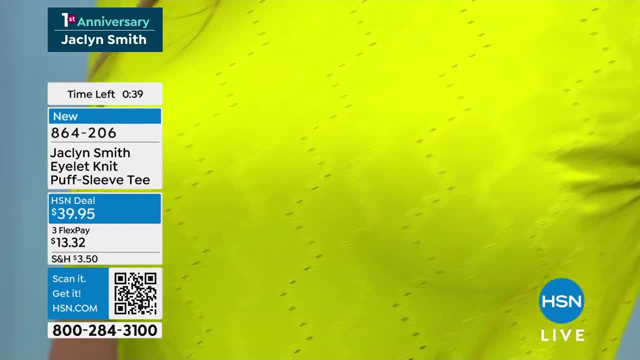 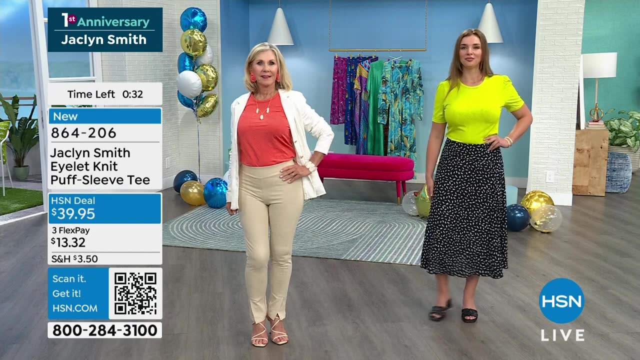 You might have to help me out with this Rocky, with the, with the size on this one Cause we. I know we aired this last hour, but I definitely check online or speak with them. Oh, here we go. I found it. 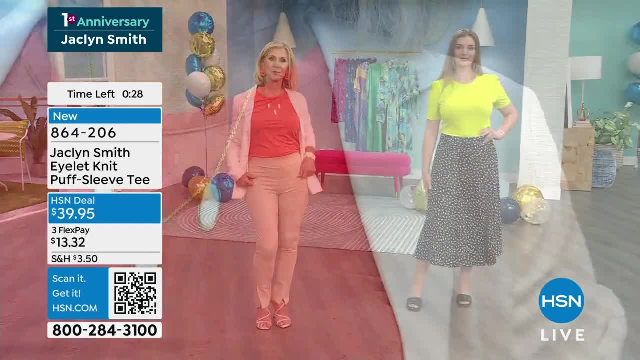 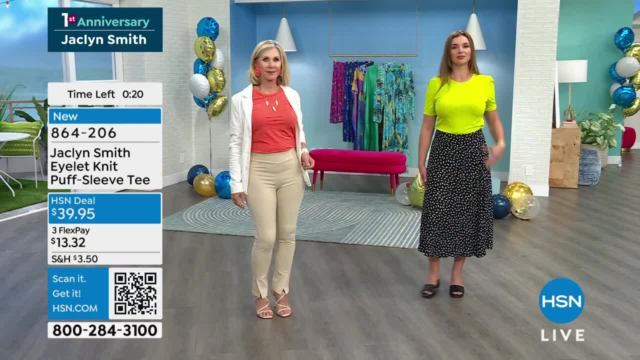 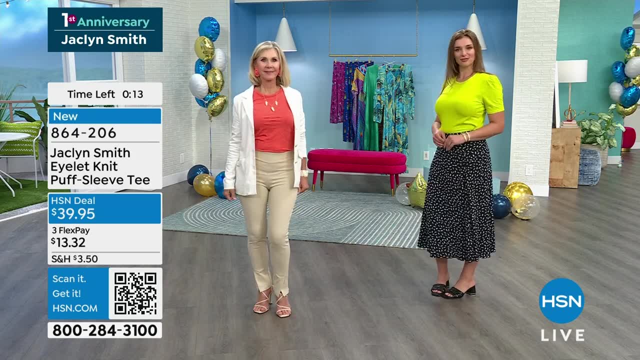 And it's made in Korea. Yeah, And it's made in Korea, But they it's made in Korea, They it's made in Korea. Yeah, Yeah, They are. So that's, that's great, Thank you, Thank you. 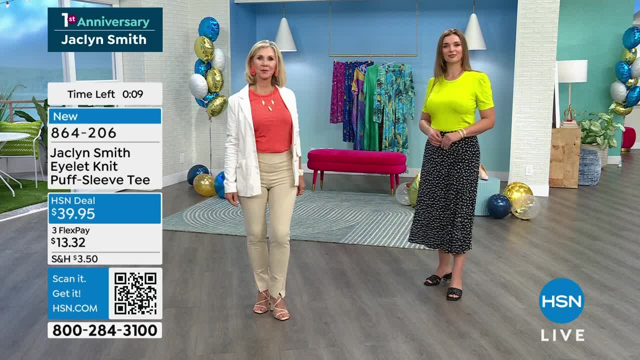 Oh, and then we got one more thing going on. Oh, we have this color on now. I know you've seen it, It's calledITY. I've watched the video. I want to see the video. I want to see, like, what's the color on this one? 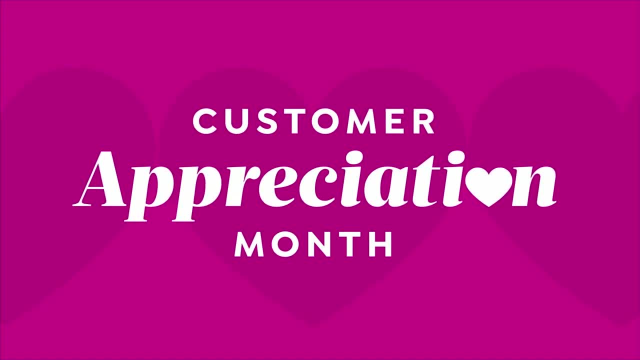 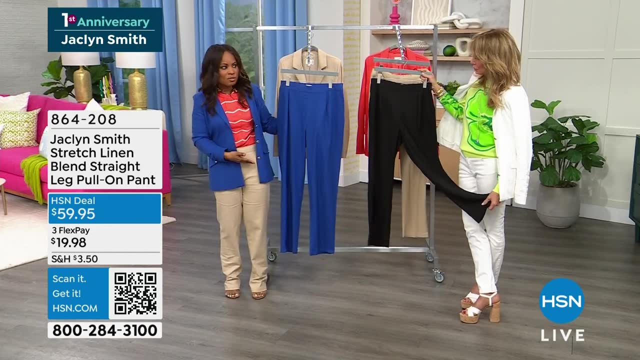 Do you know what that color is? stretch linen pant that goes with the blazer, That goes right back with the blazer, which is really wonderful, So you can see. if you want to do that entire suited look, you can do that. 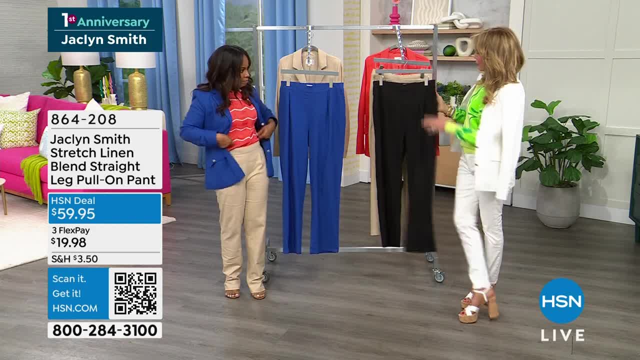 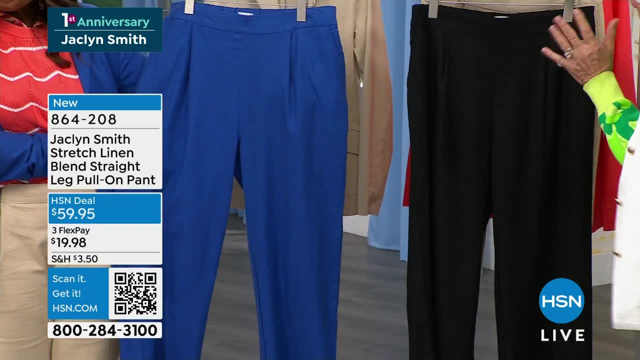 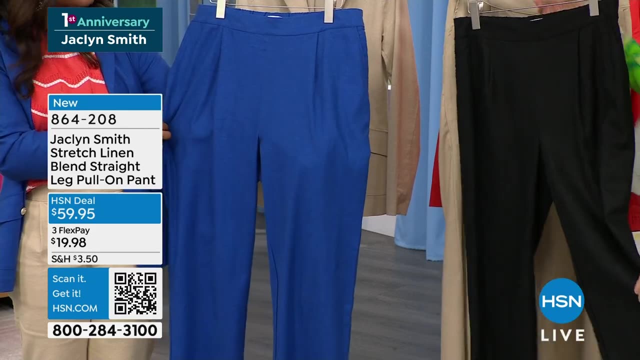 Or these are standalone pieces And it is the same body of my twill, that is the pull-on pant. The same amazing fit. It's a basic, it's the foundation to build your wardrobe on. But I love, you know, when you can put it with the blazer. But again, all these colors stand on their own. 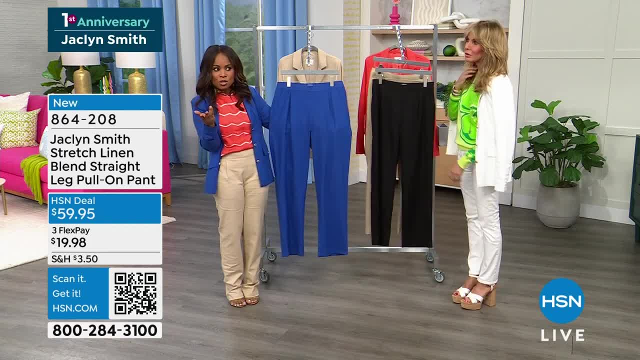 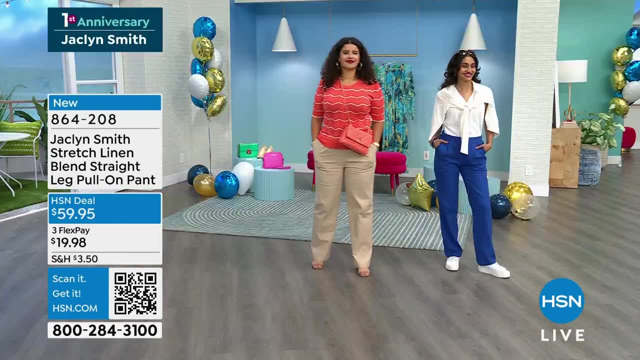 They are fantastic. You know we've had so many pieces in the show. Last hour we started with the little oh, there's the cardigan I was thinking about. You'll see in a moment. You'll see what we were talking about. Look at how wonderful this look. Amazing, So clean, So. 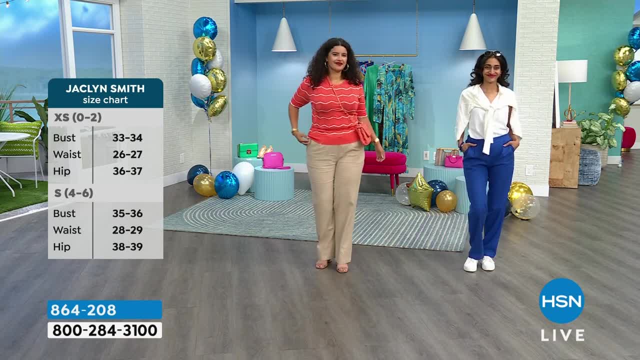 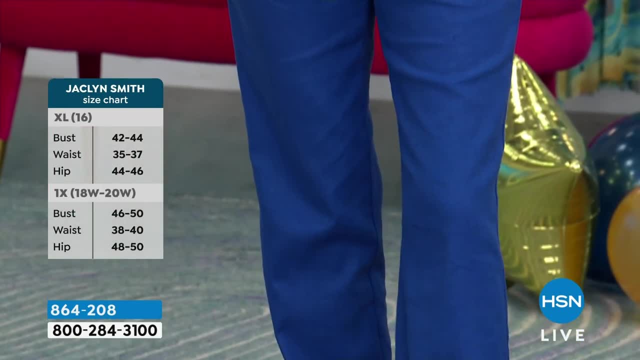 Simi has created this amazing nautical look That's fabulous For the summer. A little cardigan that she has over her shoulders. That's online. We actually gave a full presentation last hour. It comes in that color and it comes in. 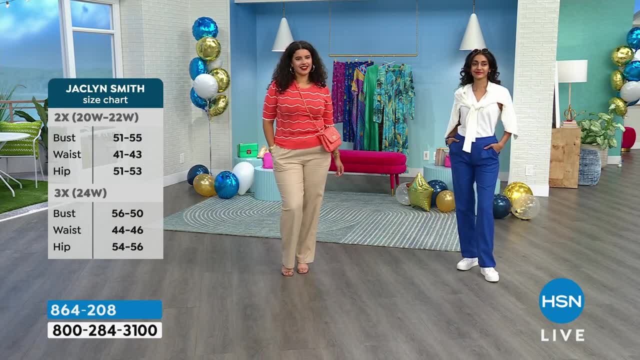 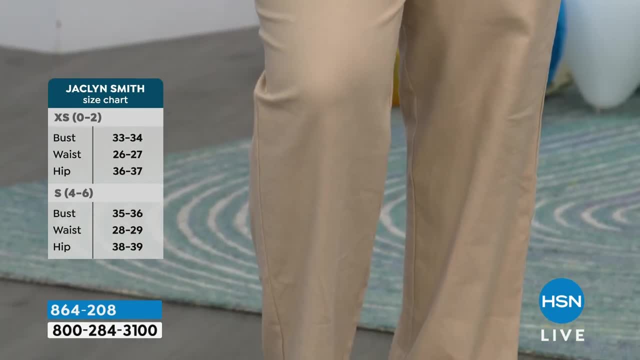 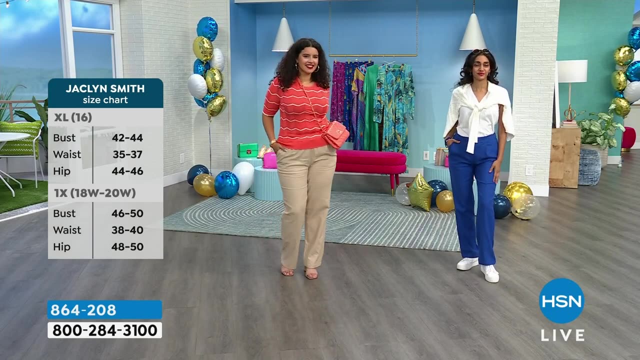 a scarlet red color. It's really beautiful, But you can see how that pant and that blue color and this color blue is so pretty. It's very refined. Yeah, It's not, you know, it's not a navy, It's just perfect. It's like a periwinkle, Yeah, But it's gorgeous And it looks so clean. 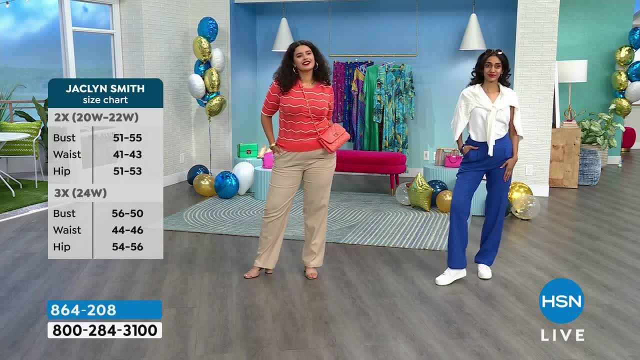 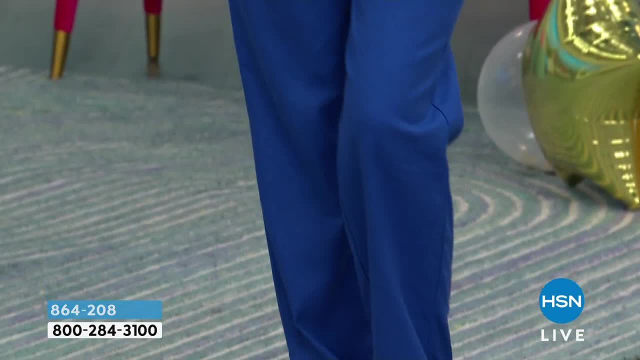 with the white and the white tennis shoes. We haven't seen it with the tennis shoes. I love it. Like I said, you can roll that cuff up, You can wear it with a flip-flop. It's a tennis shoe, But it looks perfect like that. If you'd love to shop, Simi, just so that you know. 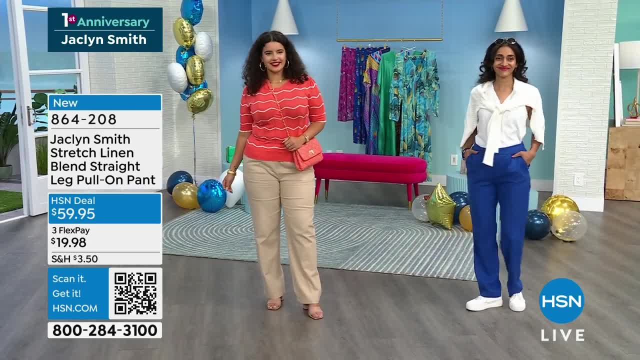 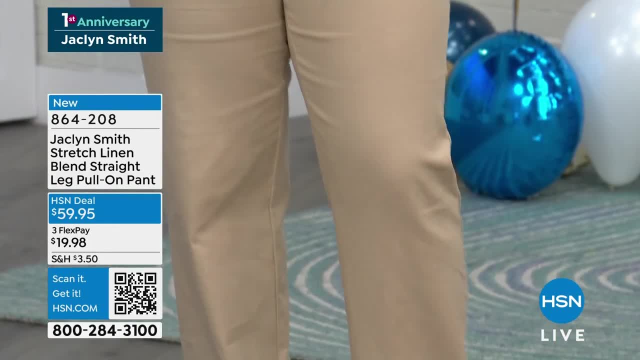 height-wise, she is going to come in at 5'7". In numeric size she's a 4. And she's wearing it in the extra small. And then our Natalie is 5'9". She's wearing the beige color in the pant. In numeric, 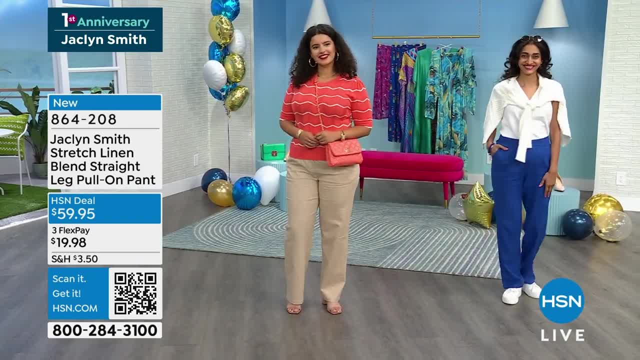 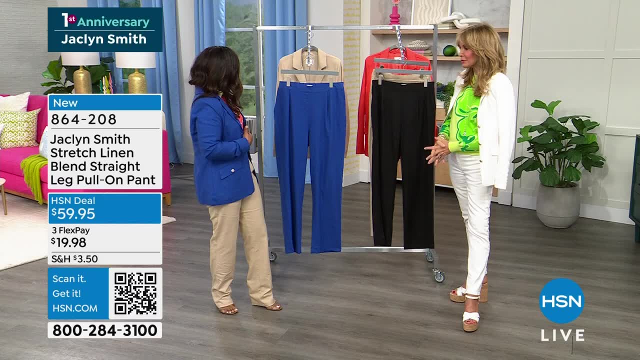 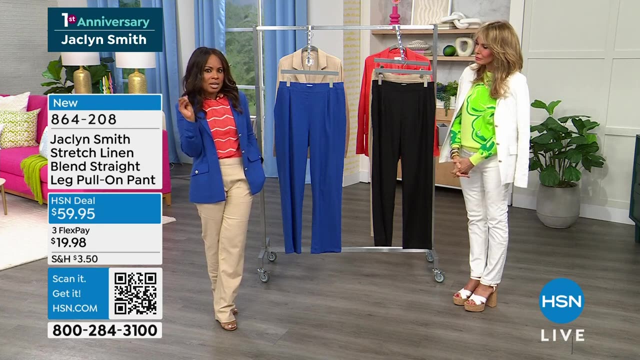 size. she's a 16. And she's wearing the large. Both ladies look spectacular. I love Natalie with the little sweater that I'm wearing, Absolutely The French dressing, So perfect, Right, With the beige. A nod to Bonnie and Clyde: Yes, And even if you're not going, I tend to go tonal because I'm 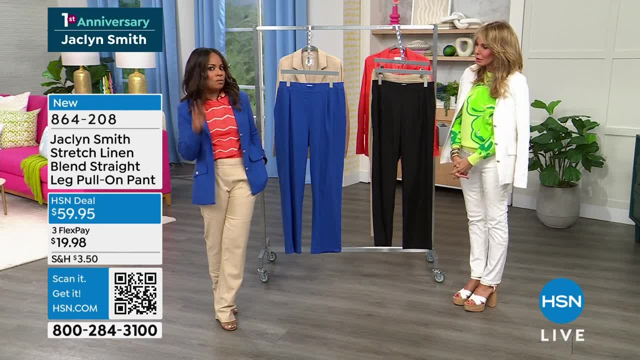 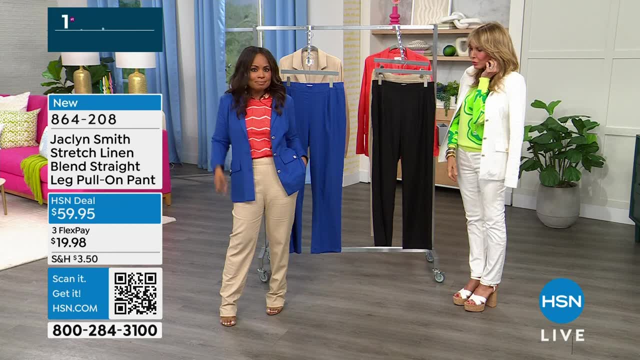 so petite and so short that I like to go tonal because it gives you the illusion of looking taller. But I like kind of the breaking up of this kind of color block. Oh, I do, I do, And it works on you. really. It's fun, you know, doing it that way, You know you just really look very chic when. 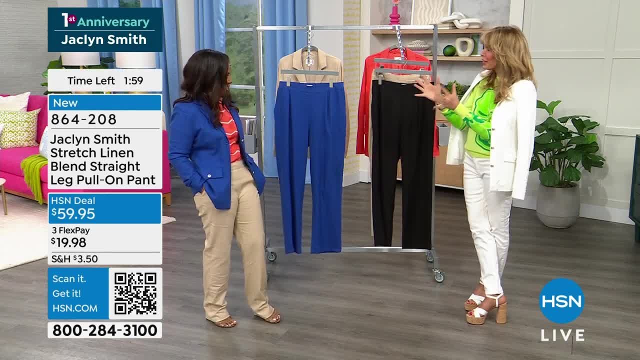 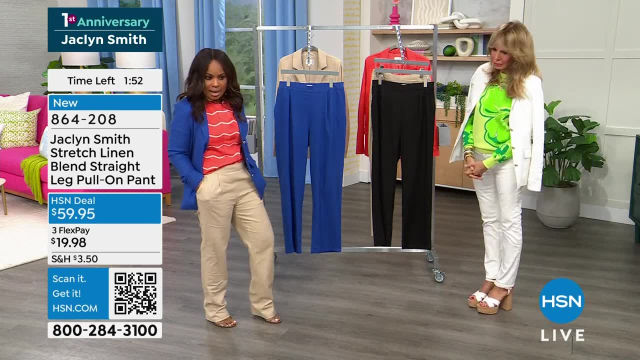 you kind of mix some of the patterns. When all pieces work, it works. It doesn't matter that it's not tonal, It looks beautiful on you. I'm wearing the beige and the extra small, And I do have on a very high heel, I have to admit. 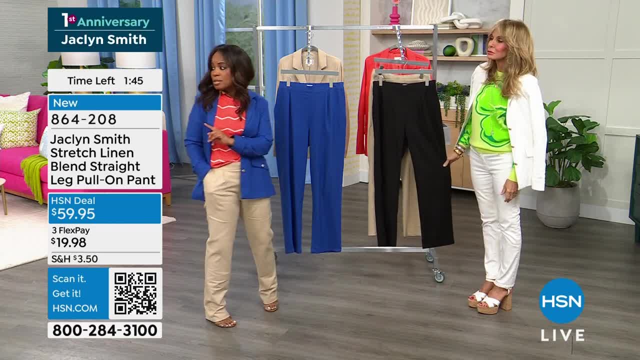 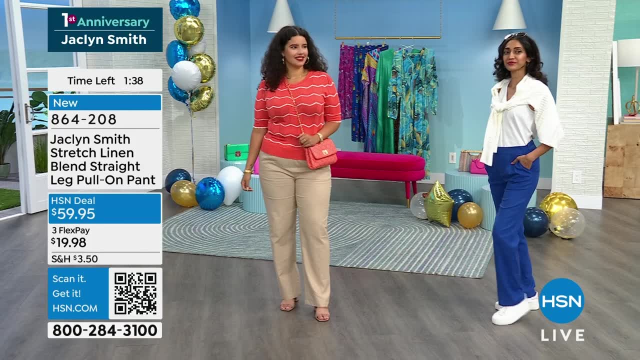 because I am on the shorter side. All right, So you'll notice our models. obviously they're 5'6 and 5,. I believe 5'6 and 5'9". Let me check my cheat sheet here: I think 5'9", 5'9", Yeah, So. 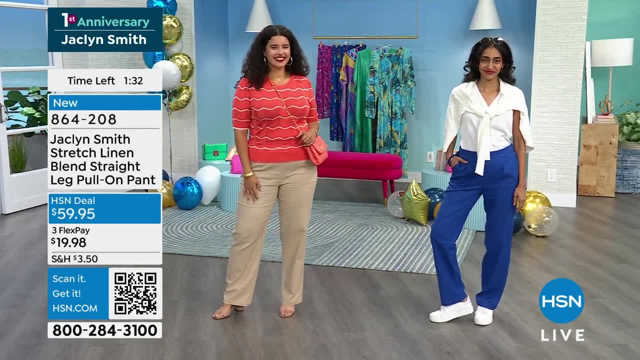 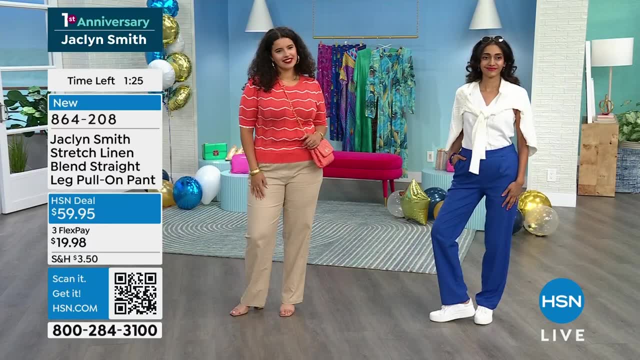 you can see, Rocky, if you can remind me of the inseam on this particular pant, just because I don't know if you can see it. Yeah, I do have two hours of cards And they were great. Oh, you know. 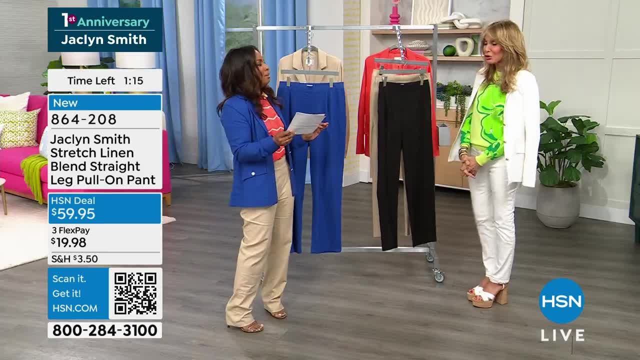 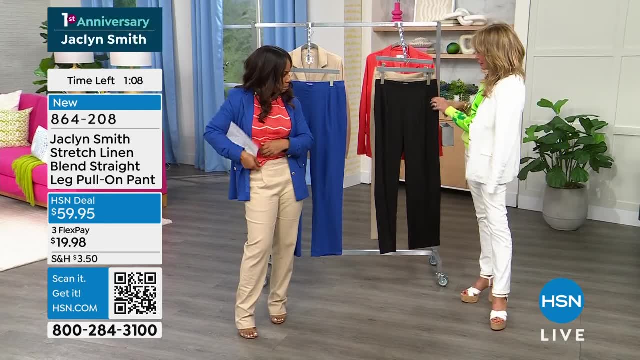 what I found it. I don't know how I did, but I did 30 inches in the inseam. Yeah, 30 inch inseam here. So you've got your nice pockets that are on a slant. Yep To not, you know, add to your hip. 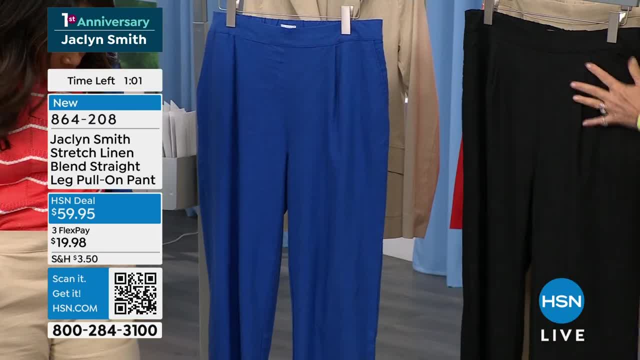 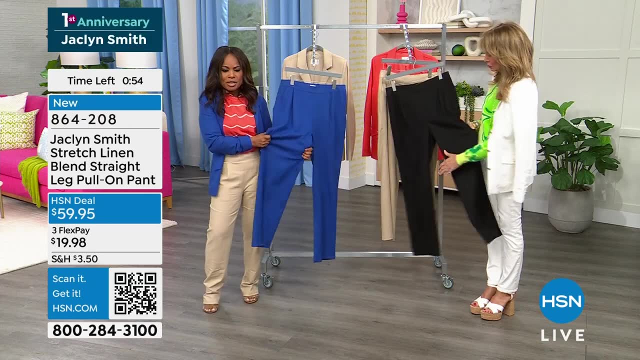 line and gap, It lays flat on your body And it just, you know, slight pleat, And it's a beautiful fabric, because remember it's a beautiful fabric, It's a beautiful fabric, It's a beautiful fabric And remember it's a stretch linen, So you can't think traditional linen, a traditional linen. 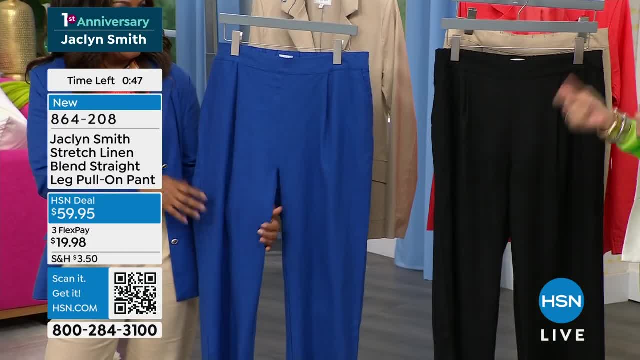 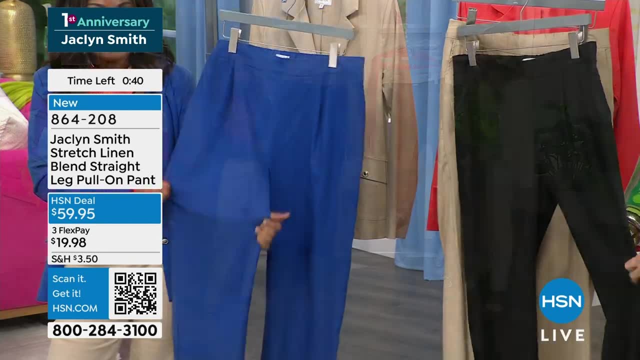 wrinkles like nobody's business. Yeah, That's another whole story. And it's also a little itchy and not as comfortable on your body. It's a little bit more stiff, Yes, Where this has a little bit more bounce to it And it has a sheen, don't you think? Yeah, I think it's really pretty, It's not? 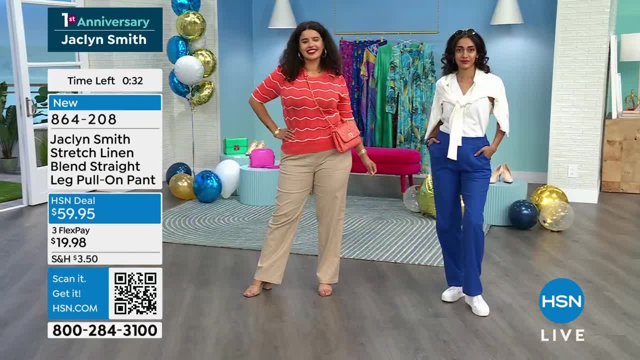 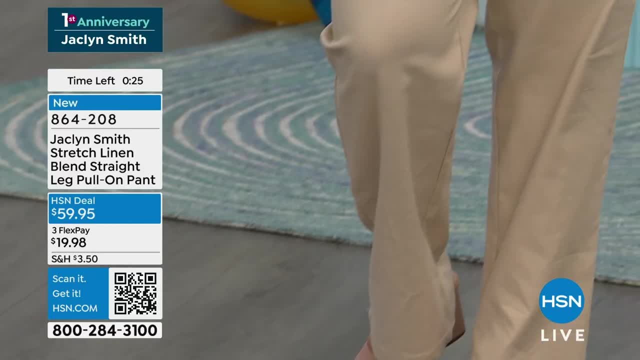 flat? Yeah, Absolutely. So I'm going to just show you a little bit of that stretch and you can see it there. There, it is in the beige, and we have it in the blue, but we also have this for you in the beige as well. So those are going to be your choices. I do want to let you know that we are.